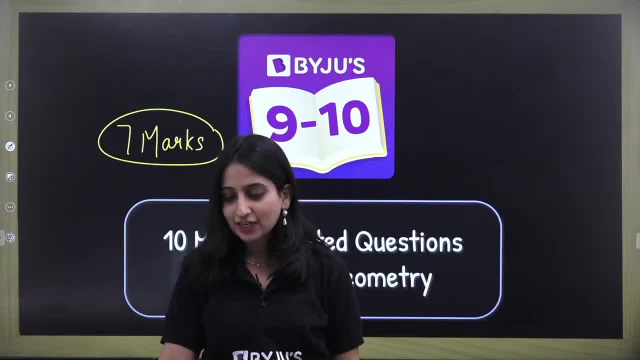 everybody. Good evening. Nitya Chitra Prachi Aradhya. So make sure, if you are coming here live and watching this session or you are watching the recorded session, watch till the end, watch at 2x speed, because it is very important. 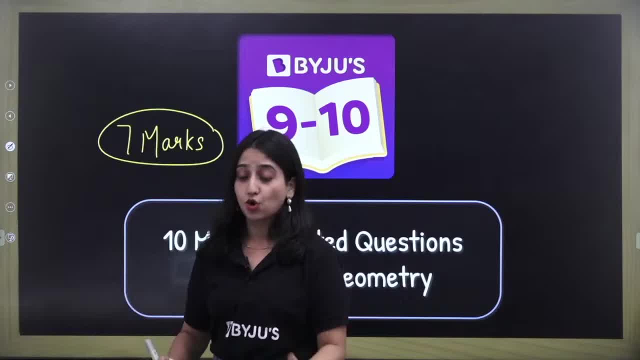 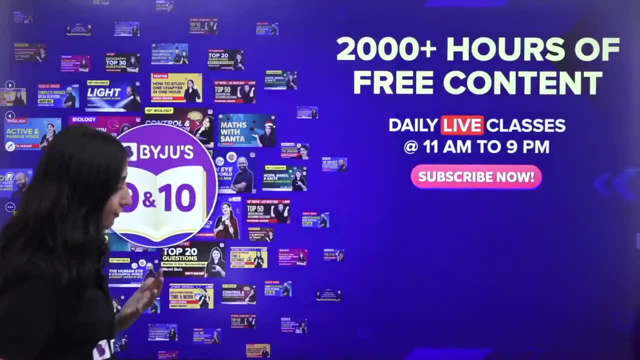 to question: Watch live, watch recorded, watch recorded, watch recorded: that is your wish, okay. So let's start today's class, But before that, let me tell you what we have, what we are doing on this channel. So we have created like 2000 plus hours of free. 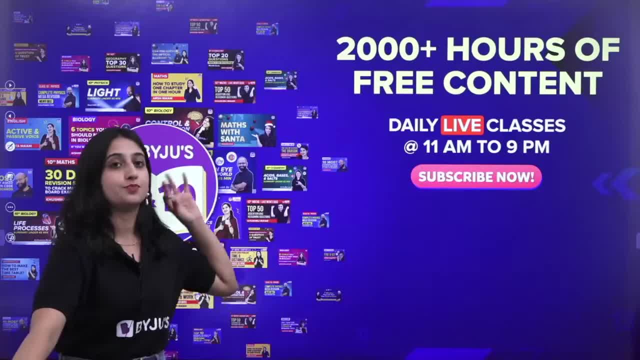 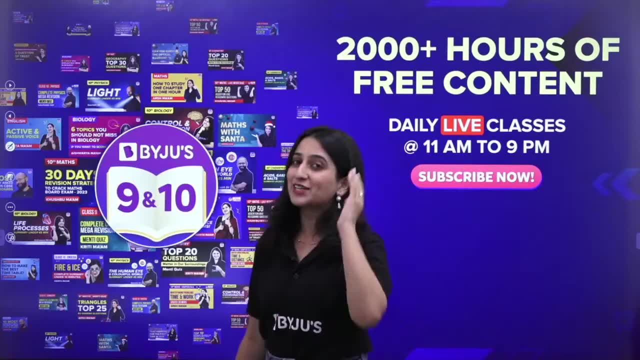 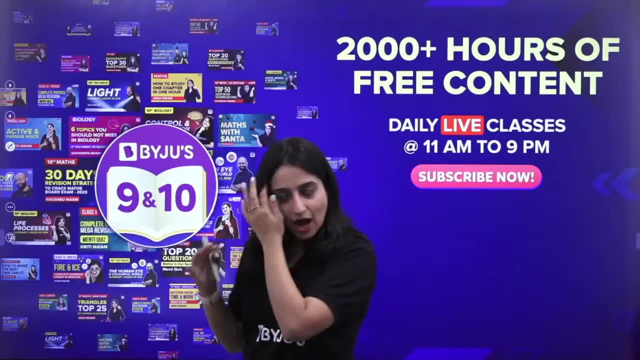 content for you guys and brilliant Sessions, brilliant videos goes here on this channel Every single day. we come here live so that you guys can ease your board exams, school exams like this. okay, So we are connected with you from the beginning and till the end. till you don't sit in the exam, don't prepare, 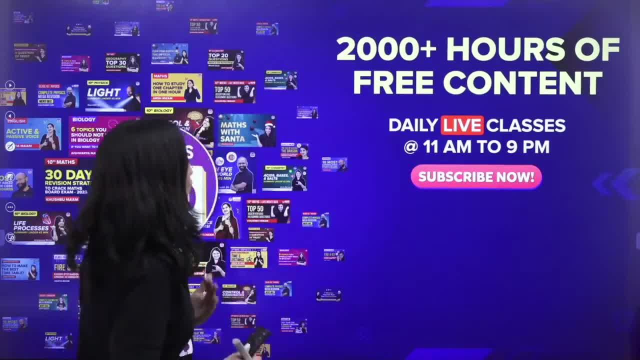 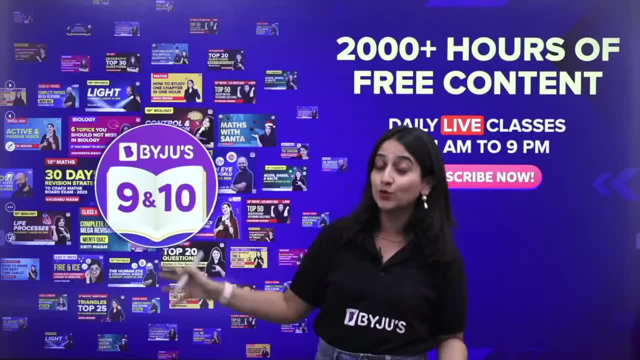 for the exams. we are going to be here for you. So if you haven't subscribed the channel yet, or if you haven't explored the channel yet, or you are new today to this class, so make sure you subscribe, because if you are not, 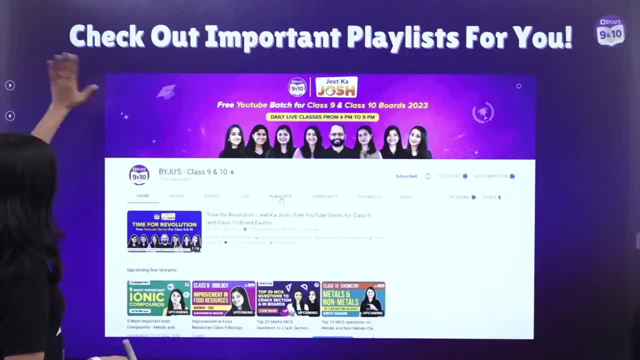 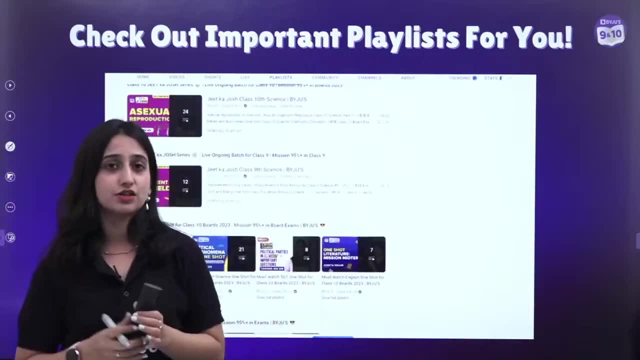 subscribing. that means you are missing out on something, right? Also, we have created these important playlists for you so that you don't have to search here and there on the channel. that ma'am, we want to see this session. where to see? can't find it, whatever. 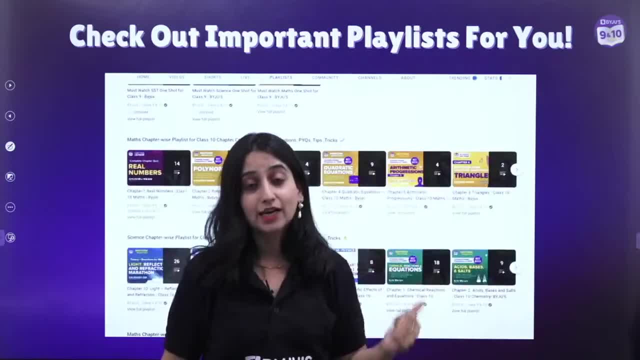 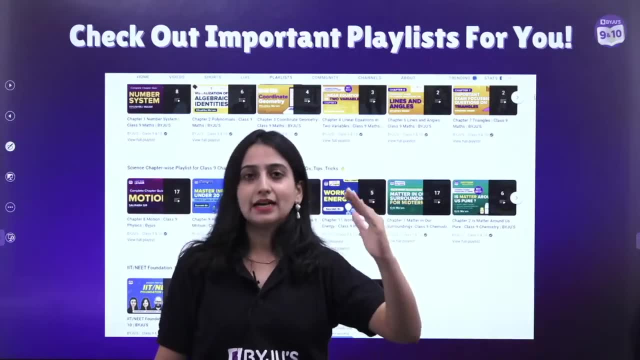 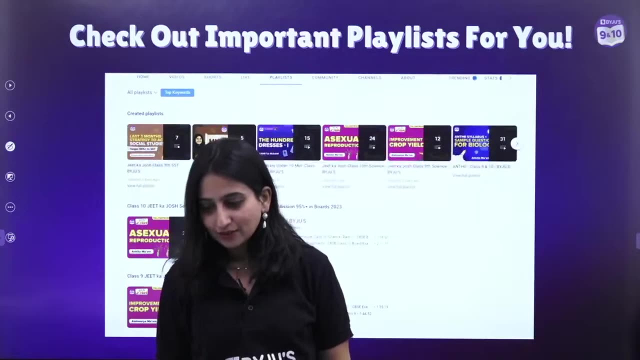 So we have created an important playlist for you guys: grade wise, chapter wise, subject wise. you will get all the playlists, okay, And whatever you want to read, all the content will be available. Yes, good evening, Ritu hi Niksha, welcome to the class, hello pro. 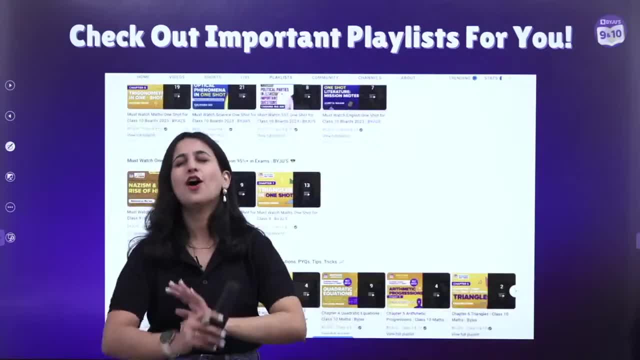 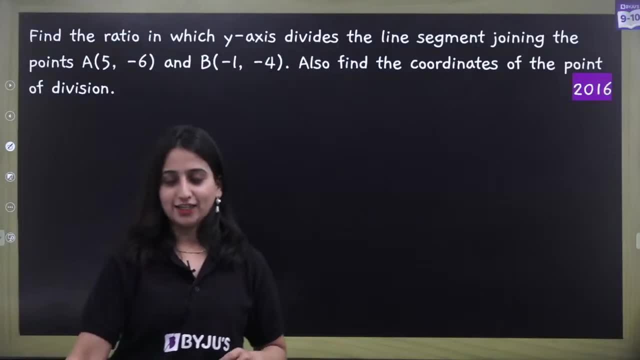 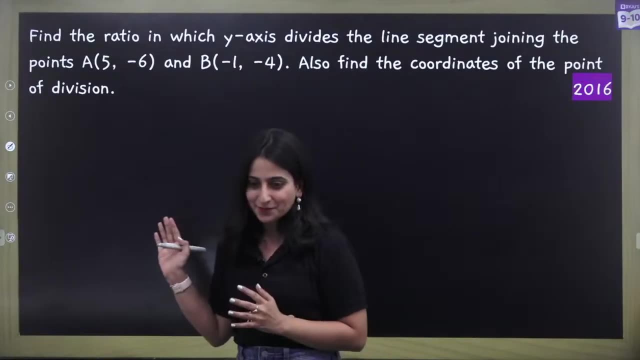 gamer. I am doing great. thank you for asking. I hope you all are doing absolutely amazing. yes, bacho. yes or no. how's the josh? yes, So are we ready to crack this chapter? Are we ready to like secure our 7 marks from this chapter? Yes, so start karte hain with the. 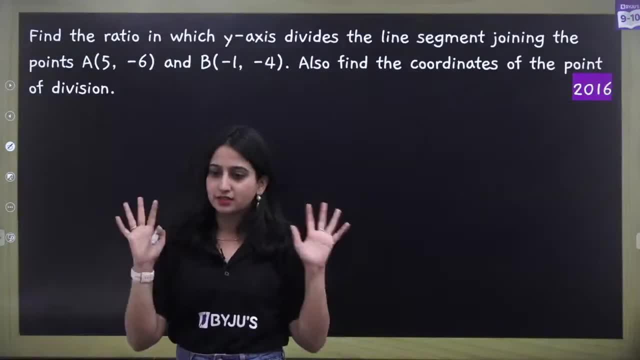 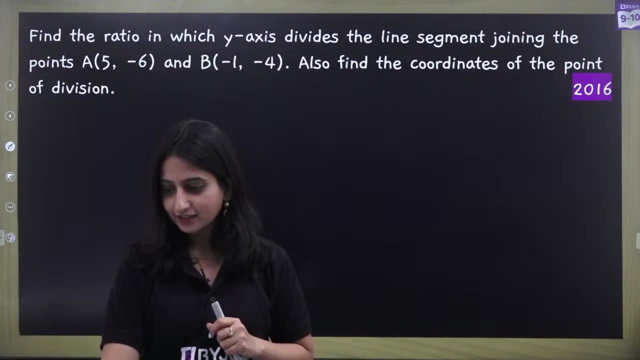 very first question on your screen. So are we facing some lag? Yeah, alright, Am I audible, bacho, Am I audible and visible? Yes, start kijiye, bas start. kardiya aapko question dikha diya hai. Chalo jisko question. 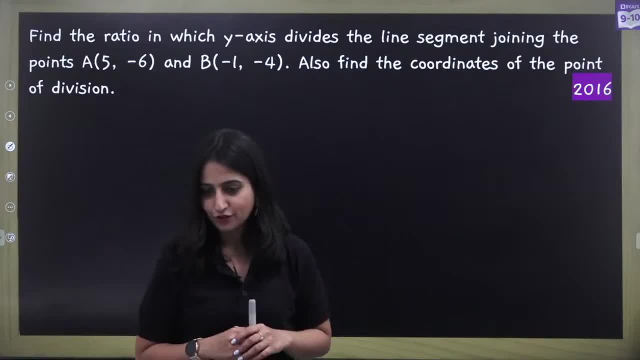 aata hai wo question karna, start kardo and let me solve it with you. I think we are completely audible, visible. now, Okay, agar beech mein kuch bhi dikkat aati hai to do, let me know. 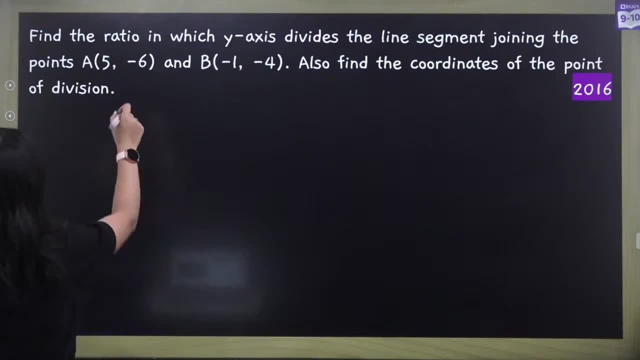 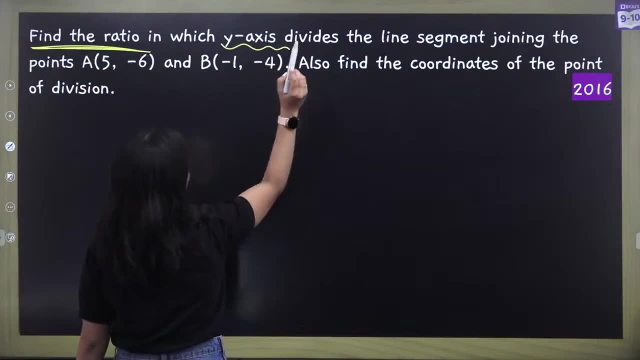 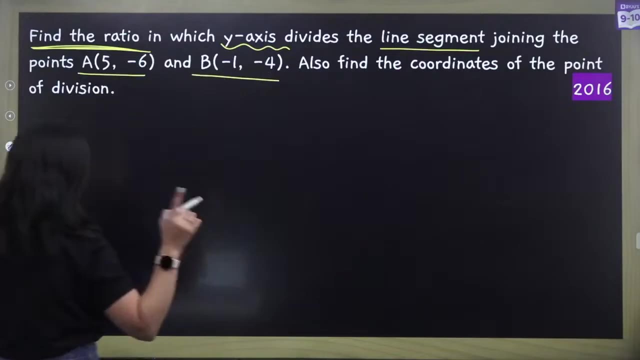 chat mein aap saath ki saath batate reyna Chalo find the ratio. So basically, is question mein kya nikalna hai? we have to find the ratio in which y axis divides the line segment. Line segment- kaunsi hai Line segment joining the points A and B? To sabse pehli aise questions. 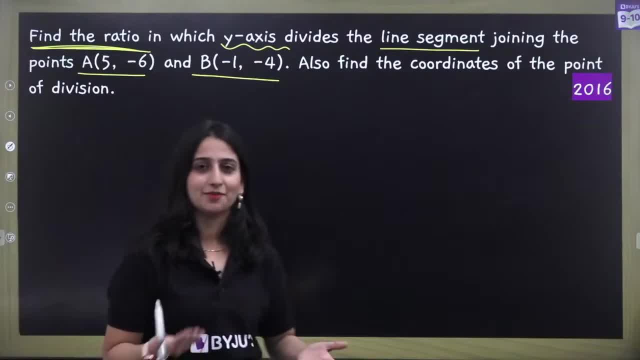 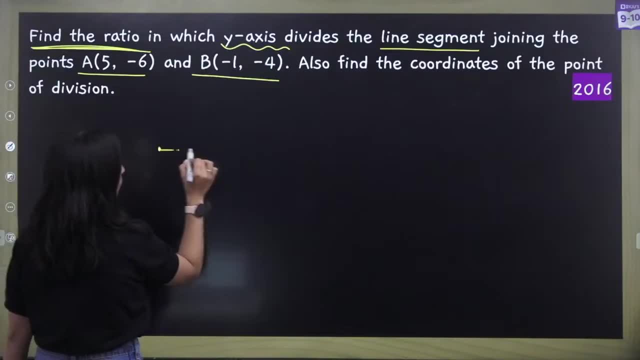 mein hum diagram banayenge, obviously, because bina diagram ke coordinate geometry ka question kaise karoge na awa mein nahi kar sakte hai. So let's draw the line segment A, B, Chalo ek line segment A bhi bana diya right, And coordinates of A is given to us. that is. 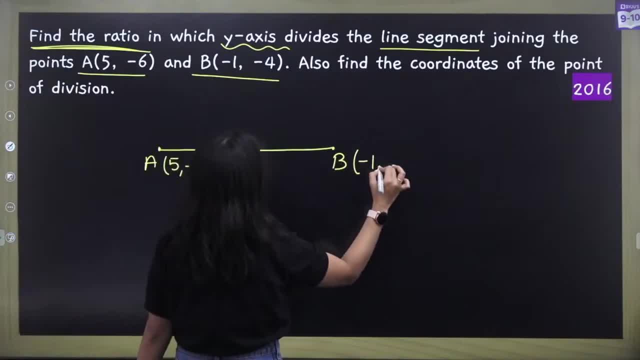 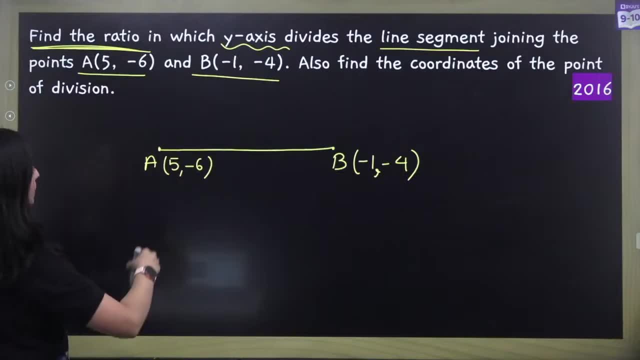 5 comma minus 6.. Coordinates of B are 1 minus 1 comma minus 4, yes, great. What else is given to us? We have to find the ratio in which y axis divides the line Matlab. there is some y axis maan lo ki ye hamara. y axis hai Maan lete ki. this is our y axis. So 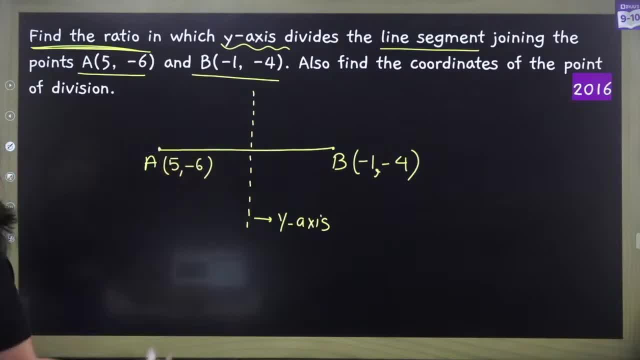 y axis is dividing this line segment in some ratio. I don't know ki, wo ratio, kya hai. So let's assume that it is intersecting this line segment at point- let me call it m right- And it is dividing this line segment in the ratio k is to 1.. Now there is one. 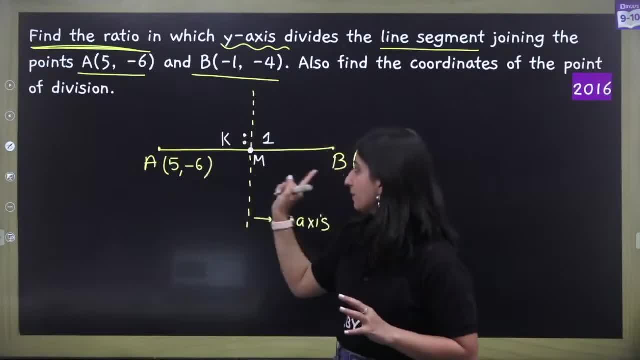 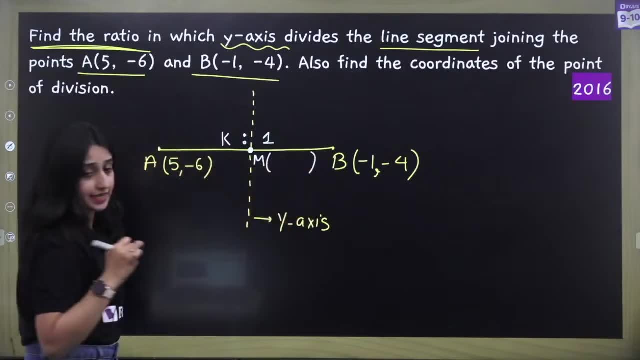 thing that you need to understand in this question: ki yahan pe m ke coordinates kya hongi. Can anyone tell me what should be the coordinates of m Bacha? m ke coordinates kya likhu yahan pe? Because it is saying that the ratio in which y axis- this is basically 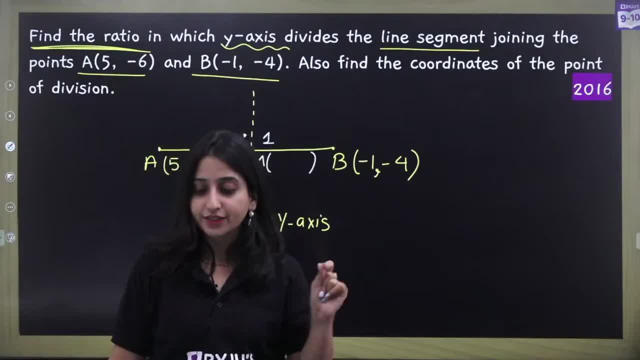 y axis ke upar. agar koi bhi point lete hain usme, kya uske coordinates kaise le jata hai? Very good, Suresh, Suresh, Shreyan Shabash, Ashraf, no, Ashraf, no, Okay, yes, very good. 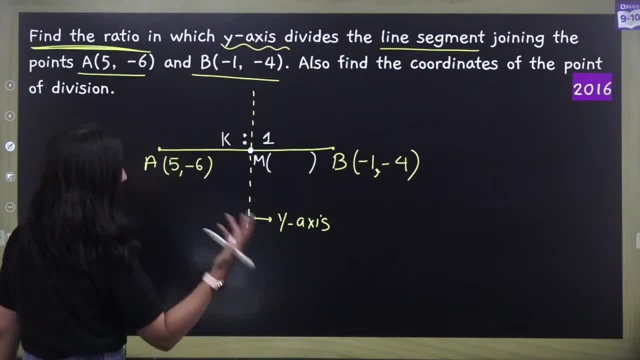 Abhinav, So coordinates, agar y axis ke upar le re hain, toh hume pata hai, ki y axis ke upar x coordinate hamesha 0 hota hai. y ki value kuch bhi ho sakti hai. So I am taking. 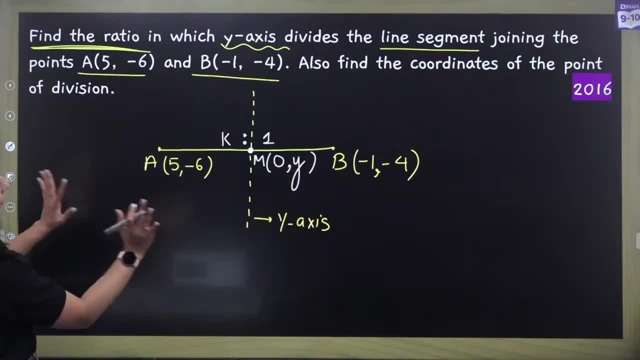 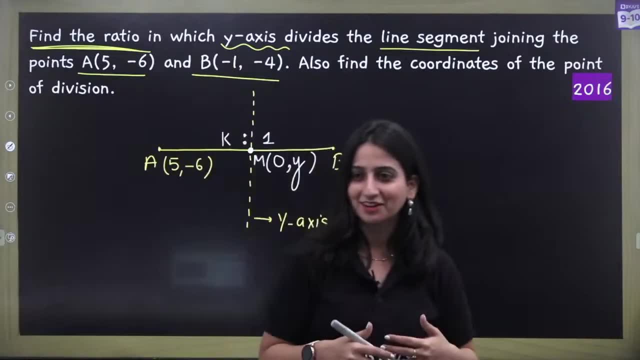 it as y. So I hope the diagram ab tak ekdum se clear hai. Is it clear to you all? Am I voice? is my voice echoing, Like I can hear the echoes? Is it fine? Okay, So haan. 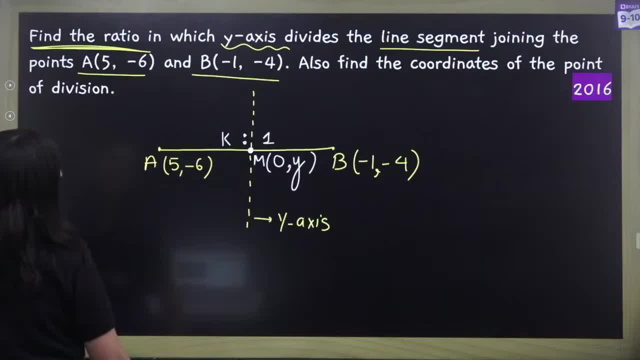 bahut easy hai, bahut commonly asked question hai: Chalo ab kya karenge. batao mujhe Ab apke paas ye point de rakha hai, ratio k is to 1 hai, wo hume nikalna hai. and these points: 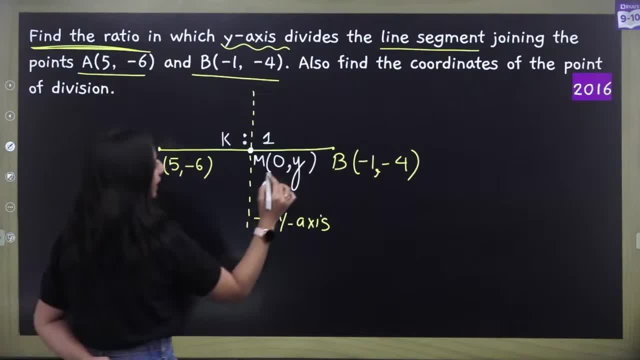 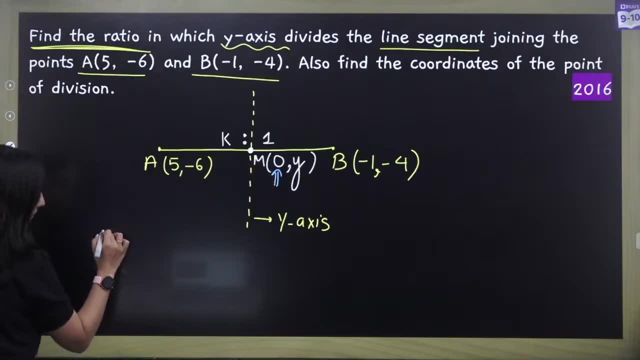 are given, Toh jo hume given hota hai. uske basis pe hum section formula lagayenge, Toh yahan pe kaunsa formula lagayege: Section formula. Toh section formula lagate hain. bita section formula. kya kaita hai Ki jo x, hai hamara jo x is equal to x is equal to x. 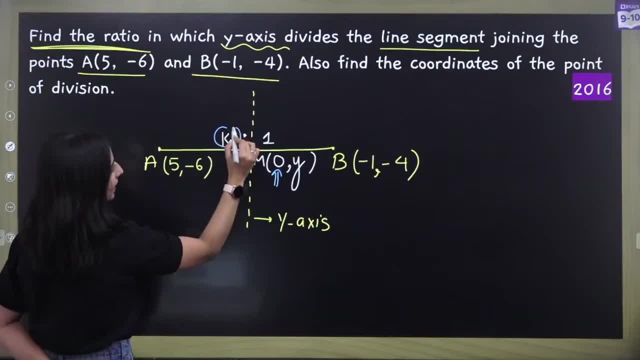 woh kiske barabar hoga. That will be equal to this k multiplied by this minus 1, right Plus this 1 multiplied by this 5.. So 1 ko hum 5 se multiply karenge Divide by ratio. 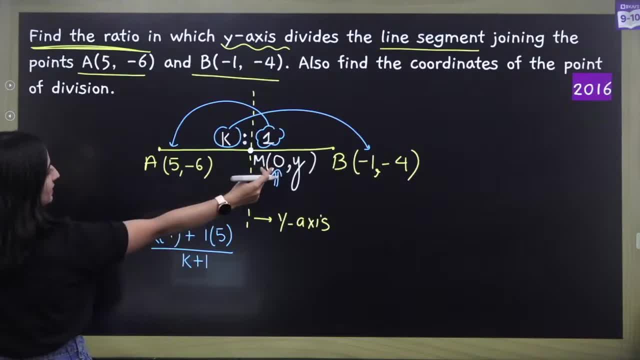 ka sum. Now we know that this point x coordinate, this is already 0, toh I can put 0 here, Right? So it will become minus k plus 5 upon k plus 1.. Toh, k plus 1, u d必a up believing. 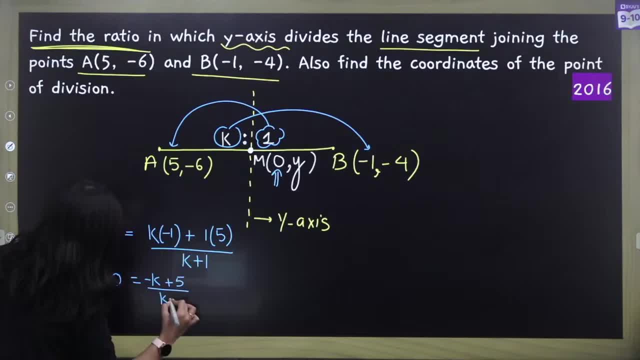 that x is already 0,. toh, I can put 0 here, Right, So it will become minus k plus 5 upon k plus 1.. Toh, k plus 1, up believing that x is already 0, up believing that x is already. 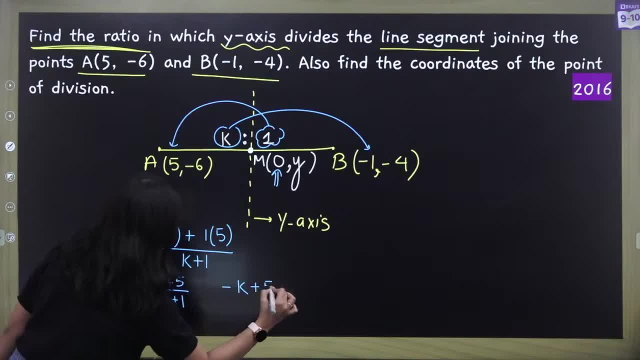 0, so it will become minus k plus 5 upon k plus 1.. Then where is the minus? So up believing that multiplied by 0. So I will get minus k plus 5 equals to 0. That means k equals to 5.. So 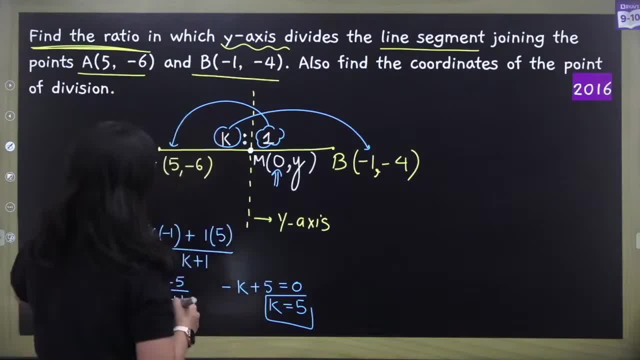 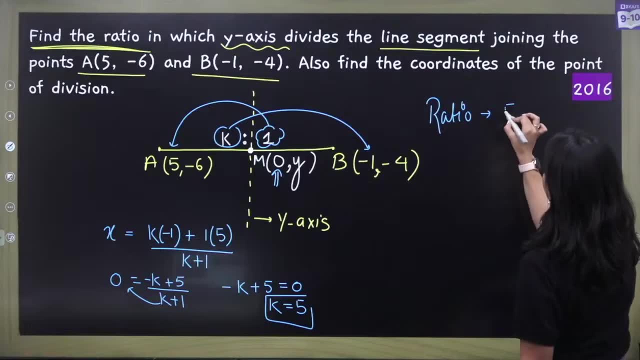 if k is 5, everyone's k is 5.. Very good. So if k is 5, then what is our ratio? So the required ratio is. so what is the ratio? Our k is to 1.. Ratio is 5 is to 1.. Do you want to take out anything? 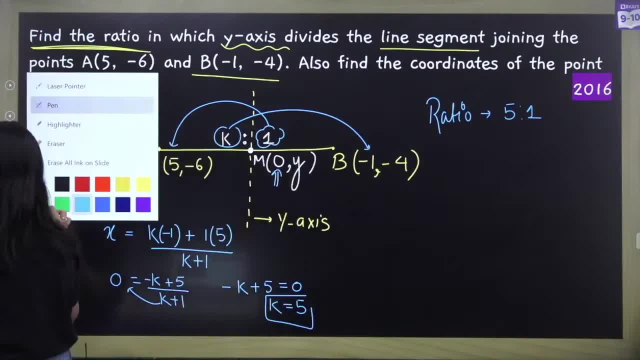 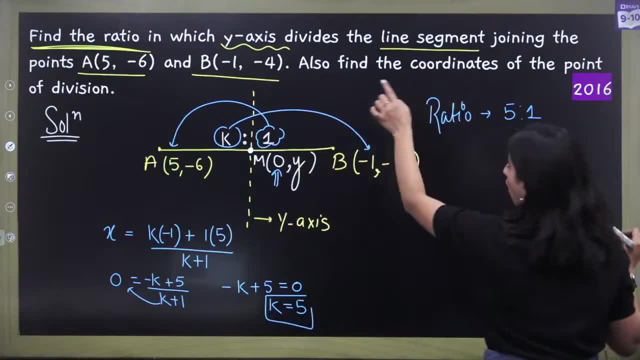 else in this question. See, some children will solve the question here and say, ma'am, our answer has come and the marks will be cut because the last line is not read again. Also, find the coordinates of the point of division. We also have to find the coordinates of the point of division. 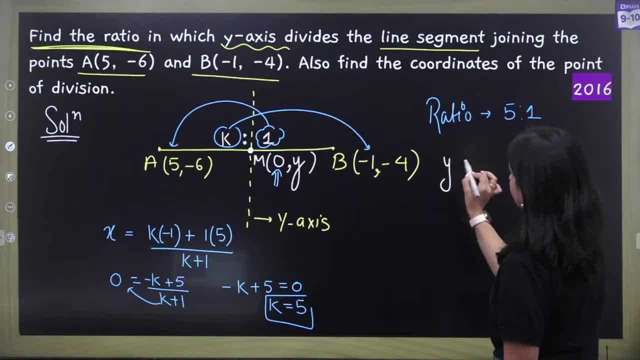 That means we have to find this y as well. How will this y be found? Let's apply the section formula again: k into y, coordinate of this b, So k into minus 4 plus 1, into minus 6 divided by k plus 1.. Now 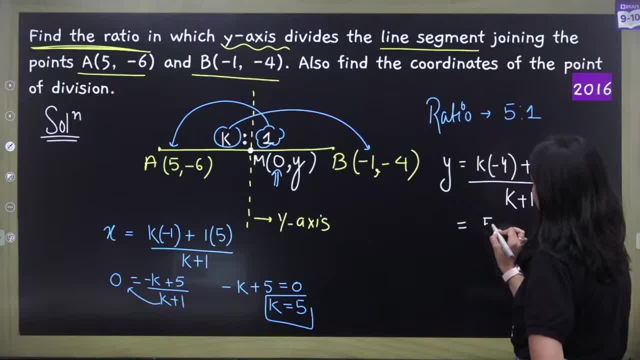 we have the value of k with us, That is 5.. So here, 5 into minus 4, plus 1 into minus 6 divided by 6.. So what has become? It has become minus 20 minus 6 divided by 6.. So minus 26 divided by 6.. So what is the value of k? 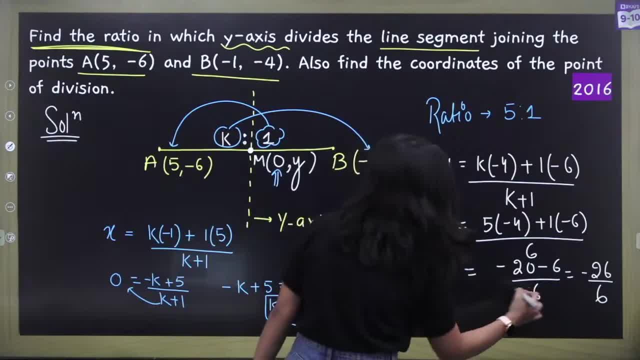 Sorry. what is the value of this point? Very good, Cut it from 2.. So y coordinate will come to us. 2- 3's are 6,, 2- 13's are So minus 13 by 3.. So your final answer will be: 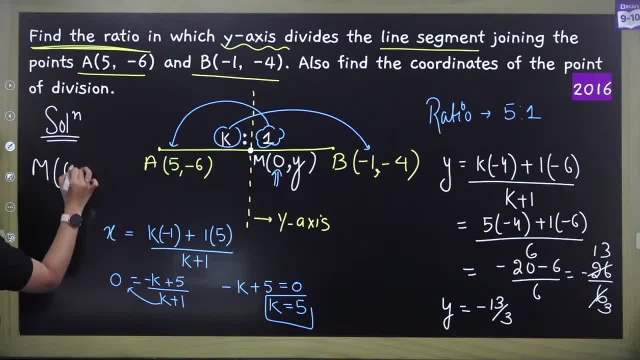 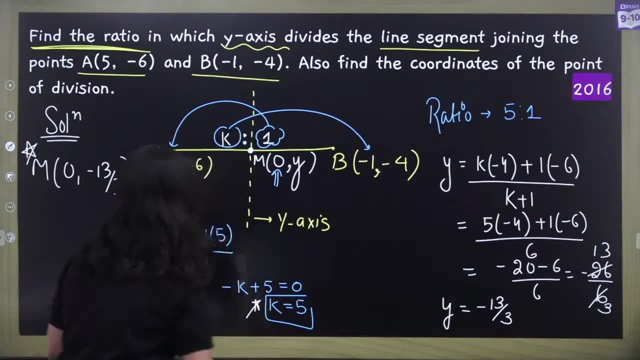 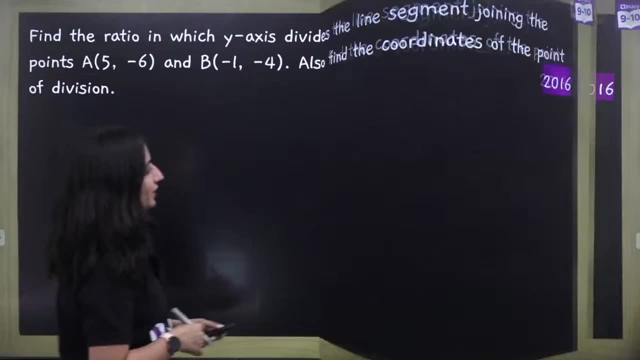 coordinates of MR, 0 comma minus 13 upon 3.. When you give these two answers then you will get full marks in this question. Is the question clear to you Everyone? question is clear. Come on, now let's move to the next question. 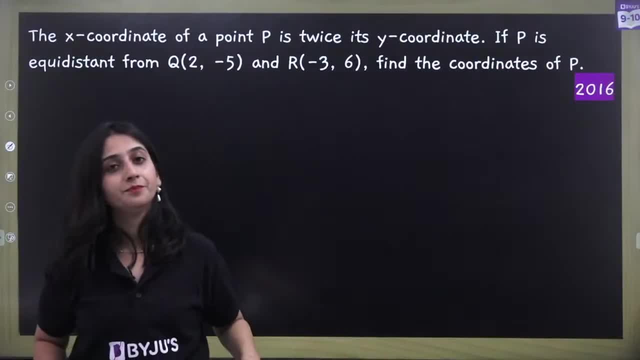 Come on, let's see the next question: How many of you have already practiced? Okay, and you are able to give me answers. Those who have not practiced, they will practice with me today. Okay, come on in 2016,, I asked. 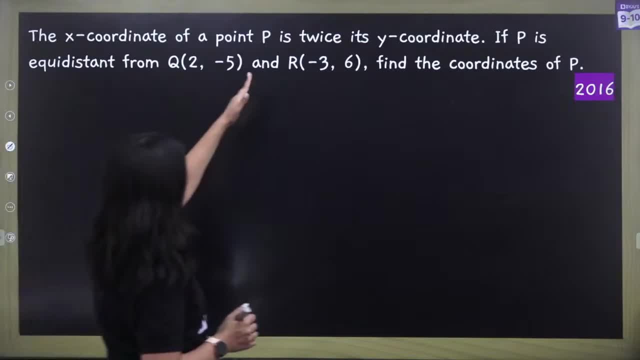 the x coordinate of a point P is twice its y coordinate. If I read only the first statement, kids, what do you understand If I only read the first line? what are you understanding from this line? Yes, already practiced Radhya, That's great kid. So what do you understand here? 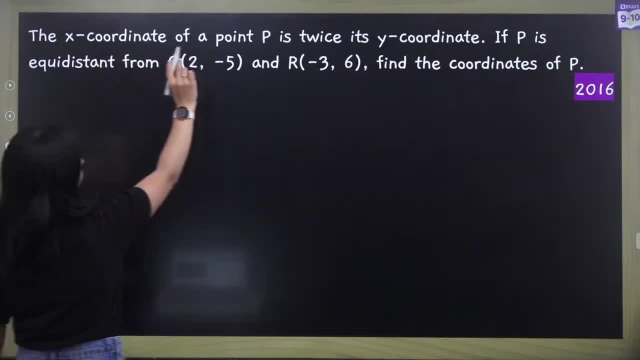 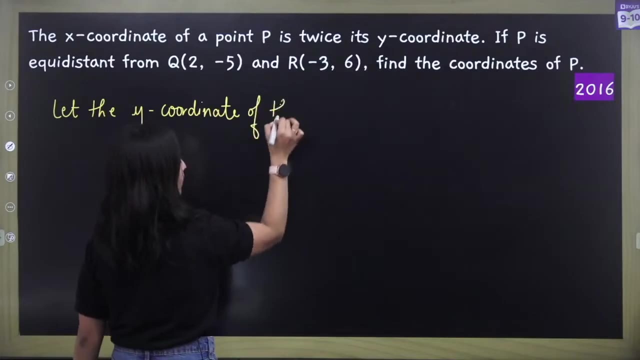 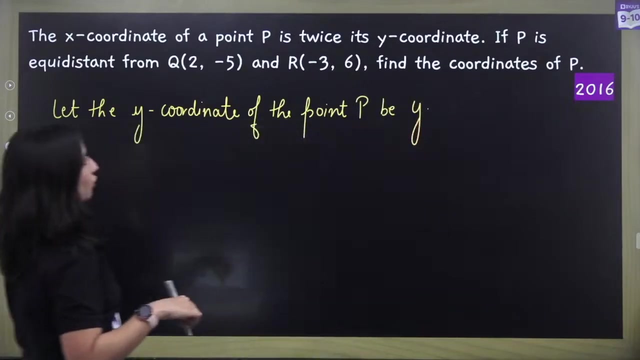 Ma'am, it is saying that x coordinate of a point P is twice its y coordinate. So what we can say is: let the y coordinate of the point P be y. We have assumed the y coordinate as y. Therefore, what can we say? what is the x coordinate of the P point? 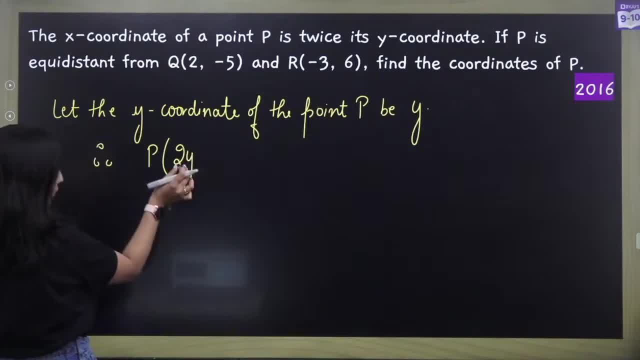 It is twice the y coordinate. So instead of x coordinate it will be twice the y, And y coordinate is our y. So our P point has become this: Is it clear to everyone? P has come to us Very good. Now what do we say next If P is equidistant? now, 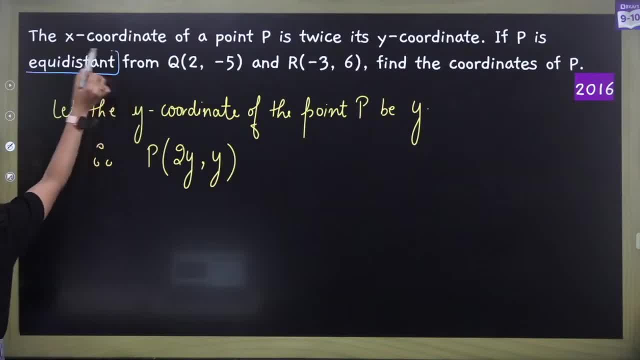 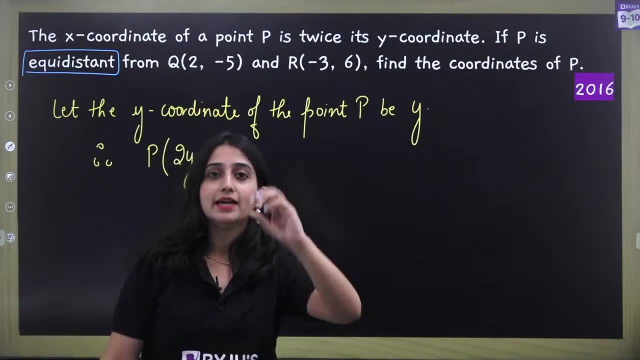 I have used one more term in this question: Equidistant. Do you understand by this term? Do you understand what is the meaning of this term? Yes, Equidistance means equal distance. Okay, You can understand from the name itself. Equi means equal, distant means distance. 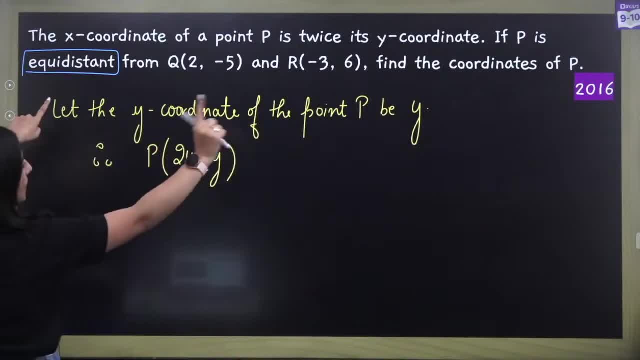 So those who are at equal distance. it says this: P point is equidistant From Q and R. It means P point is at equal distance From Q point and R point. If P point, assume that this is my P point. So if I make Q point here and R point here, 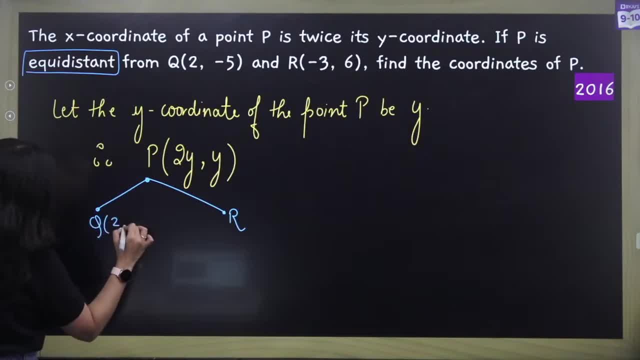 So basically it is trying to say that this is my Q point, that is 2 comma minus 5.. And my R point, that is minus 3 comma 6.. These two are at equal distance. That means, according to the question, 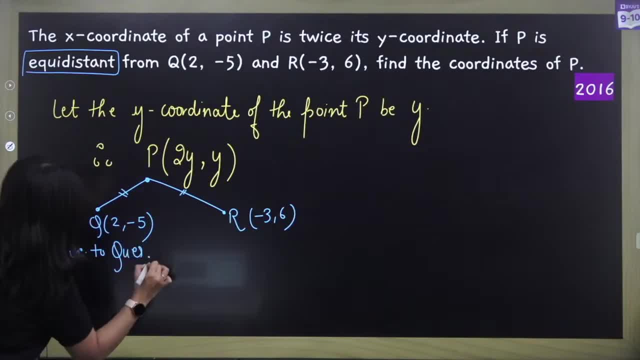 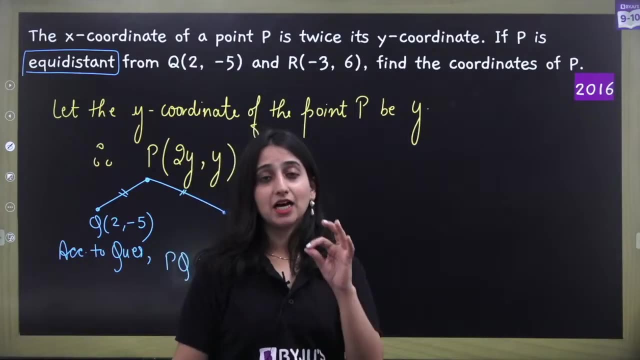 you can say that, according to the question, you can say that distance PQ is equal to distance PR. Is it clear to everyone? If it is equidistant, then PQ will be equal to PR. Did everyone understand? Now, children, do you know what they do? Listen to me. Some children do a blunder here, do a silly mistake. 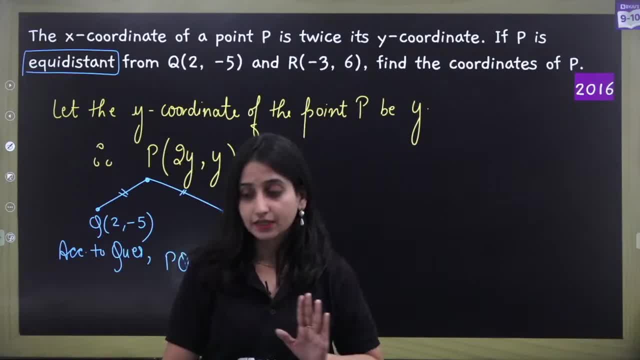 Here they will consider P as midpoint, which is not Okay. What will some children do After reading equidistant word? they start applying midpoint formula, which is wrong. Okay, He did not say that these two points lie on the same straight line. 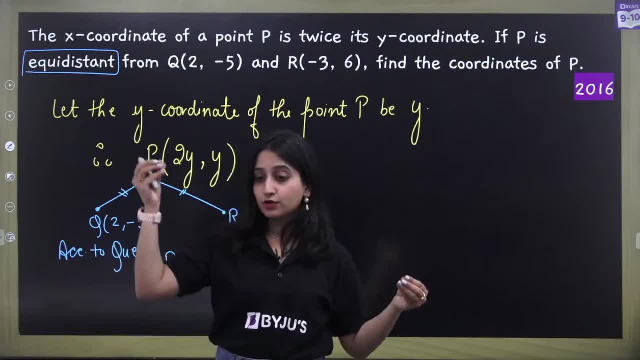 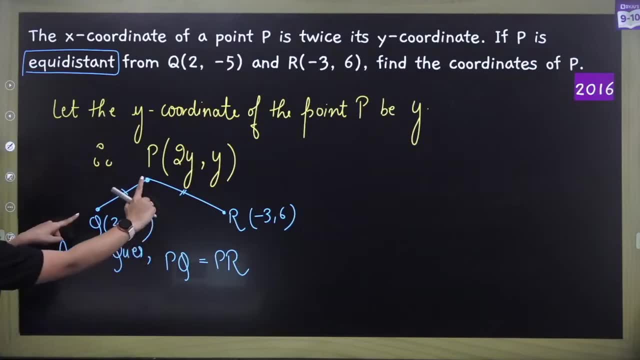 He did not say anything like that, right? Okay, These two points can be anywhere, So you do not have to take out midpoint here. Right Here, distance formula will be applied That distance of P and Q is equal to distance of P and R. Okay, So PQ equals to PR. 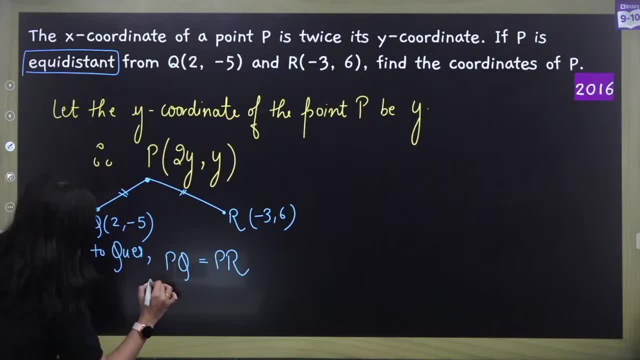 So what does distance formula say? Distance formula says: let's do squaring of both of us, Squaring both sides. Why did you do squaring? Because in distance formula root comes, we do squaring, root will disappear. 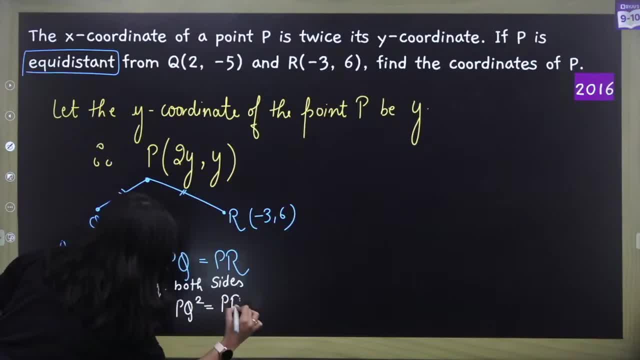 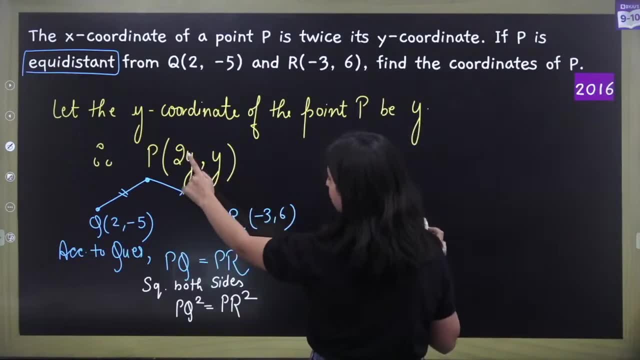 So it will become: PQ square equals to PR square. Come on Now, quickly put the values and give me the answer. How will PQ come out? X2 minus X1 square, that is, 2Y minus 2 square plus Y2 minus Y1 square. 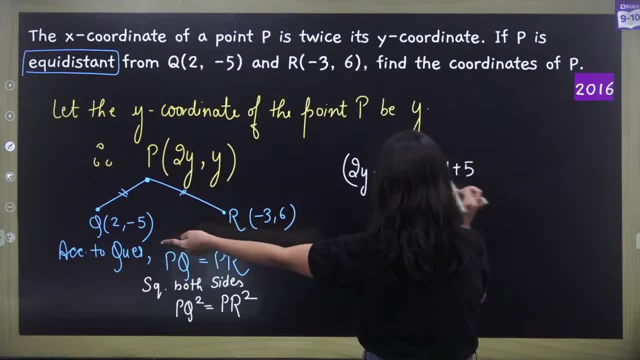 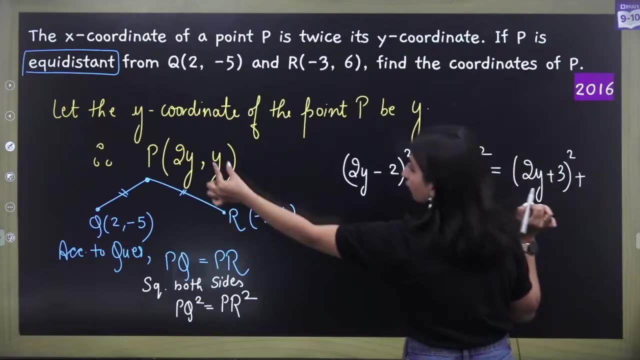 Y minus of minus 5 will be Y plus 5 square, Don't make a mistake of sign. equals to Now put the distance formula of both of them: X2 minus X1, minus both of the X coordinates: 2Y minus of minus 3 will be 2Y plus 3 square plus Y2Y minus 6 square. 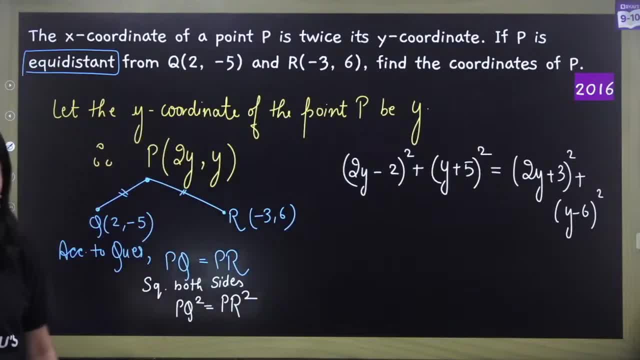 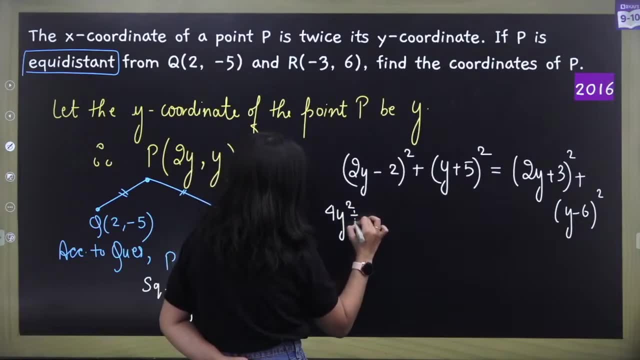 If someone has got the answer, then you can tell me. Has anyone got the answer? Yes, child, Come on, Let's open the brackets. So this will become A minus B whole square, That is, 4Y square plus 4.. 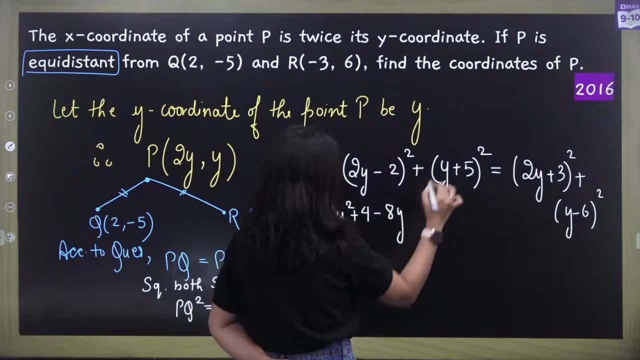 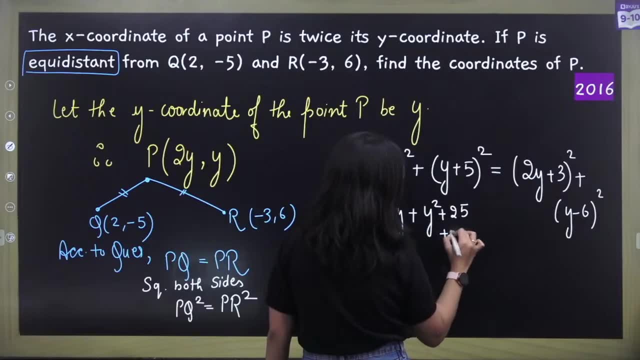 This is minus 8Y, Okay. Plus- Let's open this too- Y square plus 25 plus 10Y. Right, What is coming on the right-hand side? Look, 4Y square plus 9.. 3 to the 6 to the 12Y. 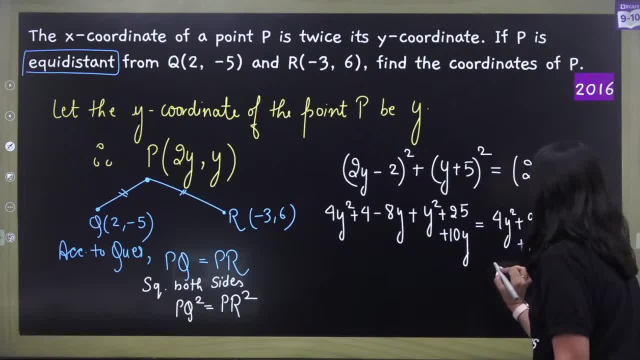 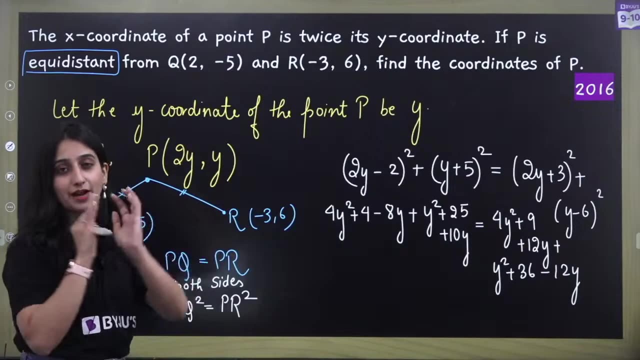 Plus 12Y plus Y square, plus 36 minus 12Y. Is it matching? Tell me, Is it written correctly? Are you able to match? Yes, everyone is matching. There are chances of silly mistakes here, So open the brackets carefully. 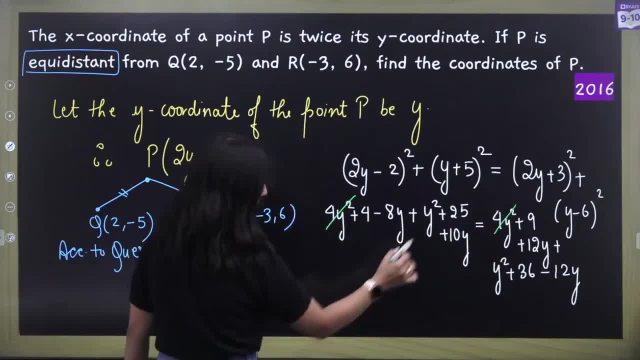 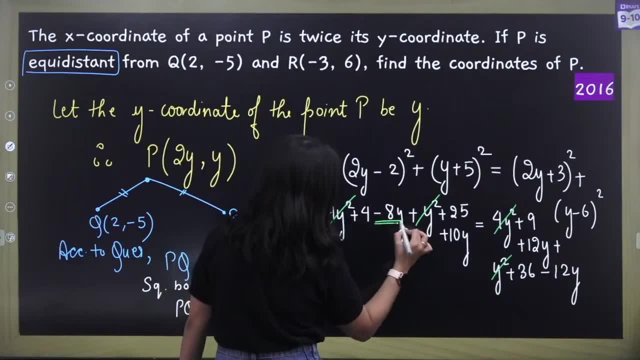 Okay, 4Y square. 4Y square is cancelled. Y square is on the left-hand side also. Y square is cancelled on the right-hand side also. What else You have here? minus 8Y, plus 10Y. So how much will this become? 10 minus 8.. This becomes 2Y. 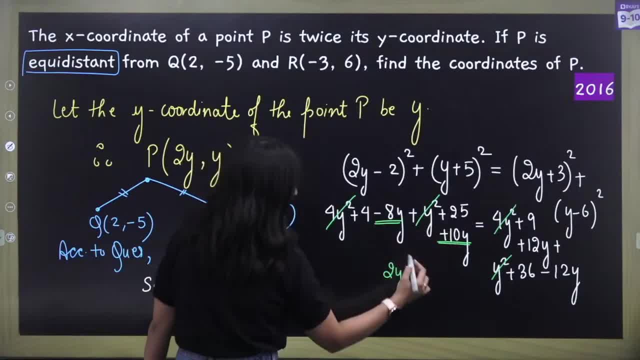 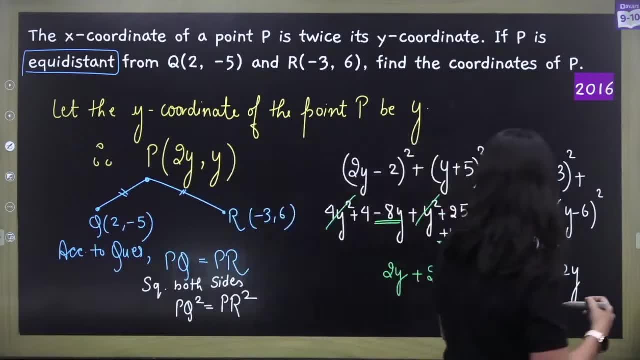 Here is 4.. Here is 25.. This becomes 29.. So I have written 29 here Equals to What is coming on the right-hand side. Look What is coming on the right-hand side. This plus 12Y, minus 12Y, is cancelled. 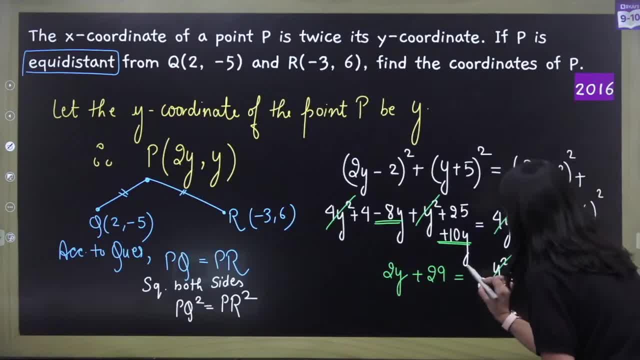 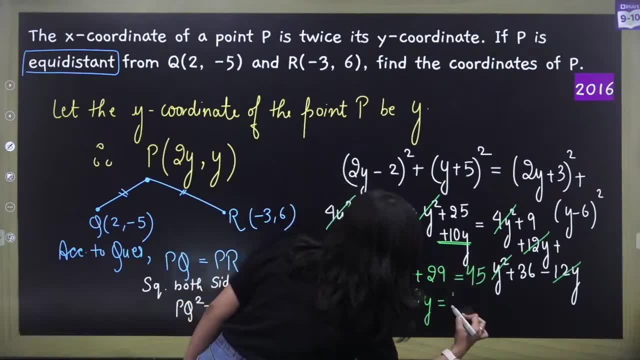 36 plus 9.. What is this? This becomes 45.. Okay, So this is our equation. So you have 2Y equals to 45 minus 29.. That is 16.. So Y equals to 8.. 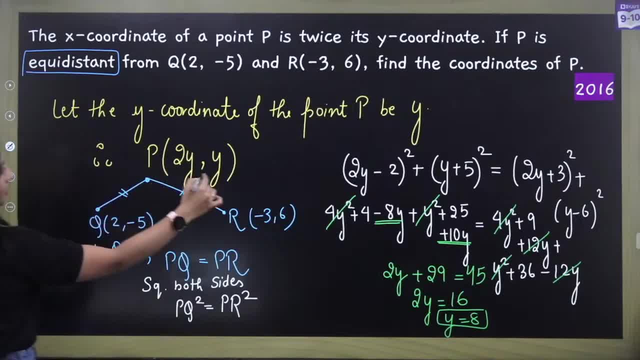 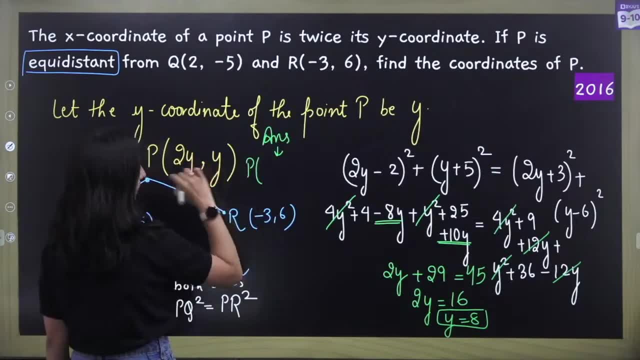 Dear. if the value of Y is 8,, then what will be our point? What will you give the final answer? What will you say in the final answer? The key point is: if Y is 8, X coordinate will be 8 into 2.. 16 and 8.. So this is your final answer. 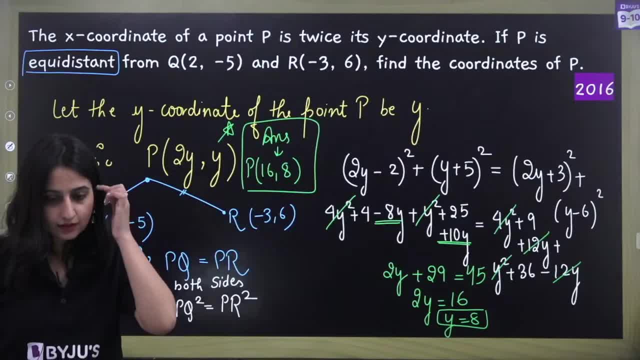 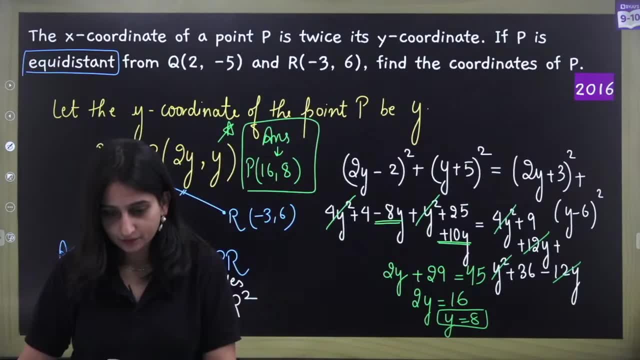 Is it clear to everybody. Yes, NCRT of Geometry is enough. Yes, NCRT of Geometry chapters is enough. Yes, Rachi, what is the square of root 2?? Look, if you do root 2 into root 2, then the square root goes away. It becomes 2.. 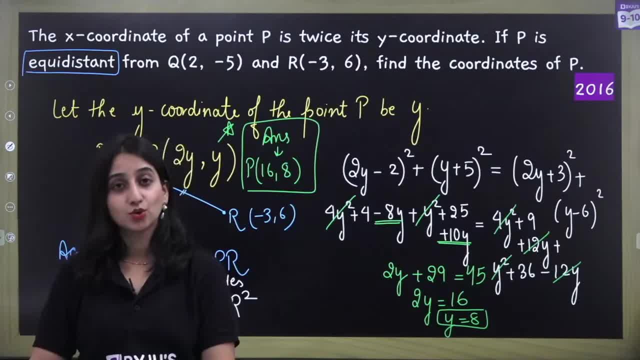 Root 4 into root 4 becomes 4.. Root 6 into root 6 becomes 6.. So when you square a number with a root then the root gets cancelled out. So in the distance formula there is a root, So I did not feel like writing the root here. 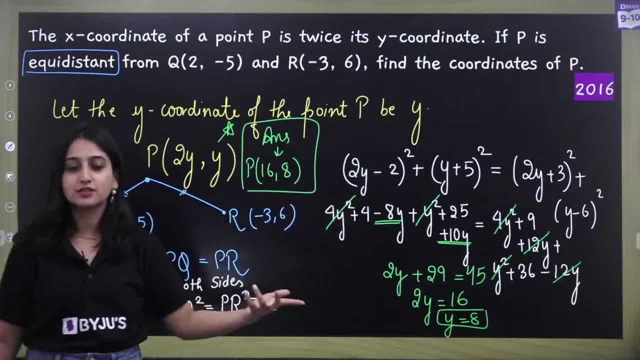 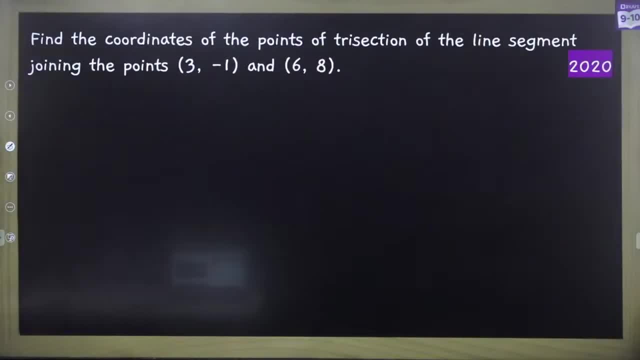 So I did its squaring so that I do not have to write the root Calculations seem easy. Okay, Let's move to the next question, Question number 3.. Look carefully, Find the coordinates of the points of trisection. 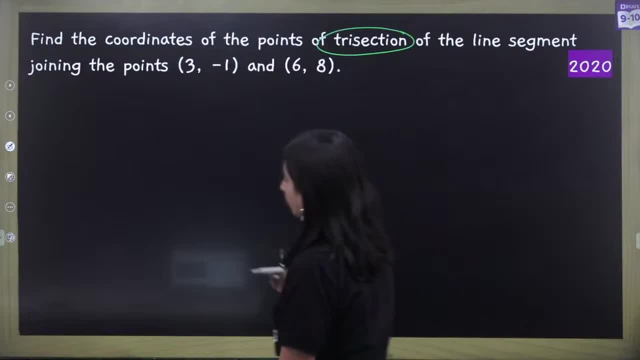 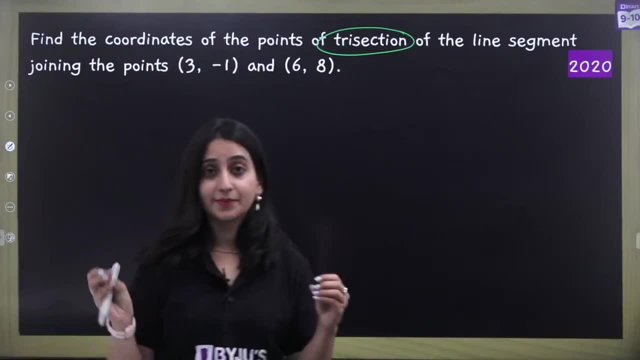 Now there is a new word hidden in this question: Trisection. The student who has solved NCRT well will know, By the way, what is the meaning of trisection When a line segment is divided into 3 equal parts. 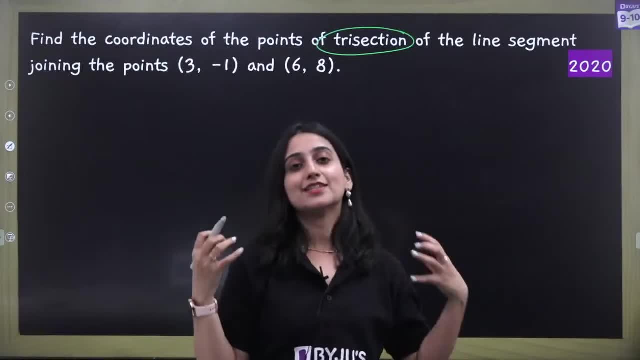 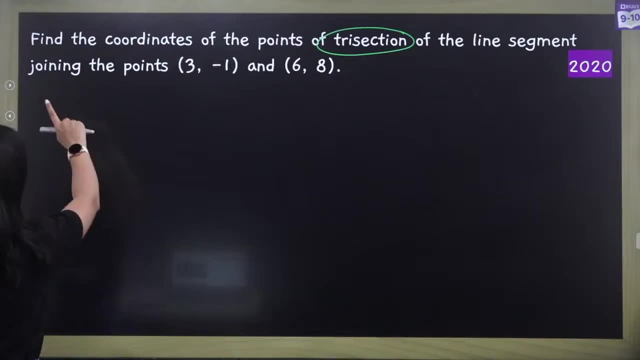 This means that that particular line segment is trisected Right. So trisection means dividing a line segment into 3 parts. Okay, Joining the points. What does joining the points mean? We are making a line segment by joining these two points. 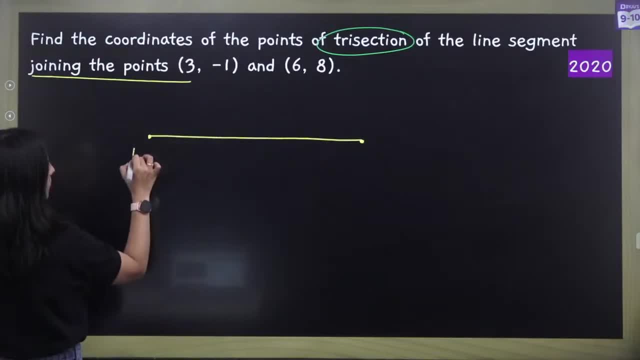 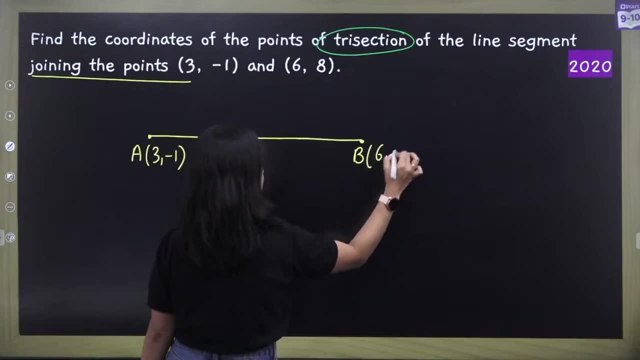 So let's make a line segment. I have made this line segment Point. I have given the name of 3 comma minus 1 as A. Let's name the other coordinate as B, That is 6 comma 8.. If this line segment AB is getting trisected, then there will be 2 points in between. 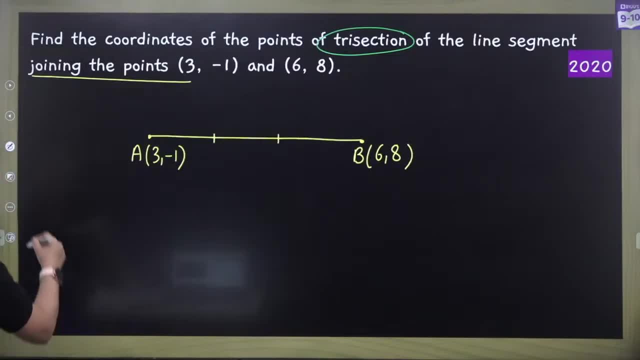 So divide it into 3 equal parts. We have to find these coordinates. I think this is an easy question. So we have to find the coordinates of P and coordinates of Q. Can you do that? So let's see Here we can say that P is dividing the line segment in what ratio. 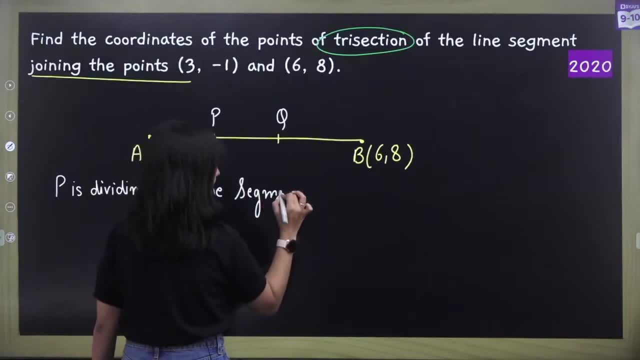 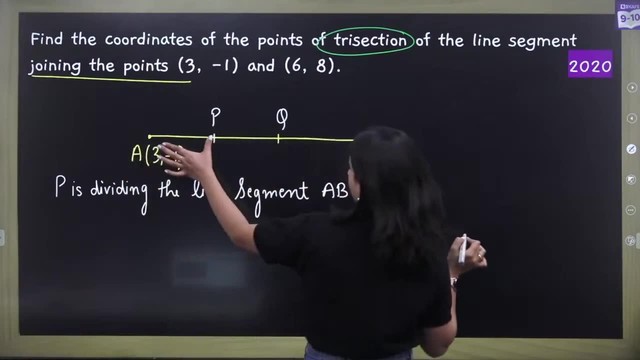 P is dividing the line segment AB. In which ratio? Can you tell me Line segment AB? in which ratio? In ratio, this is 1 part, This is 2 part, So 1 is to 2.. In ratio, 1 is to 2.. 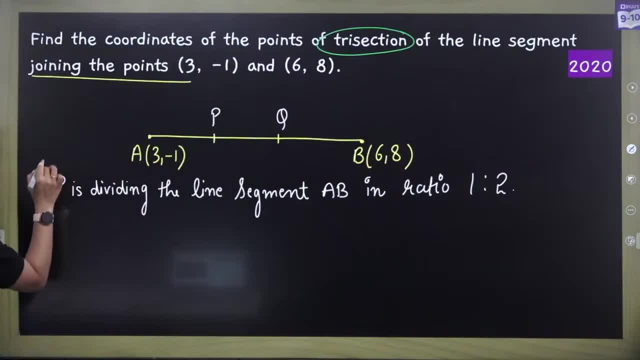 Do you agree with this line? Are you agreeing with the statement which I have written here That this P point is dividing the line segment AB? in which ratio? Because all these 3 parts are equal. So on the left hand side I have 1 part. 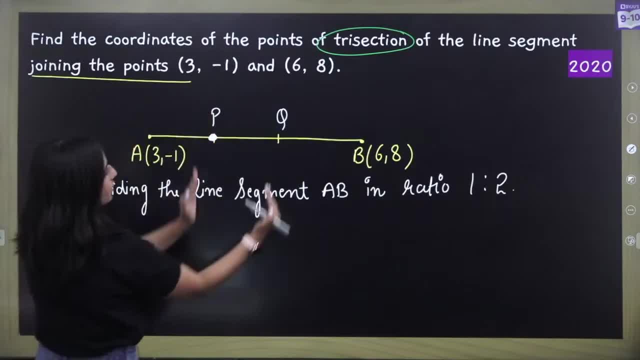 On the right hand side I have 2 parts, So the ratio becomes 1 is to 2.. Is it clear to everyone? Yes, Very good, So we got the ratio. So can we apply section formula now? 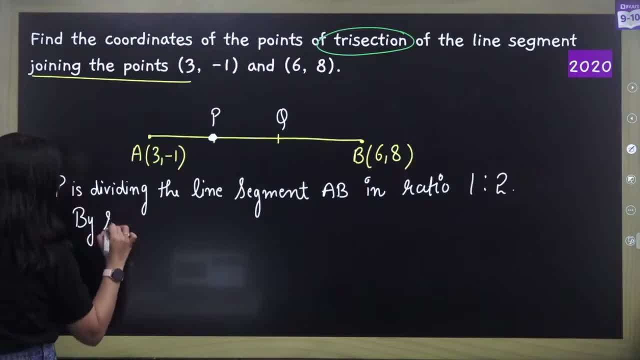 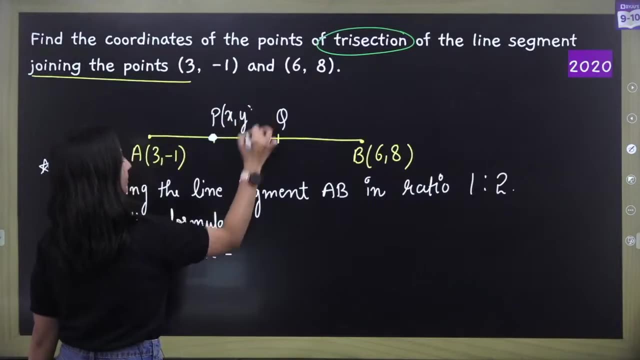 So by section formula, what will you say? By section formula, we can find the coordinates of this point P. So let's apply section formula. So let's assume that its coordinates are: So x will be equal to. if this is, 1 is to 2.. 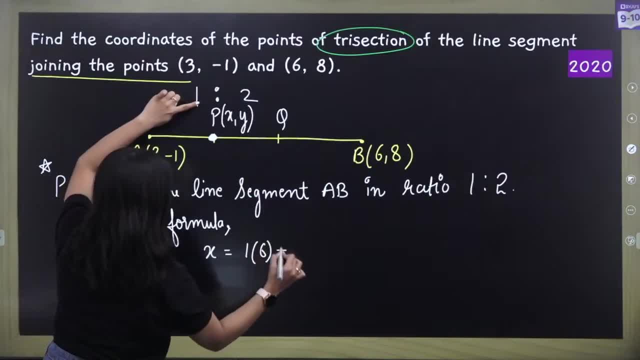 So first we multiply 1 with x 6 plus 2.. We will multiply 2 with this x 3 divided by ratio's sum, That is, 1 plus 2.. So what will be? x 6 plus 6 upon 3.. 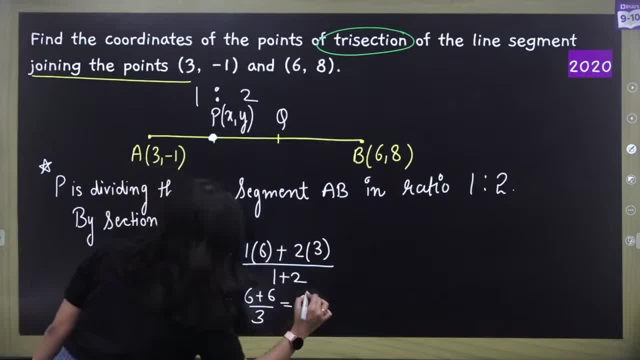 So this becomes 3.. 4 is the 12th. Similarly, what is y? What will be y? Can you tell me, yes, What will be the value of y? Y will be: first: multiply 1 with y. 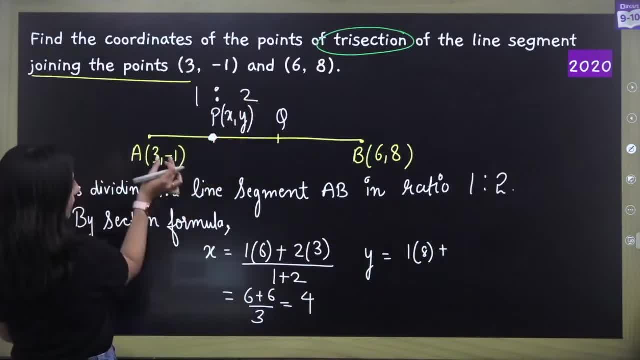 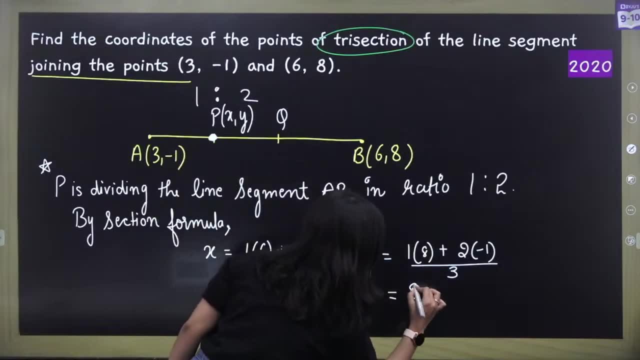 8 will be there, Plus 2 is here with y coordinate. 2 into minus 1 will be there, Divide by 3.. So this will be 8 minus 2 divided by 3.. That is 6 divided by 3.. 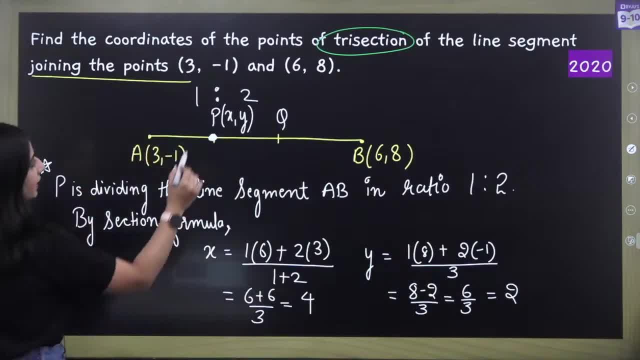 That is 2.. So what is this point This P point is coming out to be? Can you tell me? It is 4 comma 2.. Everyone got 4 comma 2.. Yes or no? So P point is sorted. 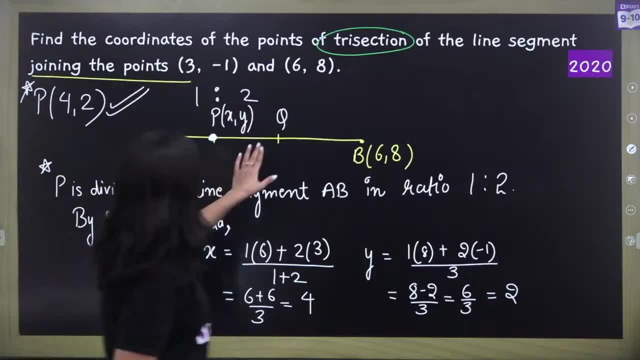 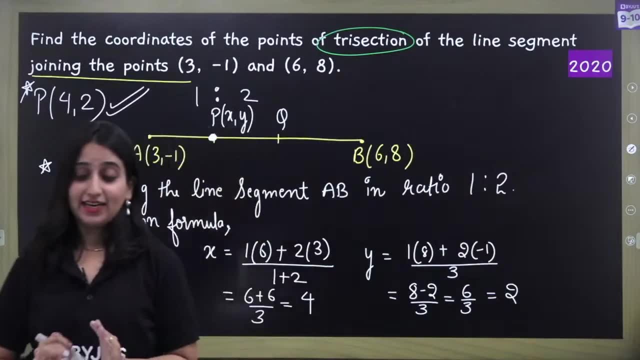 You have got one answer. Okay, how will you get Q? To get Q, we have to apply section formula. For that, we will apply section formula. Yes, everyone. To get Q- point, we have to apply section formula again. 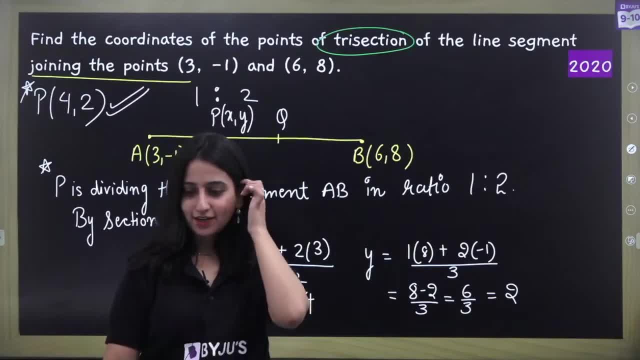 Yes or no, Yes or no? Let's see How many children say yes. See, Some of you are saying yes, ma'am. So look, There is no need to apply section formula again. We can use midpoint formula And we know that midpoint formula is so easy. 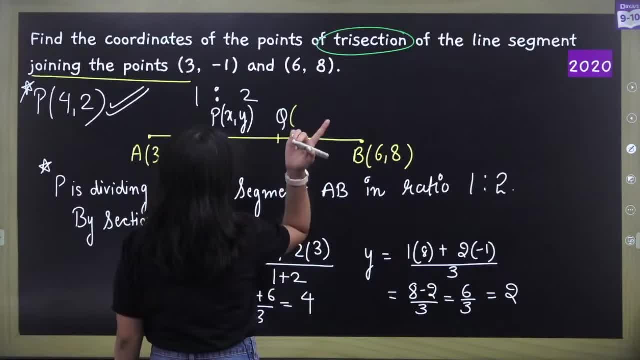 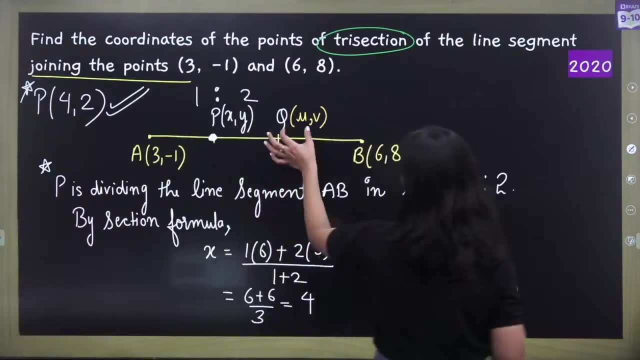 So let's assume that we give the name of Q, point U, comma V, So to get Q coordinates, why do we have to apply section formula? ma'am, We can apply midpoint formula, Because its Q will be midpoint only. 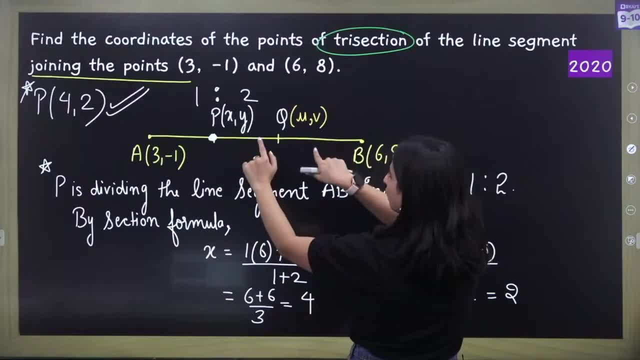 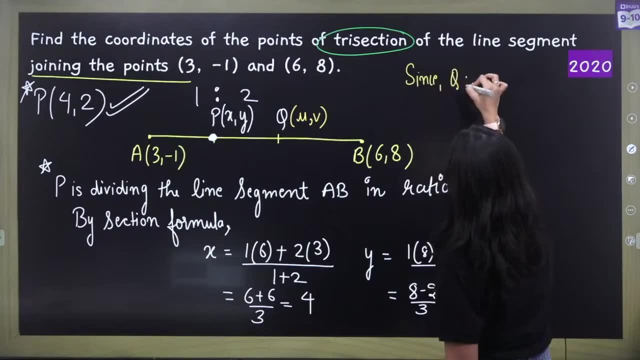 Because these two are equal. So Q is the midpoint of P B. So you can say: since Q is the midpoint of midpoint, of what Midpoint of P B? So to get Q coordinates we will apply midpoint of P B. 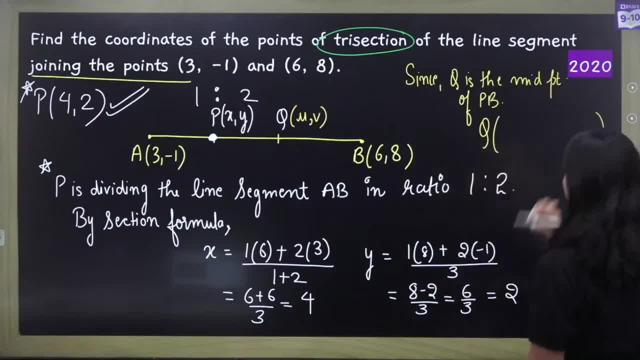 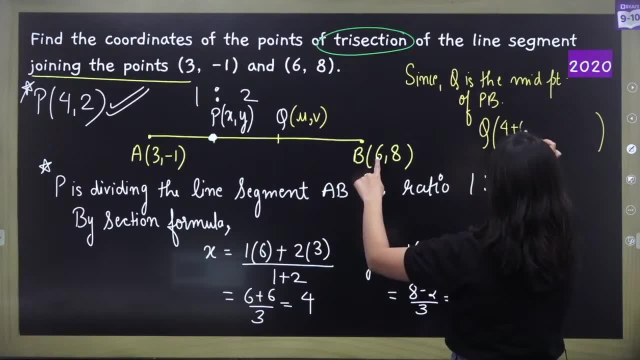 So to get Q coordinates we will apply midpoint of P, B, So we will apply midpoint formula. What does midpoint formula say? x plus 6.. So what was x, Four plus six divide by two, Comma two plus eight divide by two. 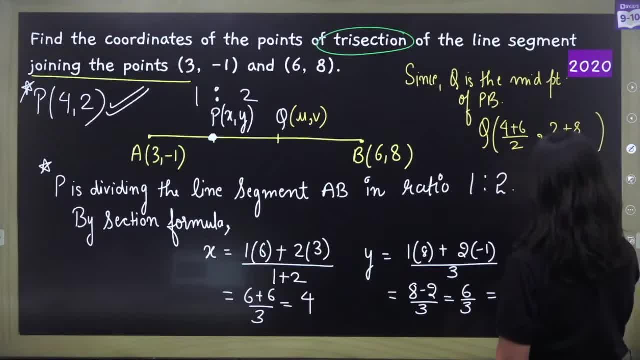 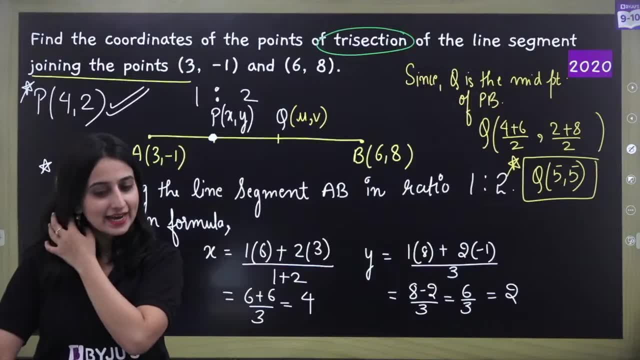 So what comes? Q coordinates came? I have five comma five. Does everyone have five comma five? See how easy the question will be. There was no need to apply section formula again. Yes, Unsure, We applied midpoint formula. son. 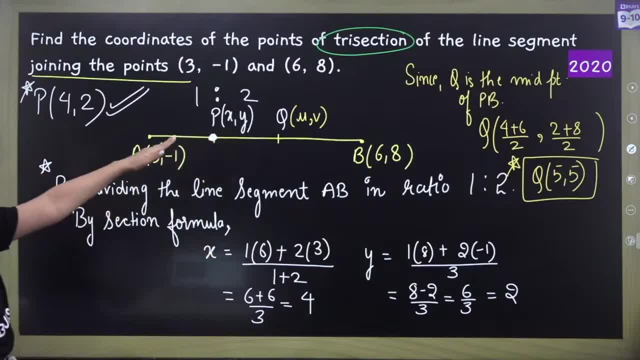 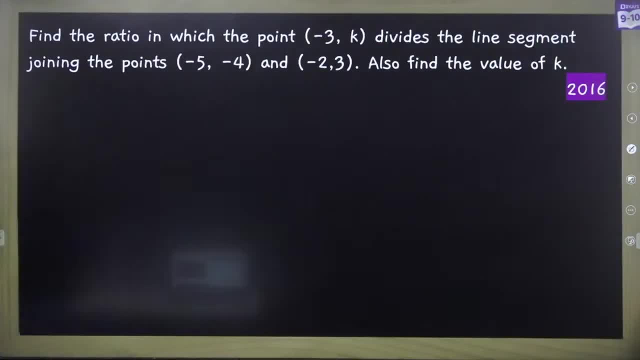 Ok, So I hope this question is clear. Look, it was asked in 2020.. Last year, only this fresh question was asked to you. Okay, kids, Now let's move to the next question. Come, let's move towards the next question. 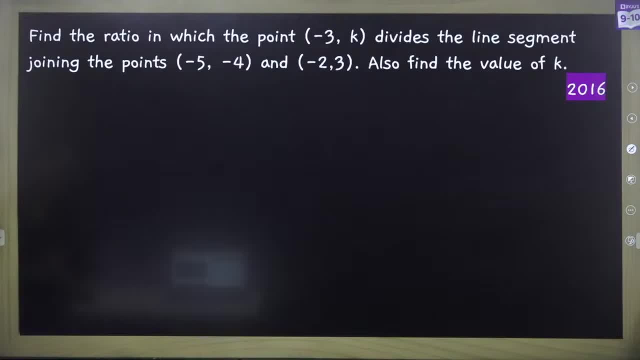 Find the ratio in which the point minus 3, K divides the line segment joining these two points. Also, find the value of K. Can you do that? Yes, How many of you can answer this question? Yes, kids. So wherever. at any point, if you are missing something, make sure you rewind and then re-watch the question again. 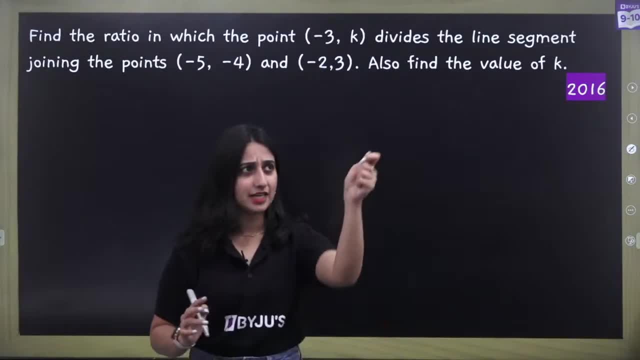 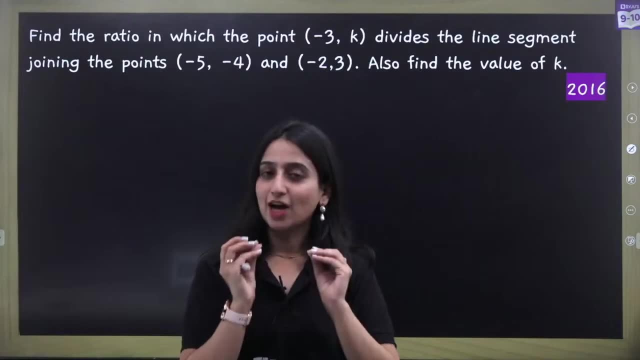 You will understand everything, Okay. So wherever you feel that I did not listen to this, I missed it, I lost my focus here and there, and ma'am explained the whole question. So just a humble request for everyone: Go back a little, look again. 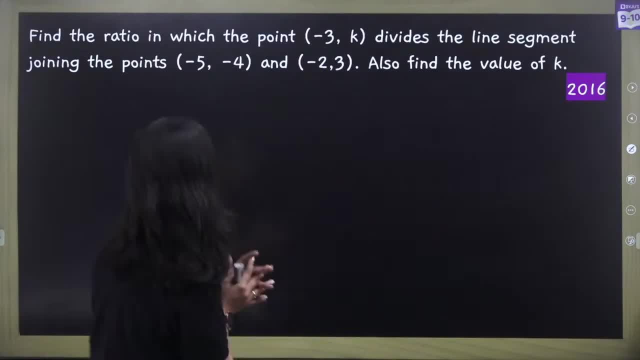 I guarantee you you will understand. Okay, Come on, let's do this question. Let's do this question. Find the ratio in which the point minus 3, K divides the line segment joining these two points. Find the ratio in which the point this divides the line segment joining this and this. 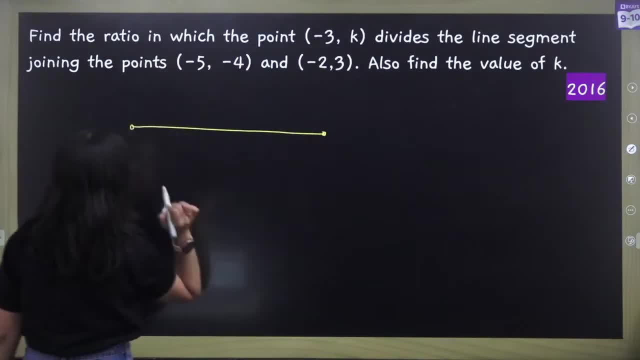 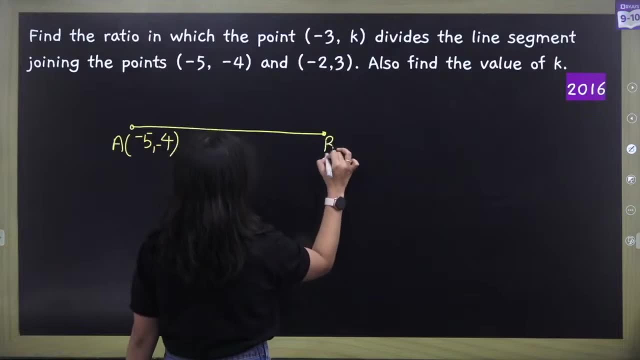 So let's make a line segment joining the points that are given to us. So it is given. A point is: let's say minus 5,, minus 4.. And B point is, let's say 2,, 3.. 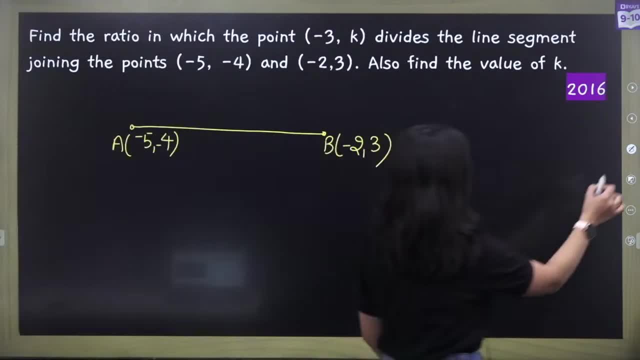 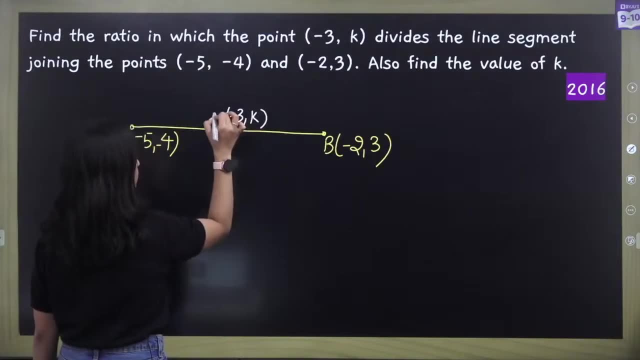 And there is this point: minus 3, K. We have this one point: minus 3, K, Minus 3, K. Let's call it P point. It is dividing the line segment. It is dividing the line segment. 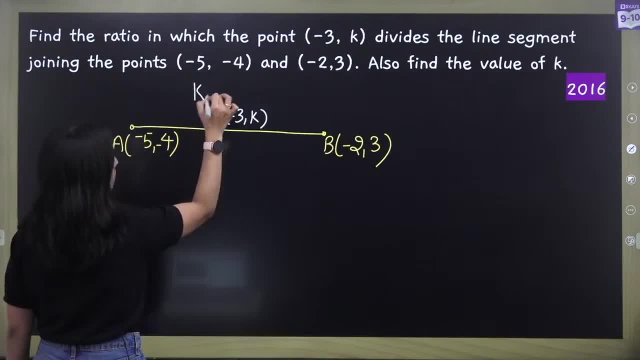 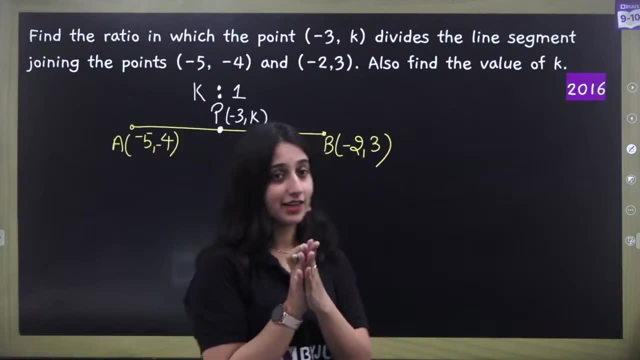 It is dividing the line segment And I don't know what ratio. So I can take the ratio as K is to 1.. So whenever you don't have a ratio, we take the ratio of K is to 1.. Come on, let's apply the section formula. 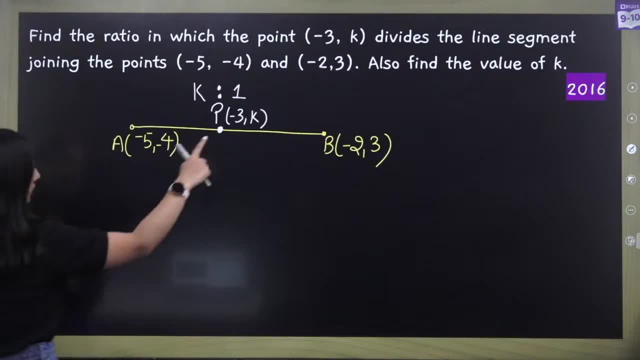 Let's apply the section formula. Alright, kids. So let's apply the section formula. So what will happen if we apply the section formula? We already know X. So what will happen with X By section formula? I think I don't need to write this. 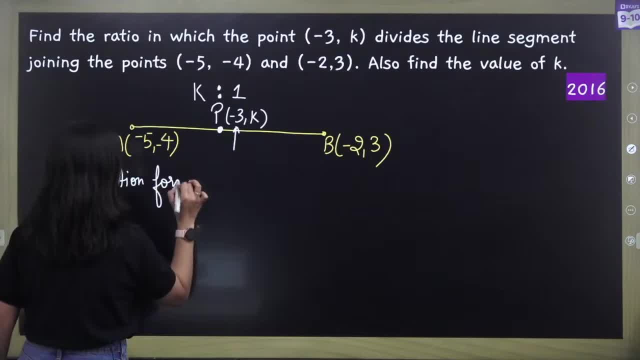 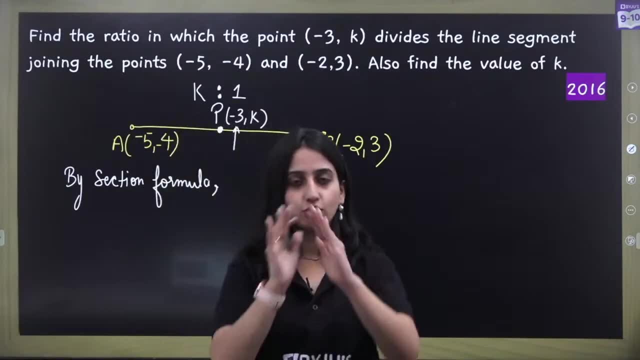 You can write these small things By section formula, By section formula. what will we do See? whenever you have to solve any question in the board, you have to write the formula and put it in the box, So it has extra marks. 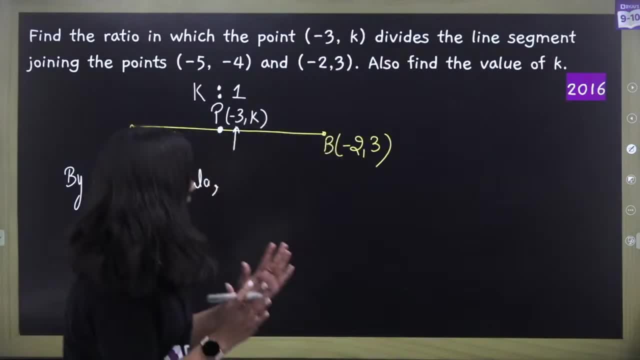 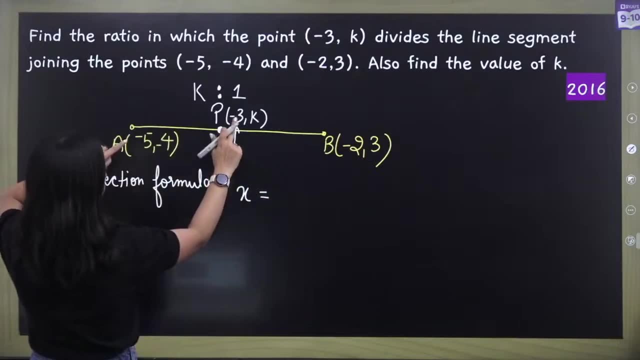 The examiner will know that the kid knows the formula well, So write the formula always To stay on the safe side. Come on whose X will be equal to. Section formula says that this X will be equal to K into minus 2 plus 1, into minus 5 divided by K plus 1.. 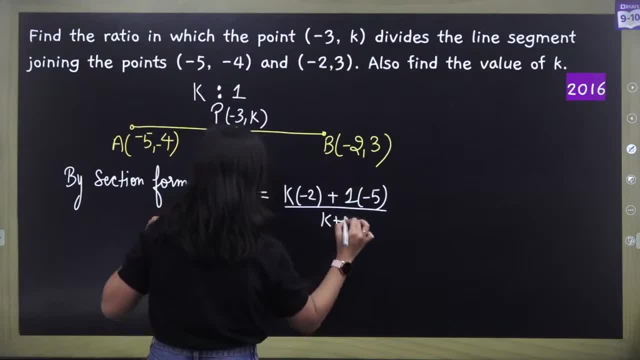 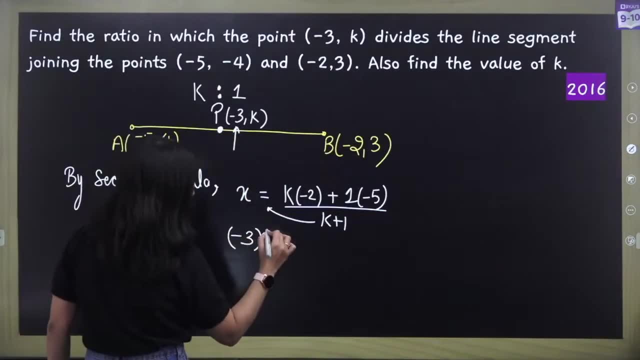 So this is the formula. So this is the formula K plus 1, right. So this X is already given to us. That is minus 3.. So I can put minus 3 here. K plus 1 here will be multiplied by X. 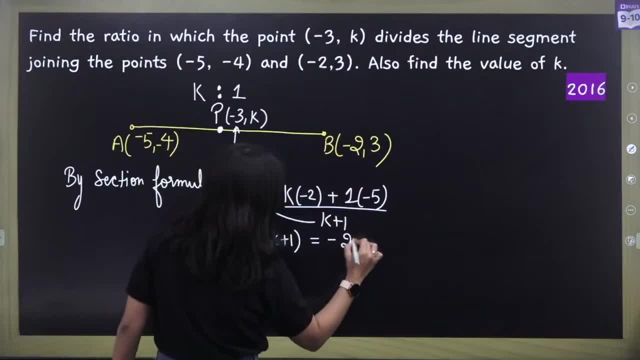 So here K plus 1 will be multiplied. Here it will come minus 2K minus 5.. So what has become? Let's open the bracket. Minus 3K minus 3 equals to minus 2K minus 5.. 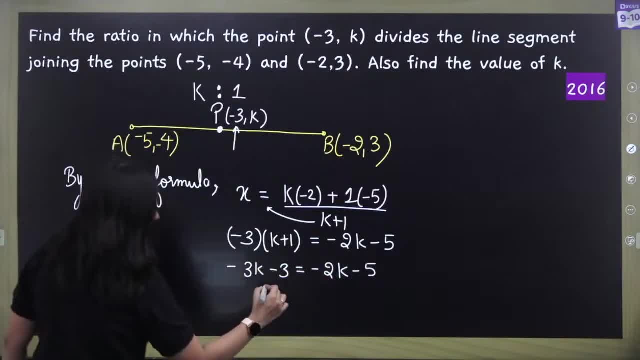 So what is the value of K kids? Let's take 5 here, It will become 5 minus 3.. Let's take 3K there, It will become plus 3K. So you got the value of K 2.. 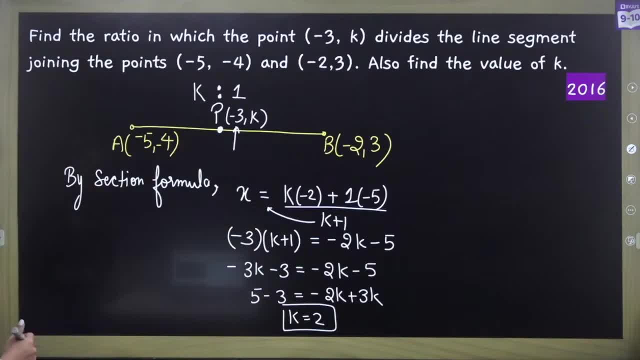 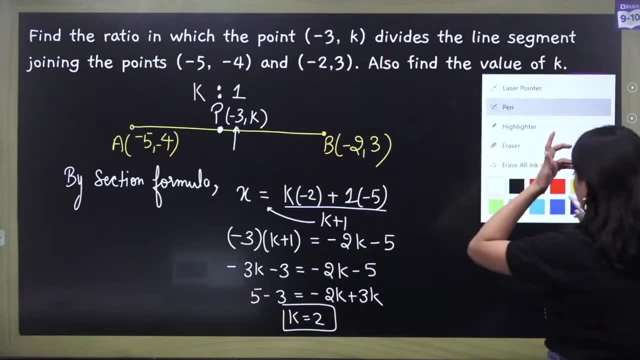 Everyone got the value of K 2.. Yes, If the value of K is 2, then what will be the ratio? 2 is to 1.. After that, you can also get the value of K here. Don't get confused here. 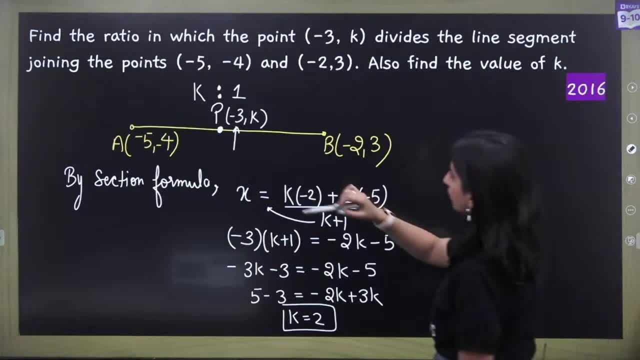 One small mistake has happened, So what will I do to change it? Here we can change this point Or take M, where I have taken K, Because we cannot use two variables. So here I have changed it to M, So that there is no confusion. 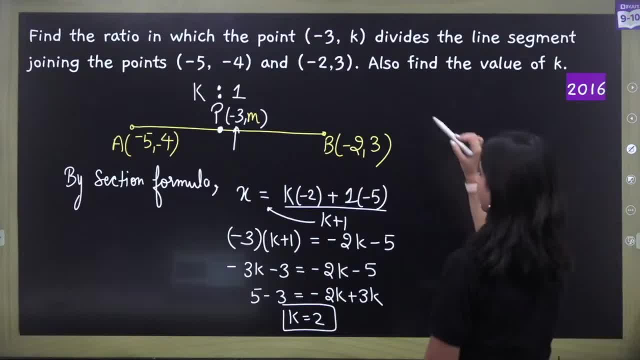 Now let's calculate the value of this M. Okay, How will we do that Now? whose M will be equal to? It will be equal to, Because K has become 2 now. So 2 into 3 plus 1 into minus 4, divided by K plus 1 means 2 plus 1.. 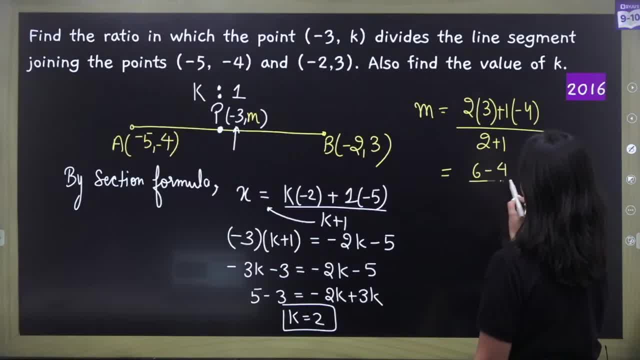 Right, So we have 6 minus 4 divided by 3.. So this becomes 2 by 3.. Right, So our final point: P. So what is our final point? P? Minus 3.. Minus 3, comma 2 upon 3.. 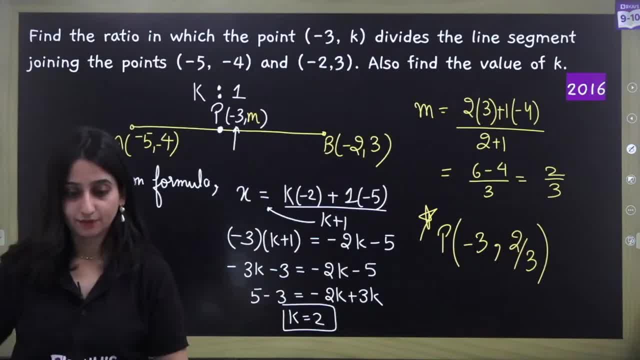 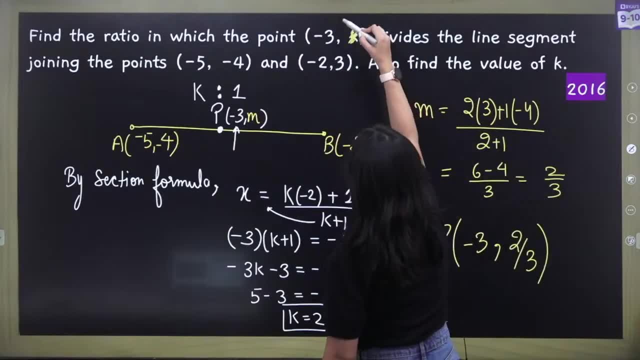 So this is your final point, Which is dividing the line segment. Yes, That is why I said: If already K is given in the question, So let's assume that M is given in this question. Okay, So separate the values according to you. 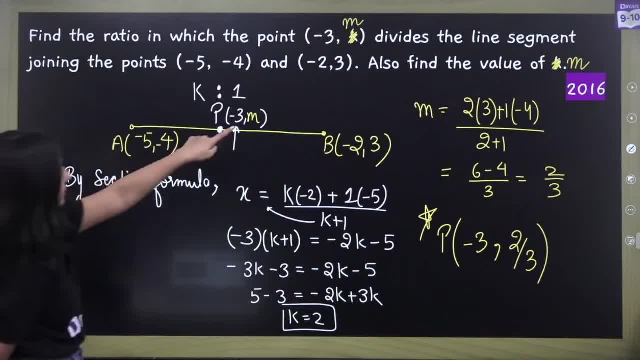 I have taken K, But you separate the values. If you have used K here, take M. If you have used M, take K. Okay, Is it clear? Yes, Is it clear. Yes, Vansh, Come on. 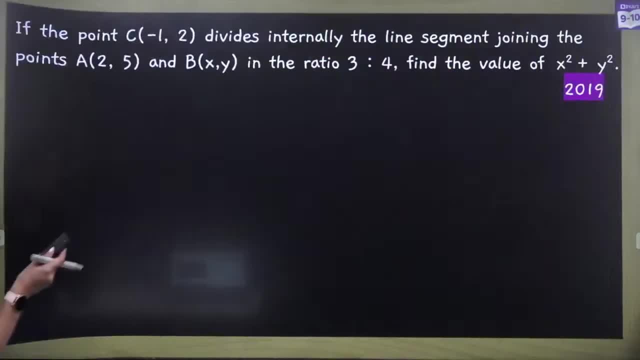 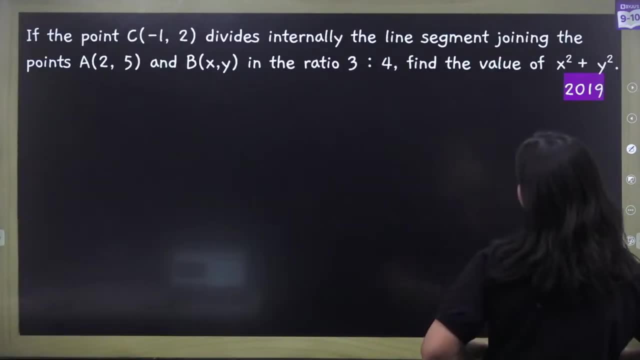 This is how the questions come in the boards. There is proof in front of you. See, I am doing the previous year questions And these same questions are repeated with different values again and again. Next question: If the point C divides internally the line segment joining the points this and this and 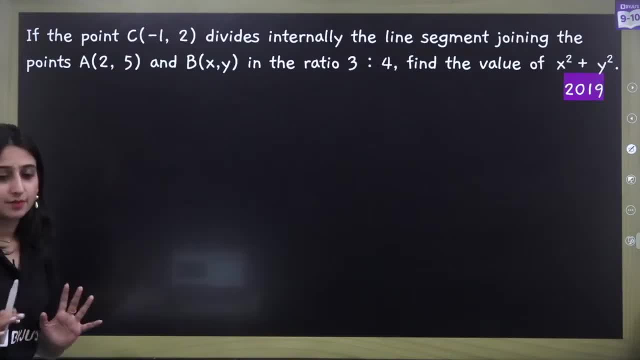 the ratio this: find the values of X and Y. I think you can do this question easily. now You have to apply the section formula on this. also, Ma'am, was P the midpoint? No, Khushi, It was not given to us that P was the midpoint. 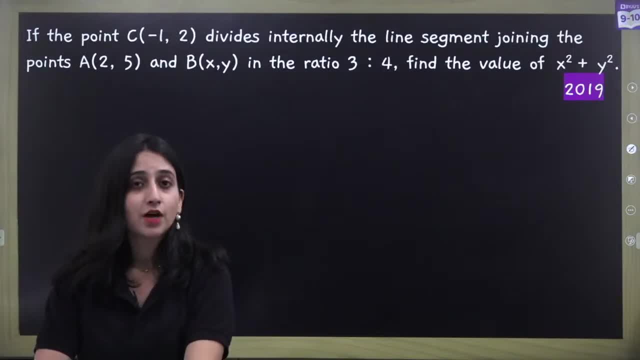 Okay, It was not given, So that is why we have applied the section formula. If he had said that P is the midpoint, then we would have applied the midpoint formula. Okay, That is very easy, Isn't it? Come on. 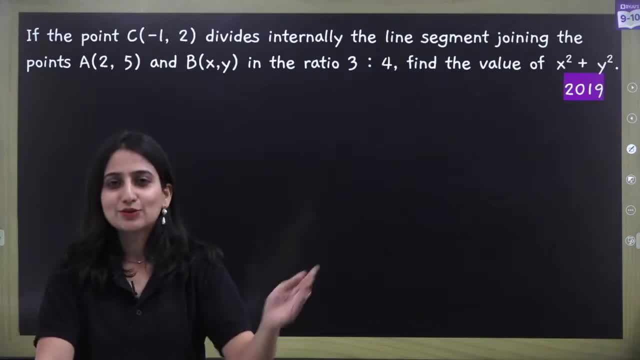 Okay, Let's do this question If C point divides this line segment. So first of all let's make a line segment, Which is the line segment joining the points A. A is 2 comma 4.. So A is 2 comma 4.. 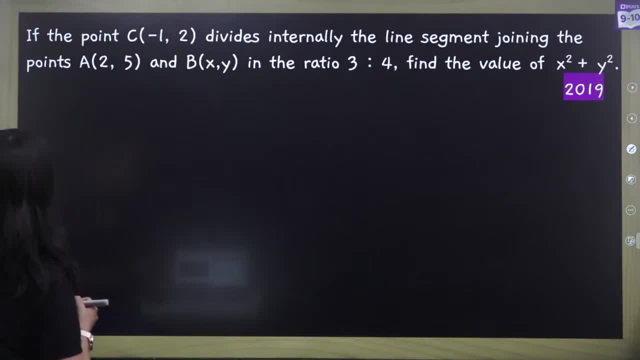 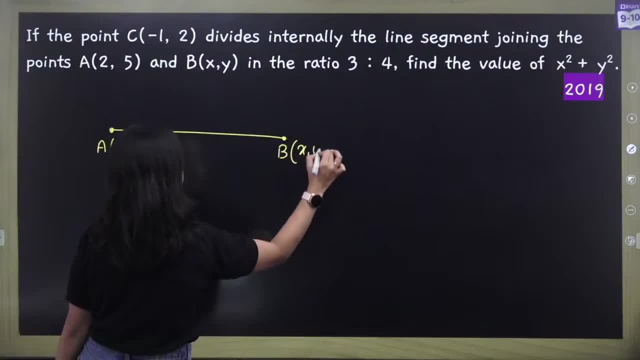 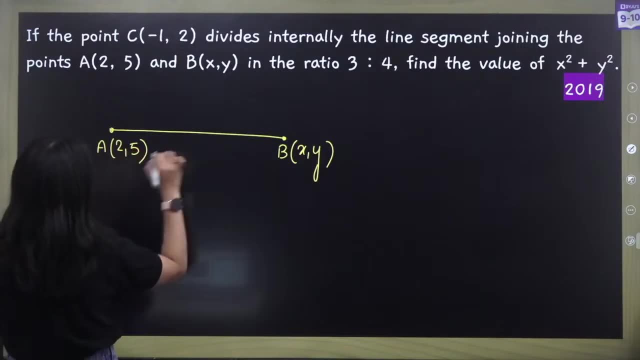 So A is 2 comma 5.. B is X comma Y. Okay, C is the point which is given as minus 1 comma 2.. minus 1 comma 2.. This is point C and in which ratio it is dividing this line segment from this point. 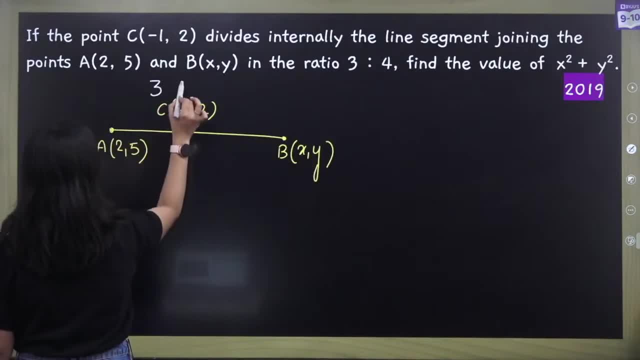 3 is to 4's ratio, So in which ratio it is dividing it? 3 is to 4.. So what is the ratio being divided in? 3 is to 4?. Find the value of the two lines of x square plus y square. 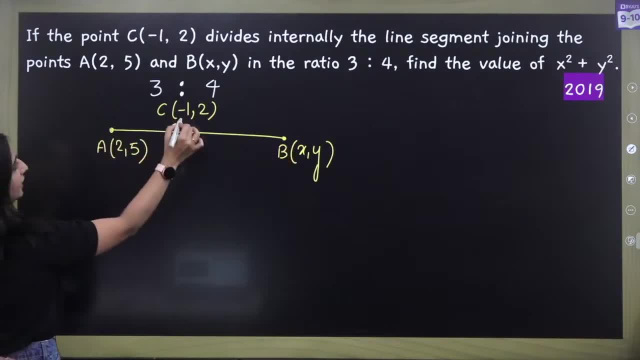 For that we had to apply the value of x- y. Let's apply the same section formula, This minus 1, how will it be equal to? It is x coordinate 3 into. multiply it with x here plus 4 into. 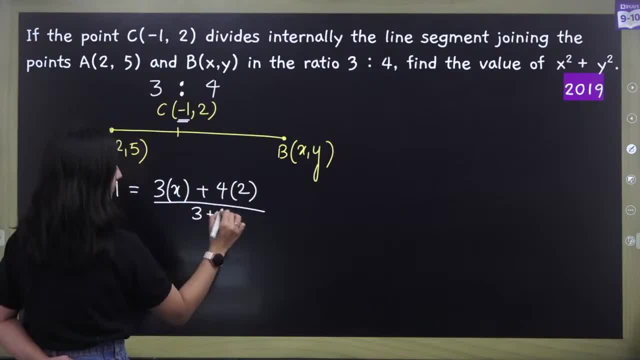 multiply it with x, here divide by both the ratios' sum. So what will this become? 7, here it will become minus 7.. This becomes 3x plus 8.. Okay, So 3x equals to: 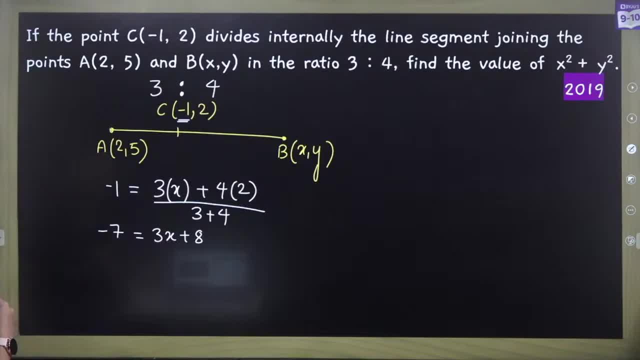 what did you get? You are doing right. you have given: 3 is to 4, only 2 comma 5 is there and minus 1 comma 2 is there. Yes, Okay, Is it clear? So this becomes: 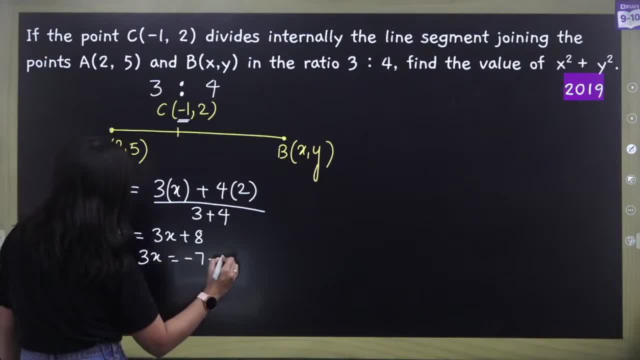 you will get 8 there. this becomes 3x equals to minus 7 minus 8.. So this becomes 3x equals to minus 15.. So the value of x is minus 5.. Absolutely right, Let's go. 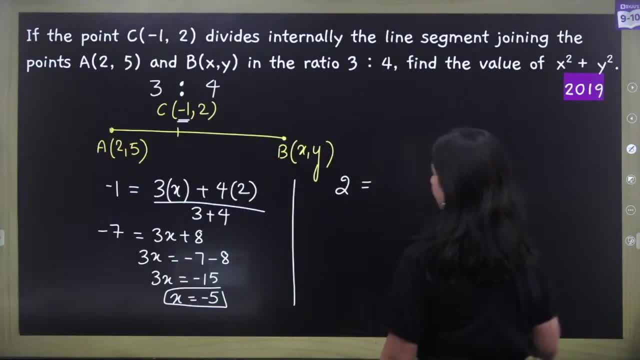 Now let's remove y. We have applied the section formula. What is y? We have already given 2. So we have 3.. So let's multiply y with y here first, Plus let's multiply 4 with y there. 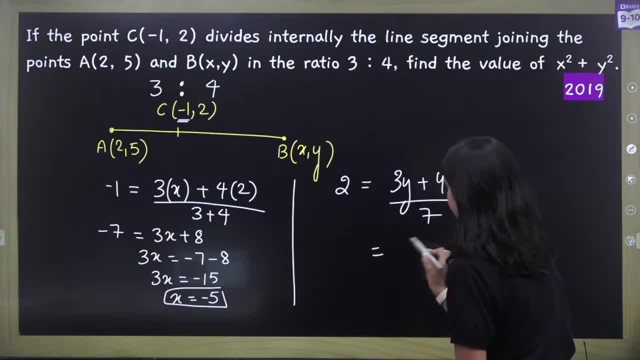 4 into 5 divided by 7.. So what will this become? Here 14 is there, Here 3y will be there, Plus 20.. So here it is. 3y equals to what will it become? 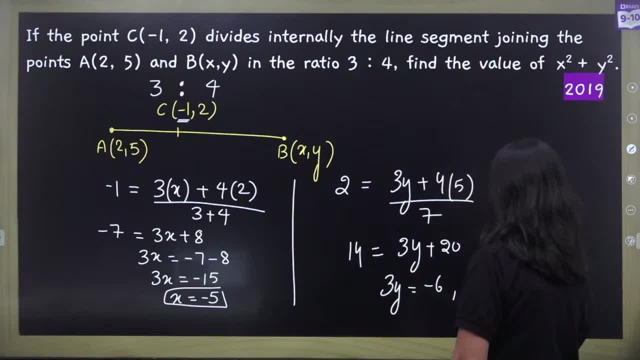 Minus 6.. So we have the value of y Minus 2.. So, how many points do you have? Therefore, how many points do we have? We have x, We have x. We have minus 5.. 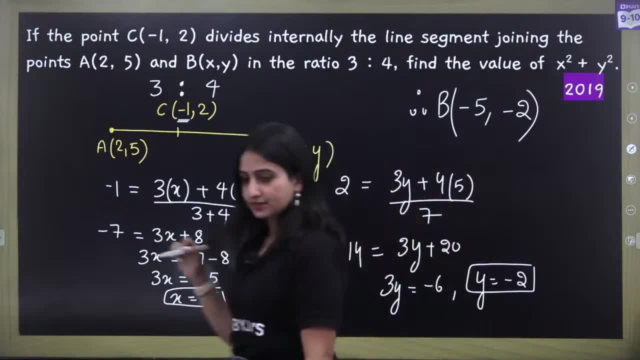 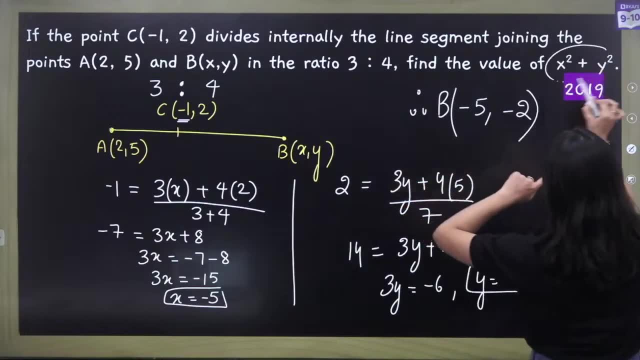 And we have y, We have minus 2.. Is this what everyone is getting? Minus 5 comma, minus 2.. Yes, So this is the b point. But what you had to find, You had to find the value of x square plus y square. 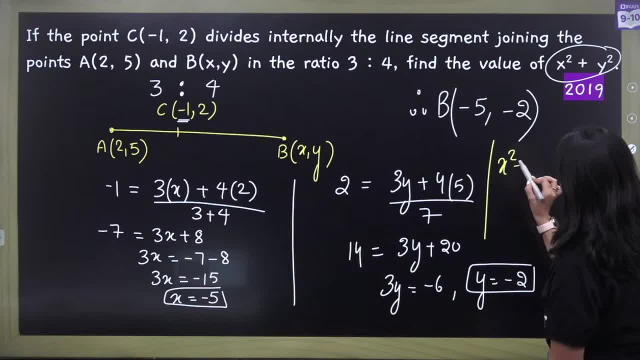 So who will get x square plus y square equal to Ma'am? very easy, I think now you will get this: x square is 25.. y square is 4.. That is, 29 will be our final answer. Clear. 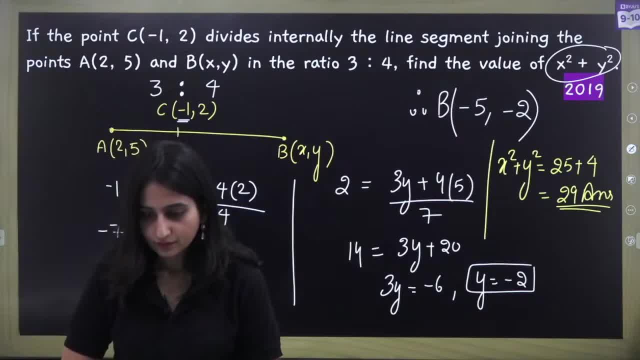 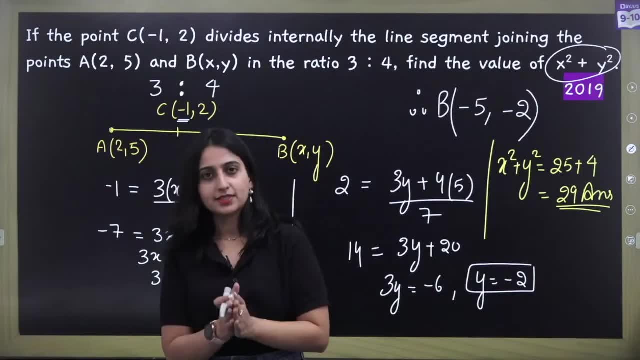 Yes, So this is the b point. So I hope you have understood. We have no more questions. You just have one more question. We will answer it. Draw your карт. Yes, I know we won't get it. What is the number of scores you have got? 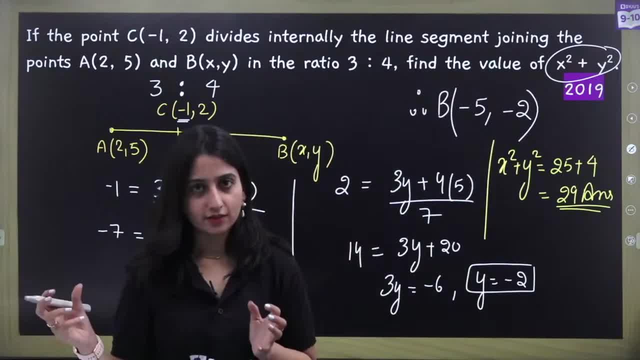 Number of scores. Yes, it is. Yes, I know, I know, I know. So your score is 12.. So what did we get? 12-12 and 3.. Do you remember what we have got? 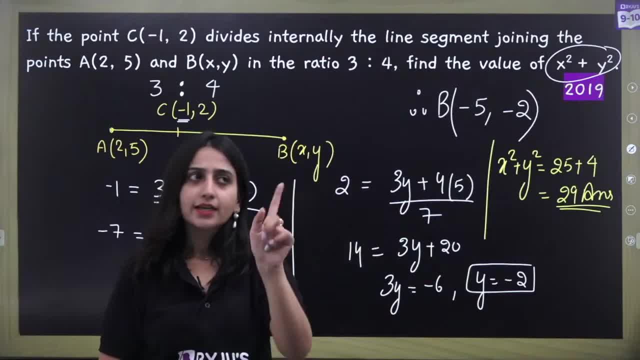 Yes, And you have got 11.. So there is none. I have noticed that 1 minus 2 is 2.. 2 minus 4 is 2.. Yes, Okay, you can use your risk. So you can use your risk. 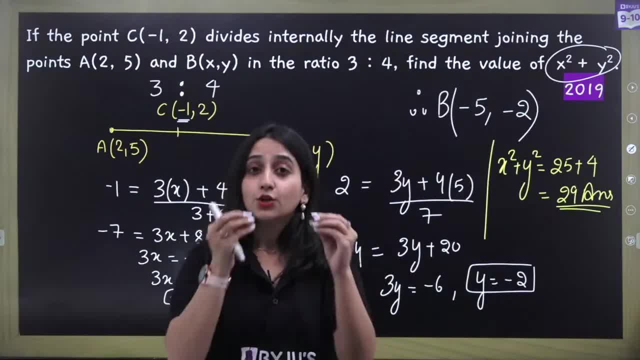 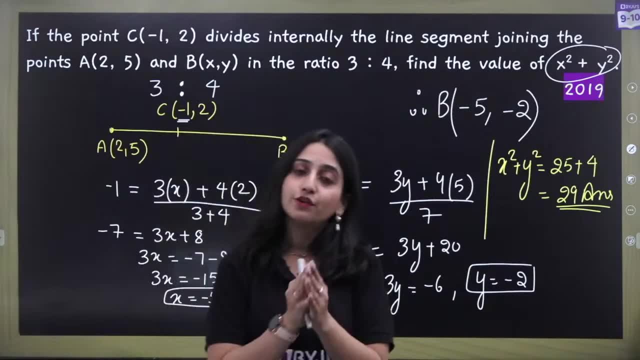 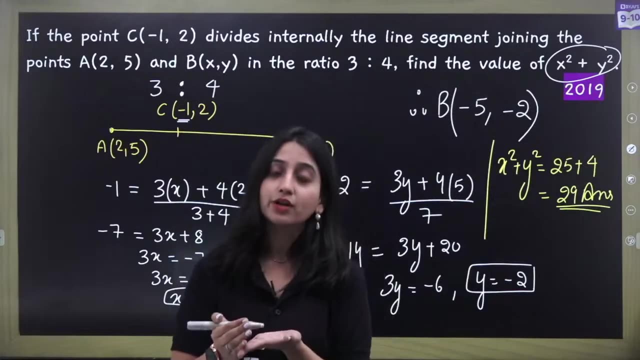 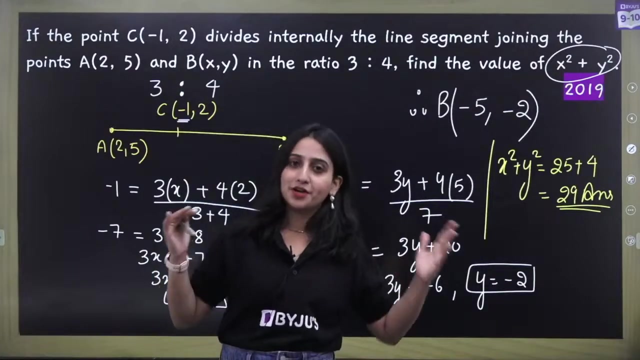 I made a mistake in the steps. I copied the wrong values, okay, so check what mistakes they are, and if they are conceptual mistakes, then you have to revise your concepts. so for that, on the channel you will find all the one shots, all the conceptual videos, right? and if there are silly mistakes, so make sure you are practicing more and consciously don't repeat those mistakes again. and this improvement will happen when you are practicing more and more. okay, so whichever child feels that I am losing my marks. so this is the only thing. 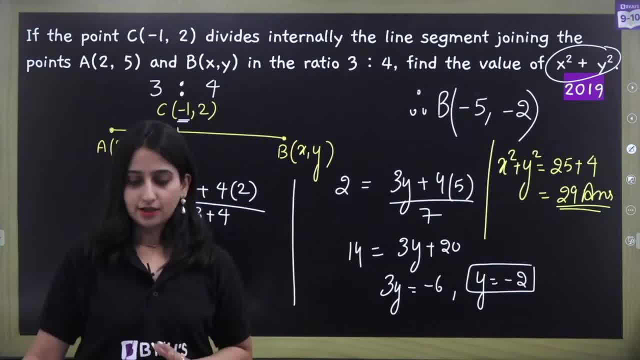 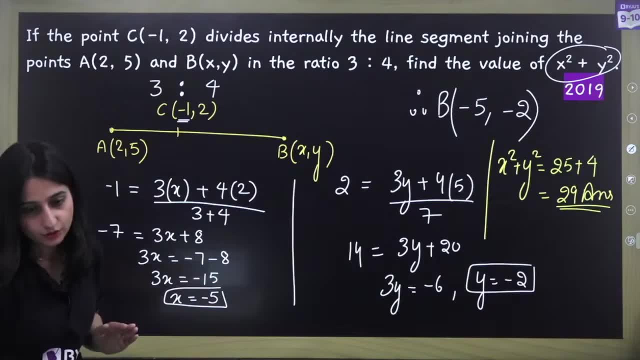 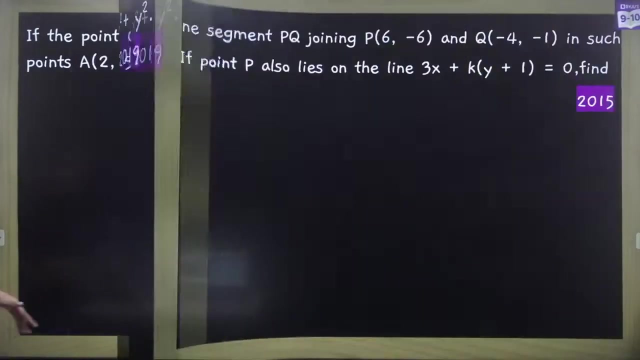 that you can do right now. this is the real way to study. okay, come on, let's see the next question, child. come on, let's move ahead. internally means that there is a division inside the branch. externally means that this point lies outside, it goes outside this line segment. so the concept of externally is not there in this 10th standard. you will go ahead and read it in the 11th. come on. next question on your screens now. who will give me the answer quickly? 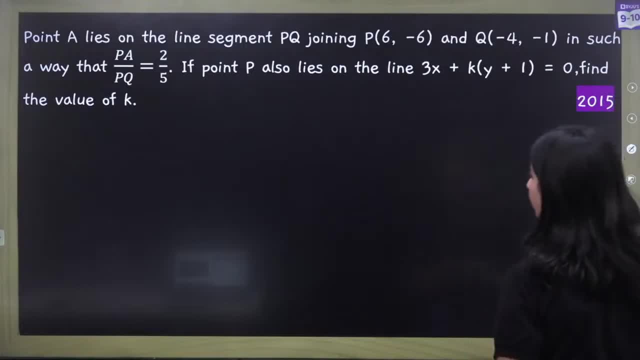 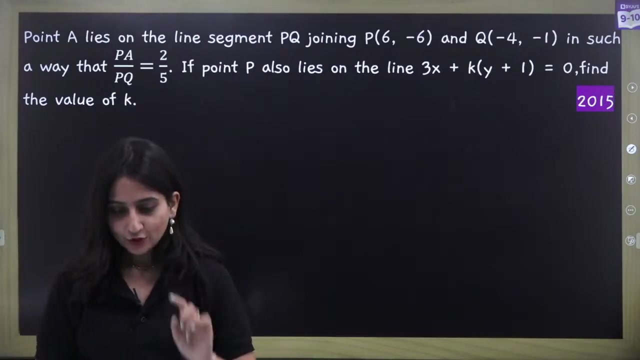 let's see how many children give the correct answer. I am waiting for your replies. point A lies on the line segment PQ joining P and Q in such a way that PA upon PQ is given as 2 by 5, if point P also lies on this line, find the value of K. I think answer is hidden in the question. so I want to see how many children are able to get the answer. 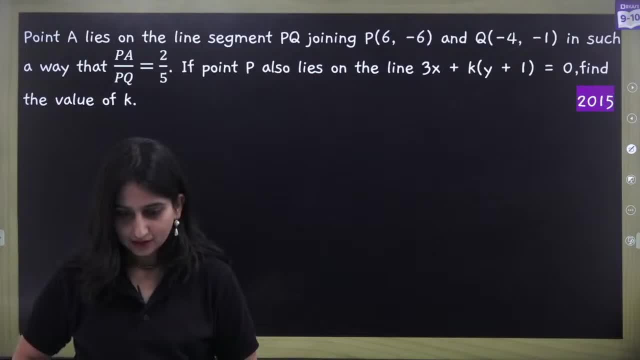 yes, blessings are always with you, Anshul. all the very best for your exam. children, light the fire and come. okay, yes, come on. so let's read the question. by reading the question, it seems that ma'am gave so much, ma'am such a big question. come on, whoever read it carefully, he will understand that this question is just to confuse. the above words are just for talking. it is just a story. 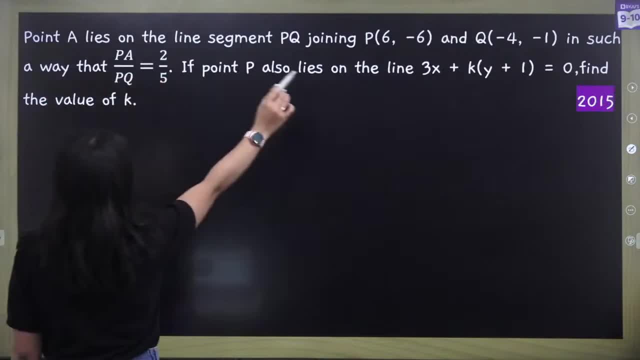 let's go. so see here: point A lies on the line segment PQ. so we have a line segment PQ. I will still tell you the story if you want to hear where PA is such a point. the coordinates of P point is given you have 6 comma minus 6, coordinates of Q point are given minus 4 comma minus 1, the question is in words in such a way that PA- let's assume any A point, let's assume A point. 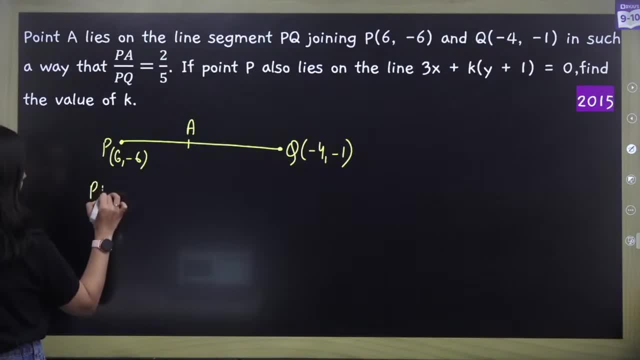 PA upon PQ is A spaghetti: 2 is to 5.. So PA upon PQ's ratio is 2 is to 5.. So if PA is to X, then AQ will be equal to 5 points, 5 units. 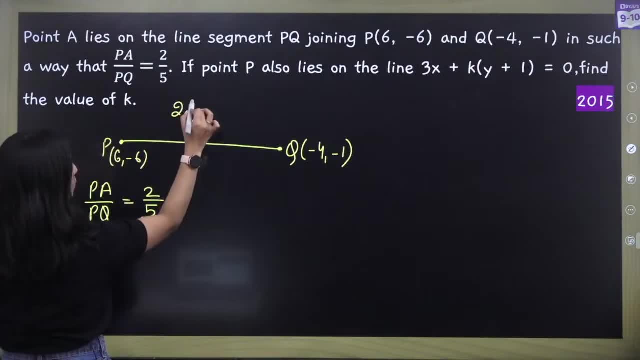 PA is 2 units. So what is this ratio? Basically, it is 2 is to 3.. Yes or no? If someone understood this much, then tell me. Total PQ has 5 parts, PA has 2 parts. 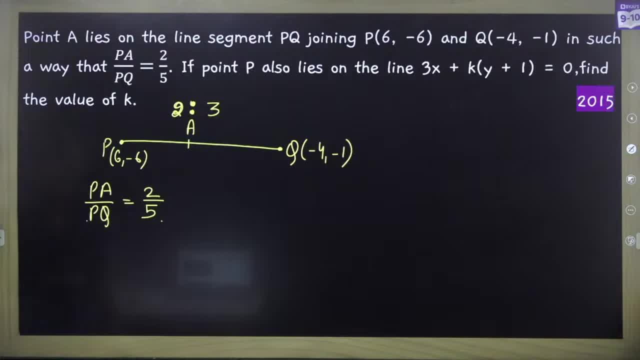 So the remaining AQ's parts will be 3 parts. If point P also lies on the line he says, which line is this point P lying on? This point P lies on this line, So we have to get the value of K. 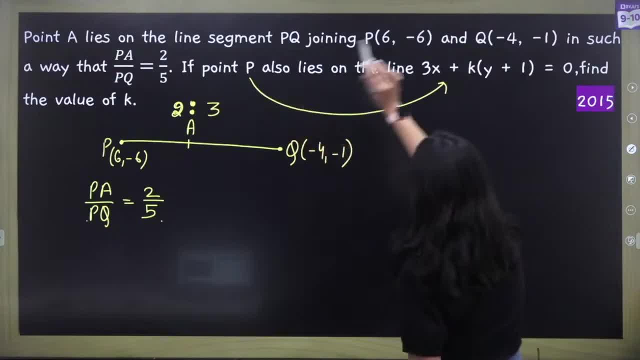 See, this will solve your whole question. If P is lying on this line, that means point P is satisfying this equation. So if point P is sitting on this line, then it is satisfying this line's equation. That means, if I put 6 in place of X, 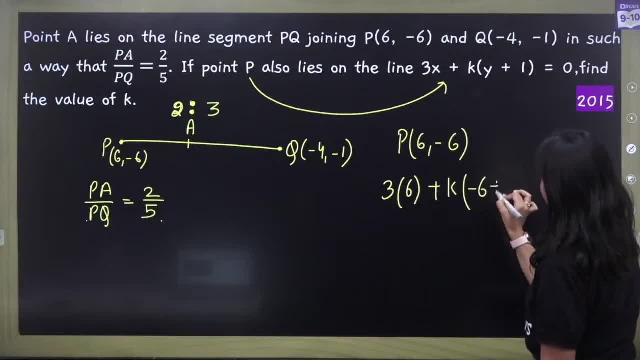 and Y in place of Y, and here I put minus 6,, then this will be satisfied. So 6, 3 is 18, minus 6K plus K equals to 0. So this is made up of 18. 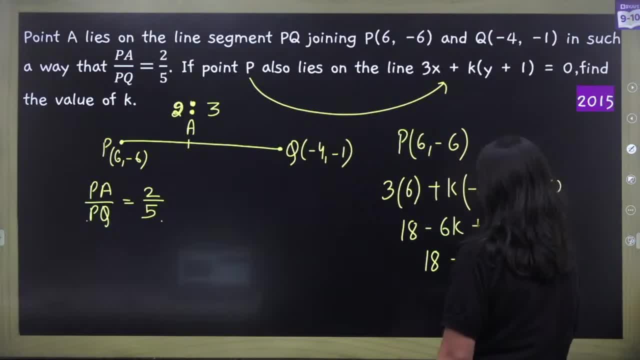 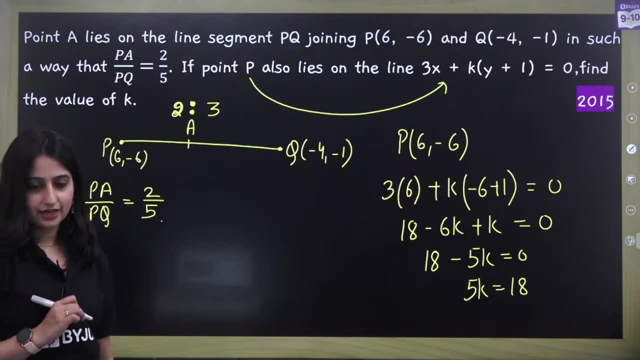 minus 5K equals to 0. So 5K equals to 18.. So how much is the value of K kids? How much is the value of K? Yes? How did 3 come? How did 3 come? 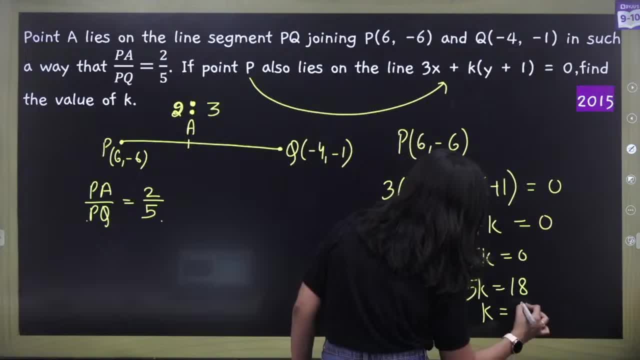 Okay, you are saying 3.6.. Yes, You got the value of K, 18 divided by 5.. 18 divided by 5 is the value of K. I have given you the story like this. It was of no use. 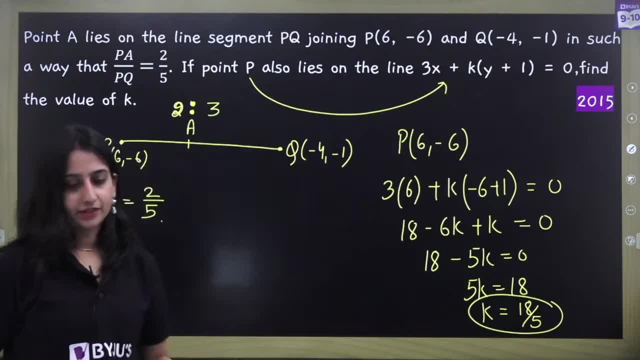 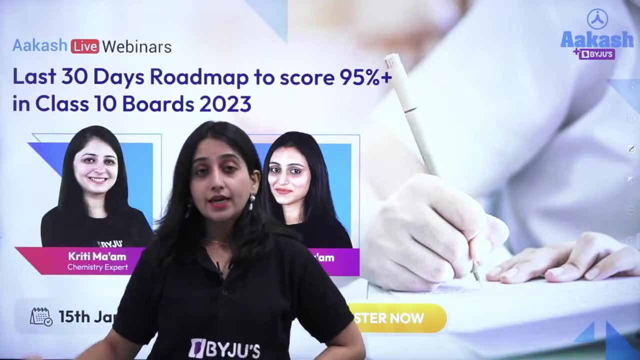 Okay, Let's move ahead. We will do all the chapters, Mehak, Don't worry. Now you know that we are bringing a very important webinar for you. Kirti ma'am and Khushboo ma'am are coming live this Sunday, on 15th, 12.30 pm. 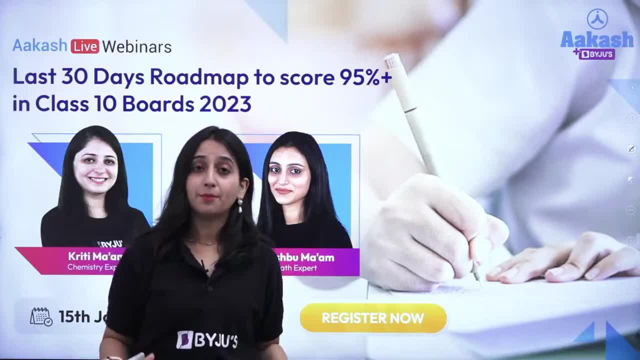 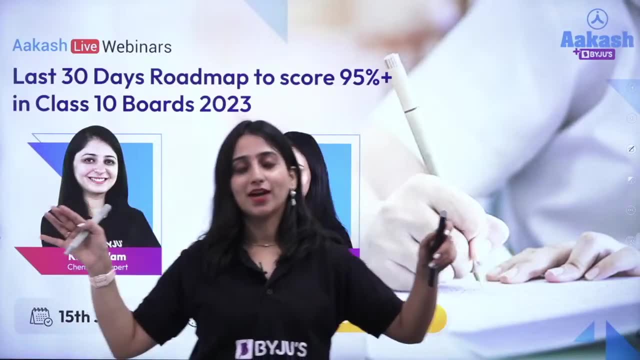 Okay, So come and watch it. We have provided you a proper road map: How to score 95 or more. What should be your strategy in the last few days? Okay, So do not forget to register. This is a free webinar. 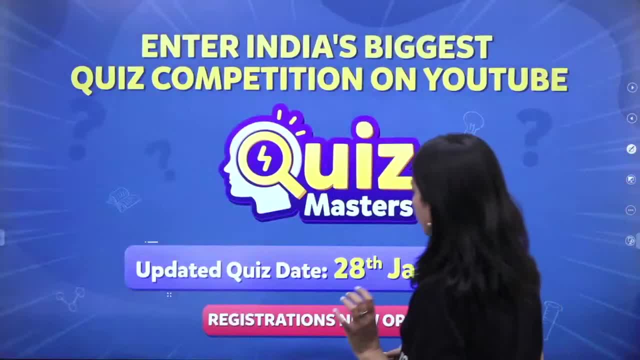 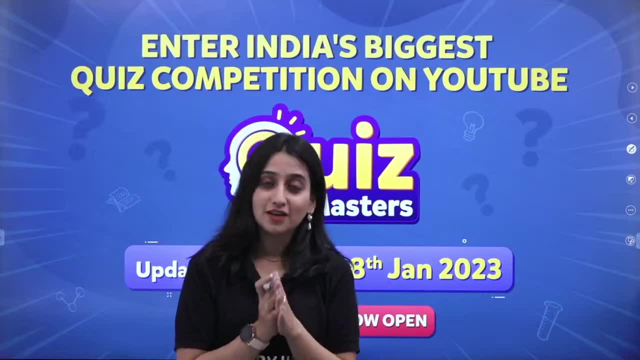 Everybody can come and watch. You will get the link in the description box. And another grand thing that is happening this month is Baiju's Quizmaster. So if you haven't registered for the Quizmasters yet, then make sure you register. 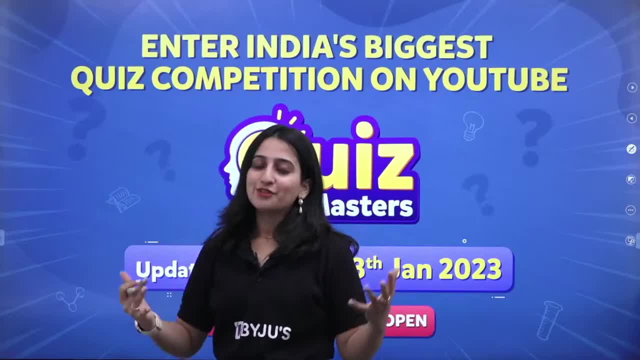 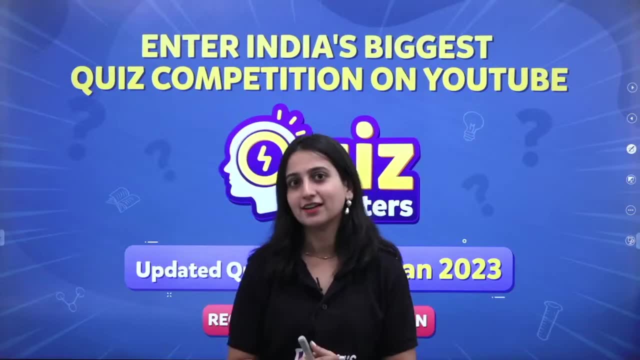 Because a lot of entries have already come. Kids are very excited Because obviously they are very excited to come here in the studio, meet their teacher, participate in the live quiz, gain the full experience. It's a wonderful thing, Right. 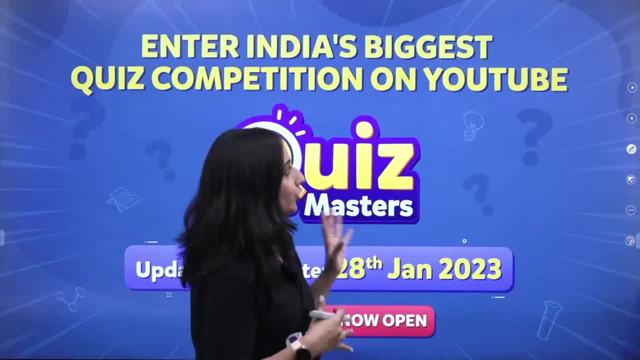 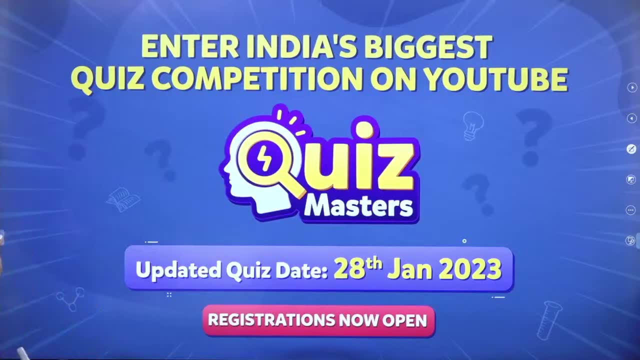 So this chance is missed by everyone. So if you also want to experience all these things, then make sure you register. Link is in the description box. It's free kids. You don't have to do anything, You just have to register. 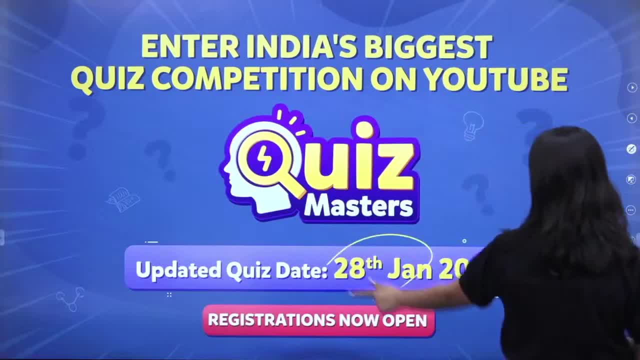 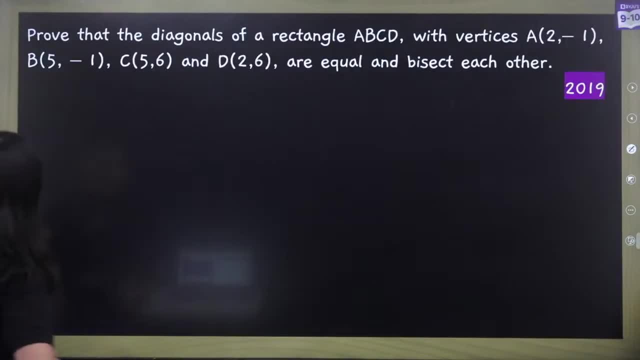 Okay, And it's possible that you are a lucky kid and you get selected. It's happening on 28th January, Baiju's Quizmaster. Come on, Let's see the next question. Prove that the diagonals of a rectangle ABCD. 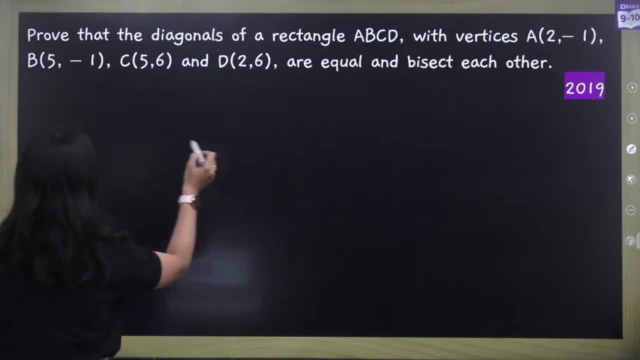 with the vertices ABCD. this are equal and vice that teach other. So how will you prove this? Someone will tell me, Ma'am. how will you prove this? So you have a rectangle: A, B, C and D. Always keep in mind. 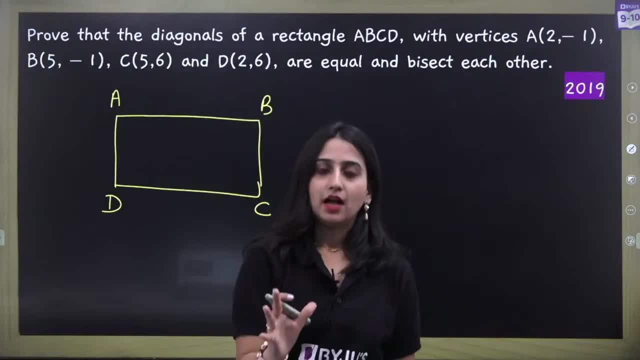 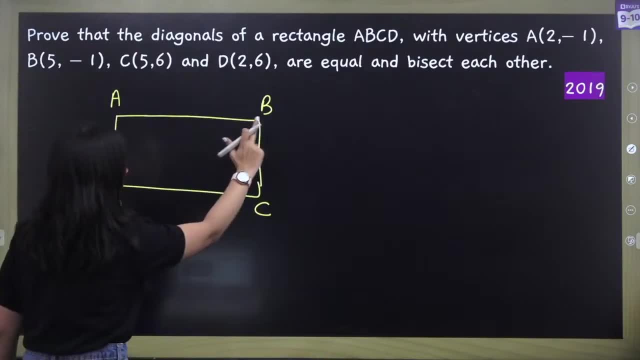 when you are naming a quadrilateral, when you are naming, it should always be in a cyclic manner. If you do ABCD, the whole question will be wrong. Okay, Order matters a lot, So keep in mind. Okay, So how much is A? 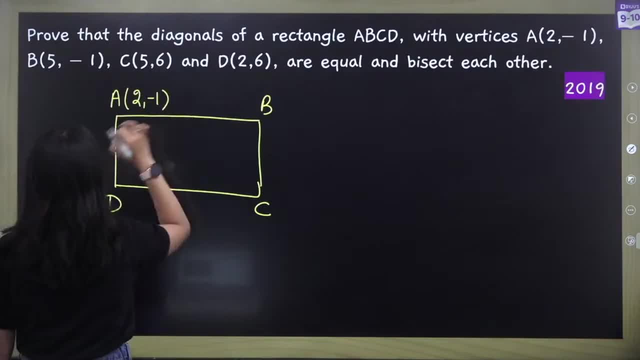 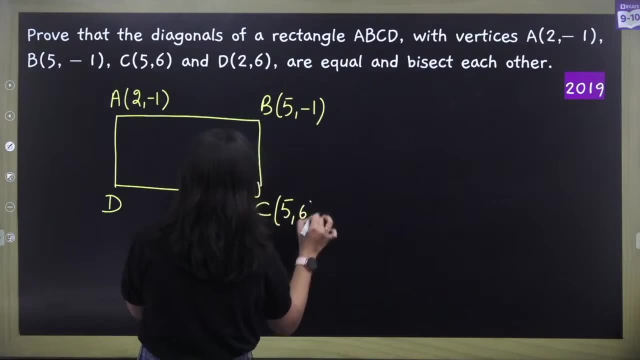 A is given, A's coordinates are 2, minus 1.. B's coordinates are 5, minus 1.. I think you can do this question. I will just explain the concept to you. How to do it. Rest, it's a kid's game. 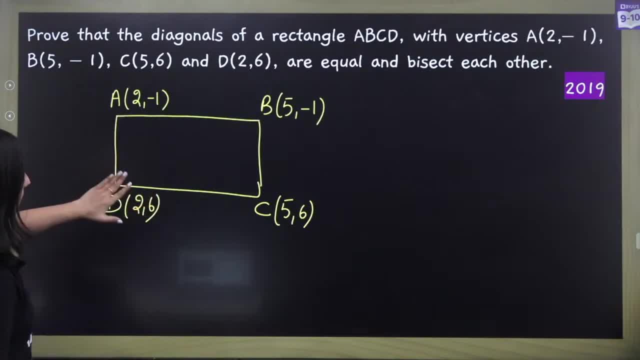 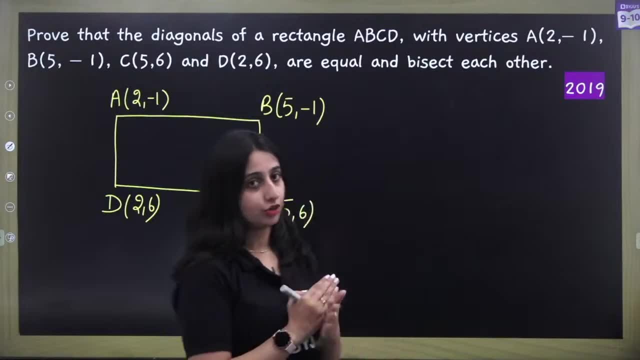 Okay, So learn the main thing: If you have a rectangle, if you want to prove its quadrilateral as a rectangle, then there are two things: The diagonals of the rectangle are equal and they are bisect, And we have to prove this here also. 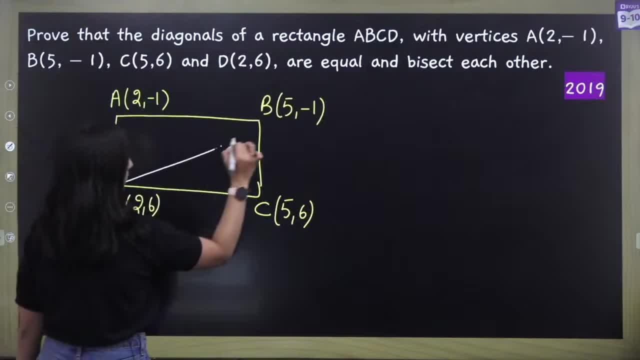 First of all, let's make the diagonals. Come on, I have made this diagonal, I have made these two diagonals. Now, if these two diagonals are equal or not, then how will we know? We will apply the distance formula. 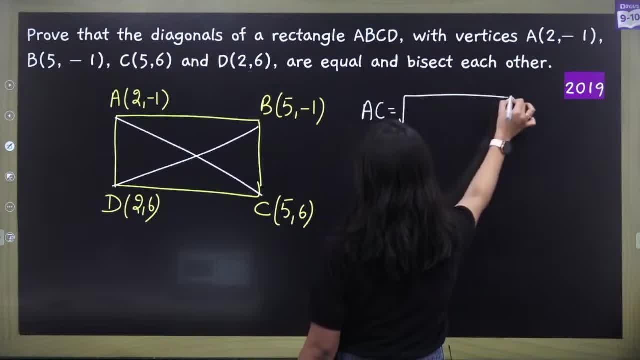 So take out AC distance, Apply the distance formula, So I will do one X2 minus X1, square Minus both X. So it is easy to do 5 minus 2.. So 5 minus 2 is 3.. 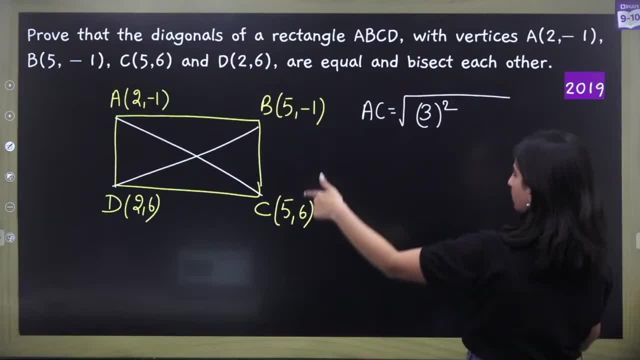 And 6 minus 1.. That is 6 minus of minus 1.. 6 plus 1 is 7.. So what is this? Someone will tell me: 9 plus 49.. So how much did you get? 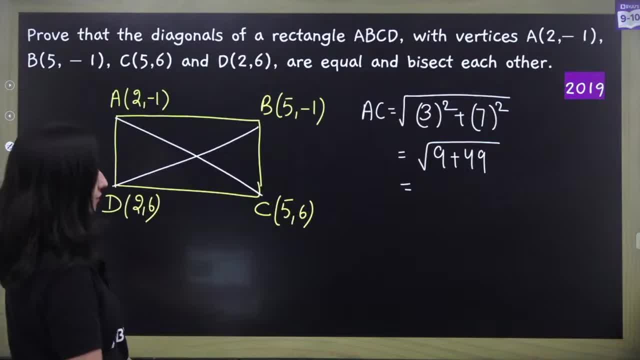 Tell me From the midpoint formula. Yes, I will tell you that too. So take out AC. Similarly, take out BD. here You have to apply the distance formula on BD too, And the value of BD will come If these two values come the same. 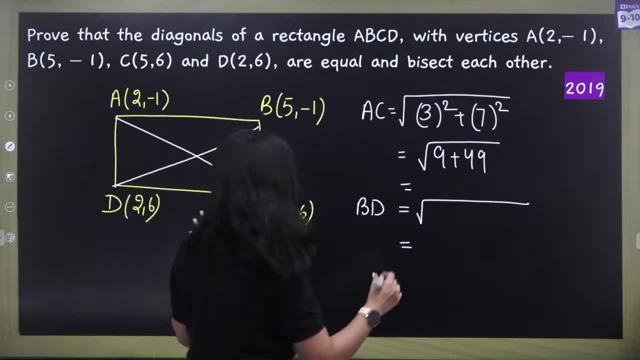 then that means the diagonals are equal. So the root of 58 has come Very good. Yes, it is absolutely correct. The diagonals will be equal if the length of BD also comes to root 58. Now how will we understand how to bisect each other? 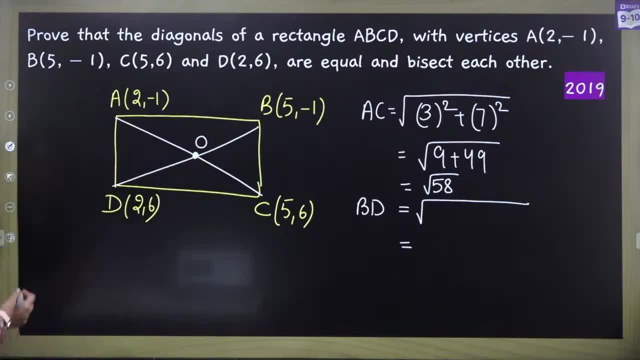 These two diagonals are on point O, So let's assume that the coordinates of point O are. So look, we know that this O is the midpoint of AC and this is the midpoint of BD, Because the diagonals of rectangle bisect. 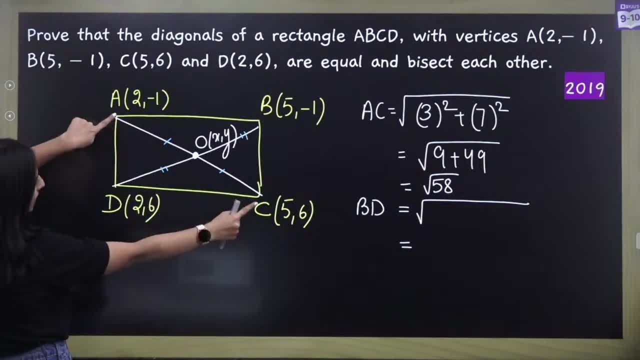 But we have to prove this. Okay, If you treat this as a line segment, then since this is equal to this, then O is the midpoint, So we take out the midpoint. Okay, Take out the midpoint. So here we will take out the midpoint of AC. 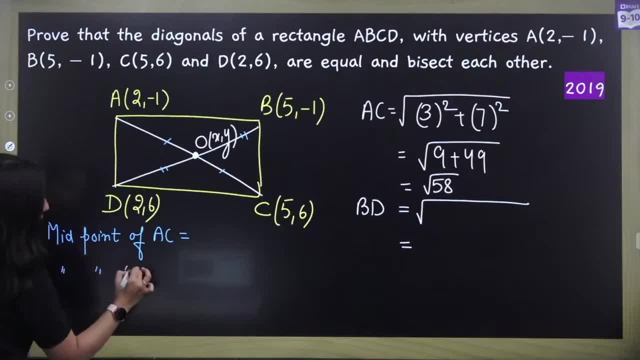 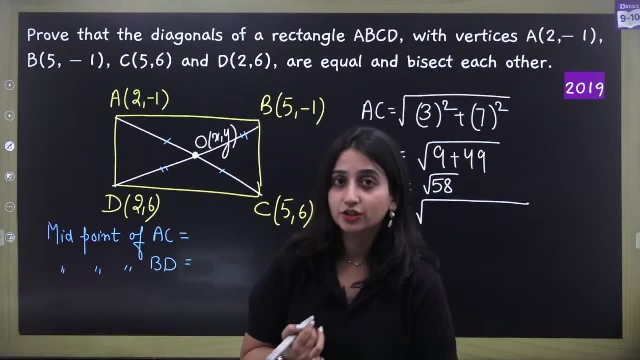 Take out the midpoint of AC. Similarly, take out the midpoint of BD. So this should also come to be the same. If this comes to be the same, then that means the diagonals are also bisecting each other. The diagonals are also equal in length. 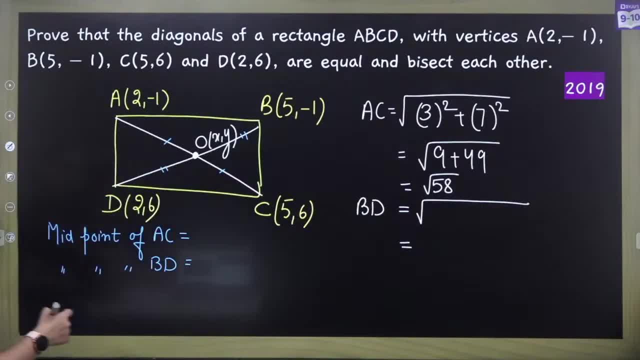 So it is proved. Okay, Yes, How will you draw the midpoint? What is the midpoint formula? x1 plus x2 divided by 2.. That is 5 plus 2.. 5 plus 2 divided by 2.. 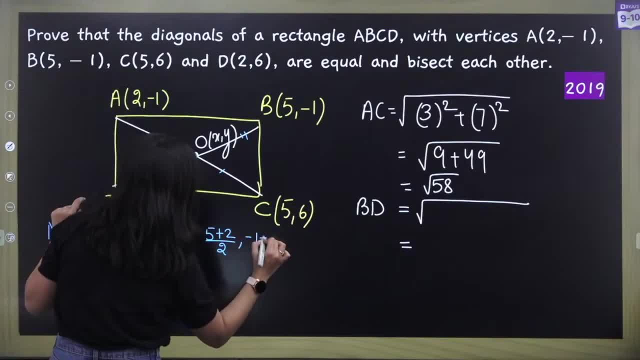 And minus 1 plus 6.. Minus 1 plus 6 divided by 2.. So what is this? So this becomes 7 divided by 2.. X will come and y coordinate will come. your 5 by 2.. 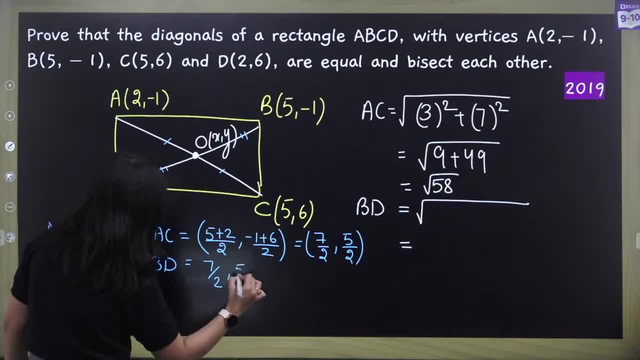 Similarly, if you take out the midpoint of BD, it will also come 7 by 2.. Similarly, if you take out the midpoint of BD, it will also come 7 by 2.. that will also come 7 by 2 and 5 by 2.. 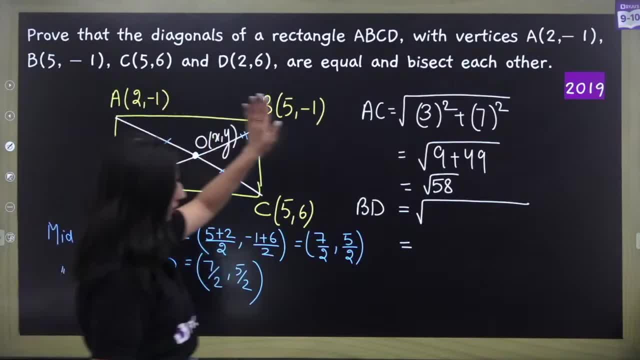 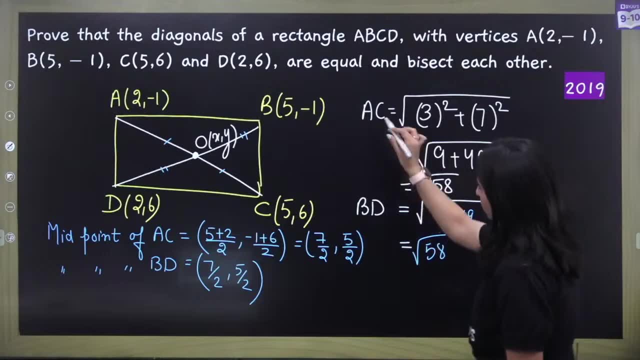 Because both have midpoint same. so both of these are bisecting. And if you do this carefully, then this will also come 9 plus 49, this will also come 58. So diagonals are equal in length. also they are bisecting each other. 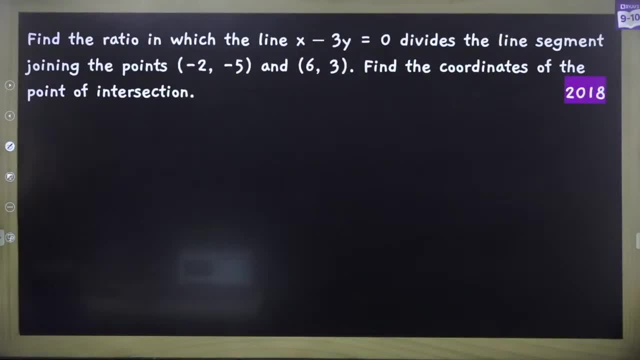 Okay, Alright. Next question. The question says: find the ratio in which the line divides the line segment joining the points this and this. Find the coordinates of the point of intersection. So what all do you have to find in this question? 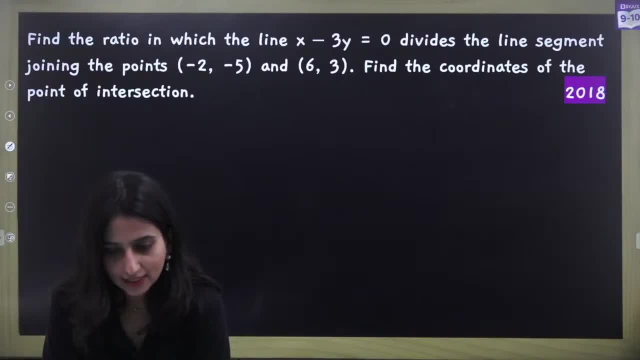 What all do you have to find in this question? Yes, Bharani, diagonals are equal. Yes, Yashvi, please, it's a humble request- rewind a little bit and re-watch it again. Okay, You will understand it. 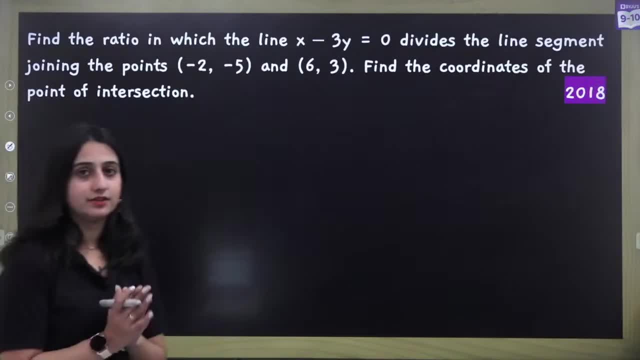 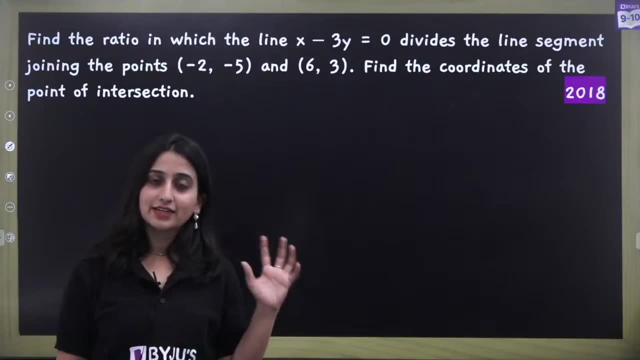 Okay So we have this time crunch. I have to finish all the 10 questions in one hour only. Okay So, so that there is no time waste for any of the children. So that's why we are providing the content in this way. 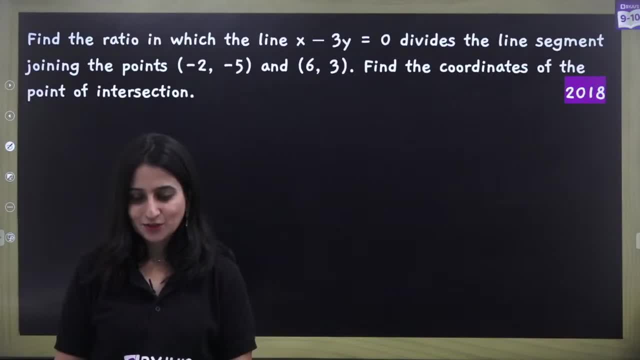 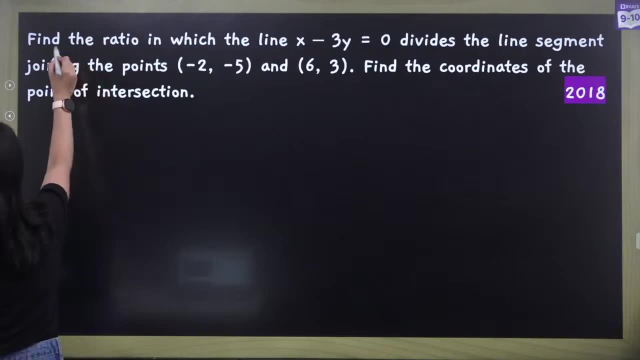 So now, if you re-watch it a little bit, you will understand. I promise you that. Okay, Let's go. Next question. let's see: find the ratio. We have to find the ratio, alright, In which the line this: 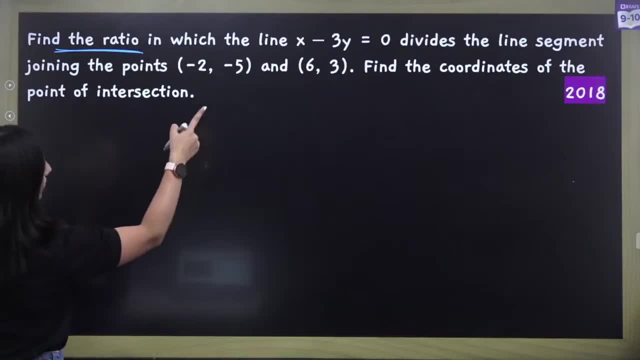 this is the line. okay, Joining the mid point divides the line segment. Okay, I have a line segment. Let me draw a line segment for you. First, let's make a line segment. Okay, First of all, do this work? 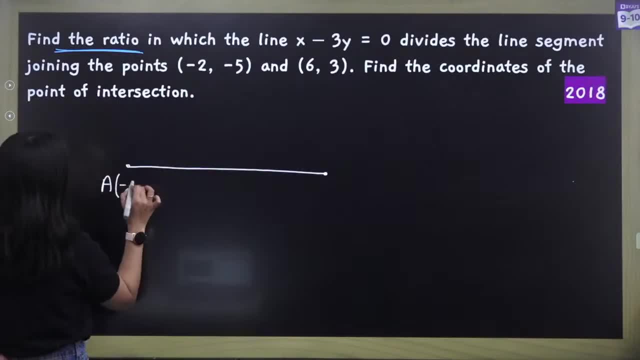 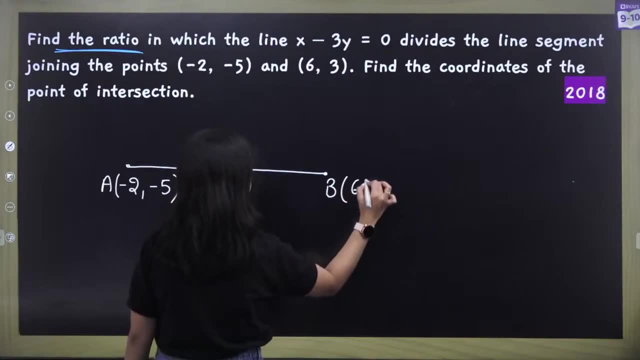 Which points do you have to join to make a line segment? I will give the name of the points: Minus 2 comma. minus 5.. Understand this question carefully And I will call it B, point 6, comma 3.. Okay, 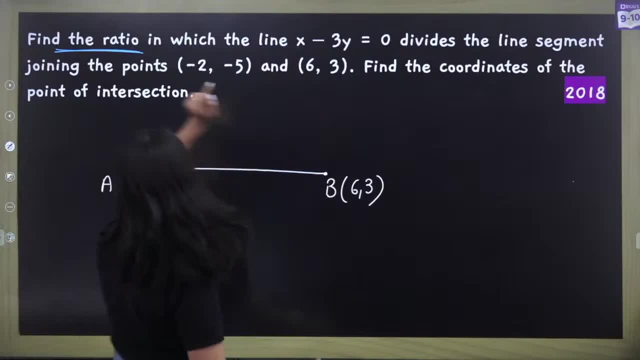 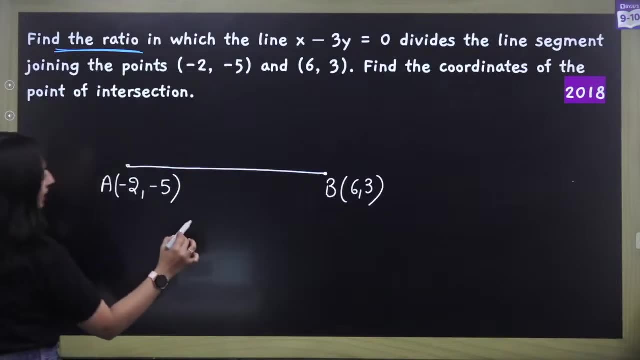 So, first of all, I have made a line segment because it has said line segment joining the points this and this. Now what is happening? This line segment is being divided by a line. So now I will make a line. 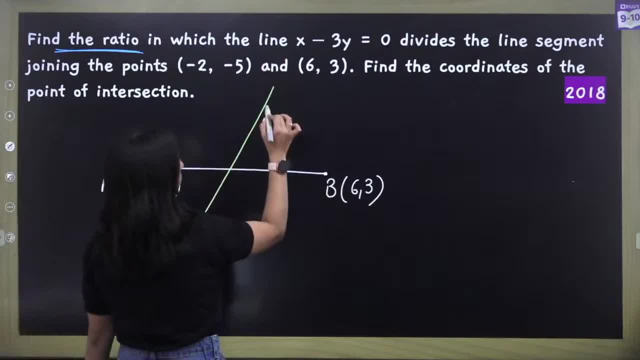 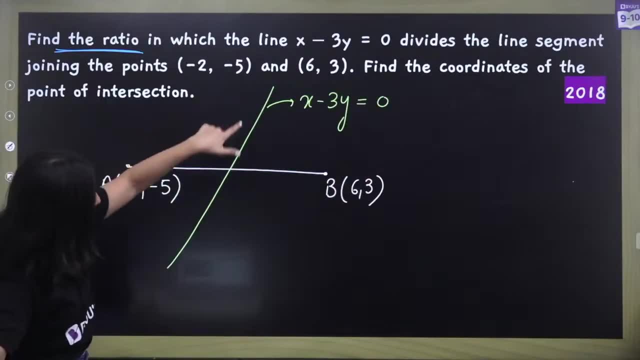 So I have made a line. let's assume The equation of this line is given to us: how much X minus 3Y equals to 0.. Okay, He is saying that this line segment, this line divide, this line segment AB. 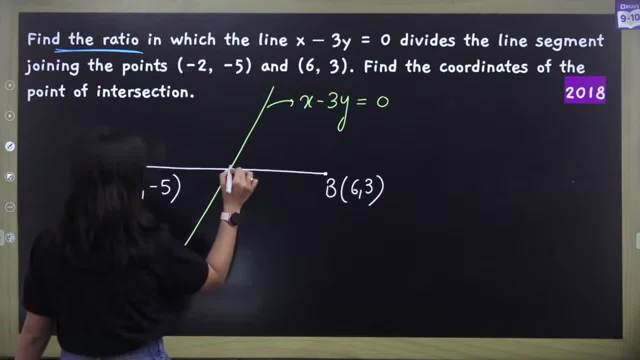 in some ratio. I don't know what that ratio is, So let's assume what is that ratio. son, Let's assume what is that ratio. Very important question K is to 1. Because I don't know the ratio. 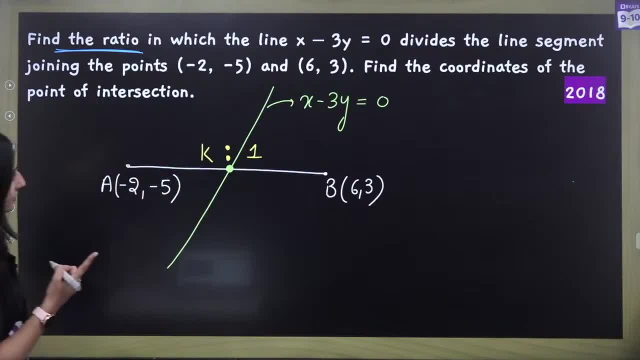 so I have given the ratio, as the sum K is to 1.. Okay, what else? Find the coordinates of the point of intersection. You have to find the coordinates of this point. Let me call it point P. So we have to find the coordinates of this point. 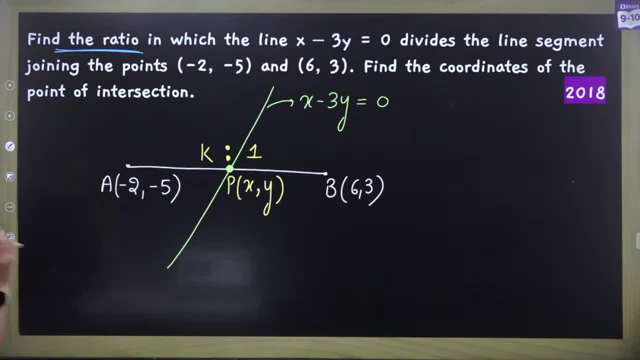 Okay, So you have to find the value of X and Y. Okay, tell me one thing: If a point is lying on the line, what does it mean? Can anyone tell me? I had told you at the back. If a point lies on a line. 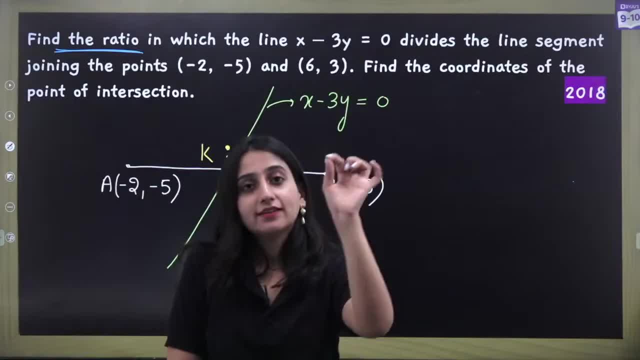 it means that it is satisfying the equation on which it is lying. Equation on the line on which it is lying. Did you understand? So if point P, if it is lying on the line, on the line, then it means that 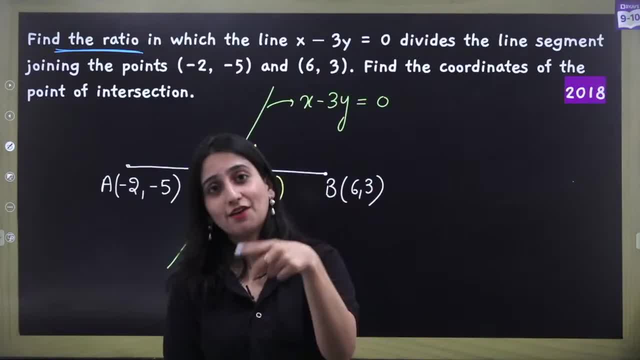 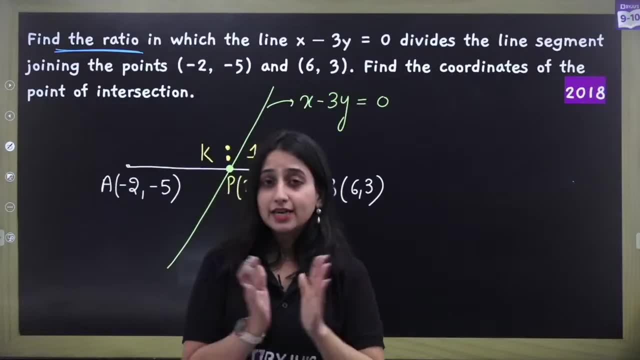 the coordinates of the point P means the values of X and Y. if I put those values in the equation, in the equation of that line, then they will satisfy it. This is what it means. This means that point P is the solution of this equation, of this line. 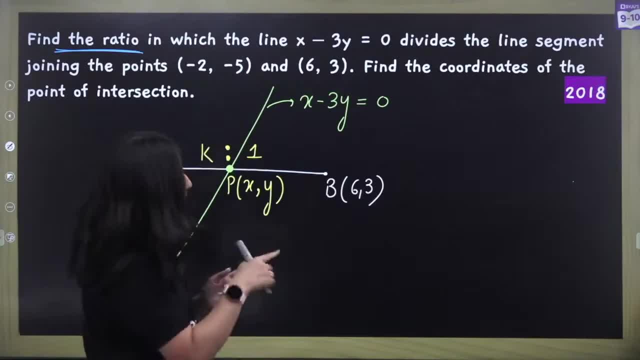 This is what we also knew in linear equations, Right? So it satisfies the equation So much that I got to know that this P point will satisfy this line Very good. First of all, let's remove these coordinates With the help of the section formula. 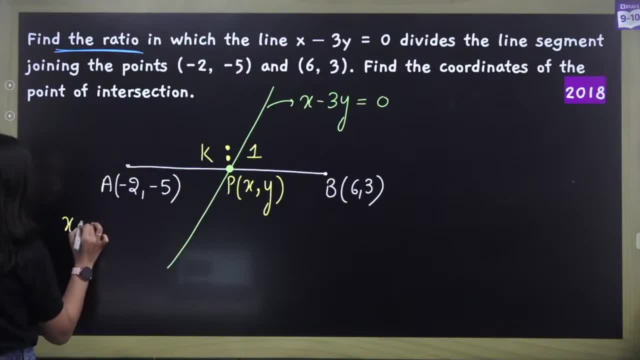 Can you help me with this? Let's go. What will be the value of X? Someone will tell me X will be K into 6.. K into 6 plus 1, into minus 2 divided by K plus 1.. So the value of X is 6K minus 2 divided by K plus 1.. 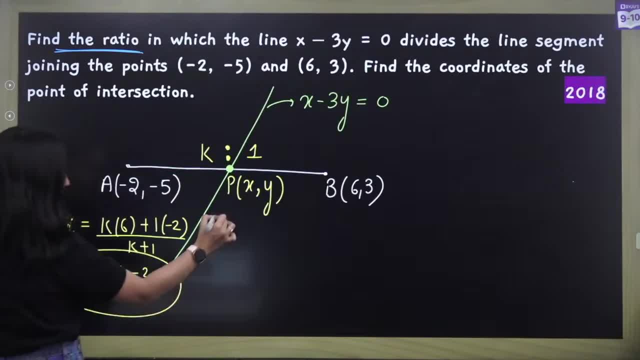 This is the value of X. Similarly, someone will tell me the value of Y. What will be the value of Y? Let's apply the section formula K into 3.. So 3K 1 into minus 5.. 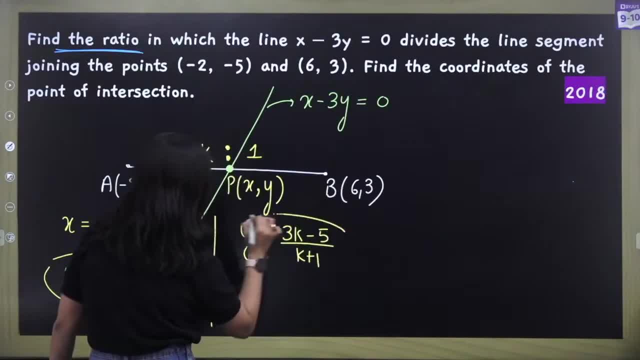 Minus 5.. Minus, 5. Divide by K plus 1.. So this is the value of my Y. So what does this mean? What is the point P that I have? This means, therefore, I can say that 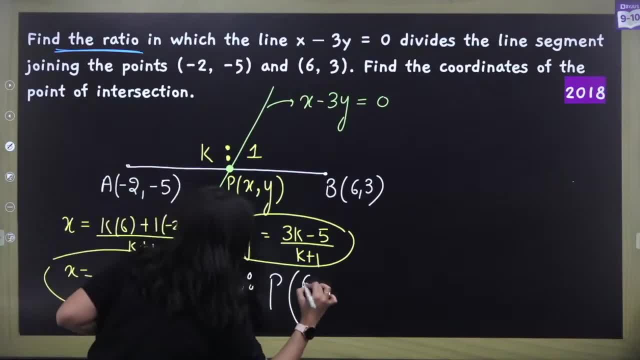 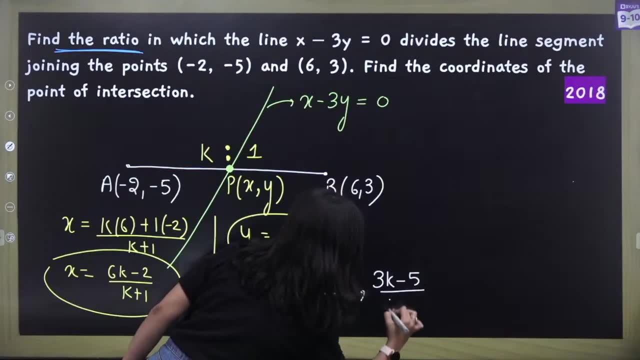 in front of the coordinates of point P, I have 6K minus 2 upon K plus 1 comma, 3K minus 5 upon K plus 1.. This is a super important type of question. Keep this in mind. This is a very important question. 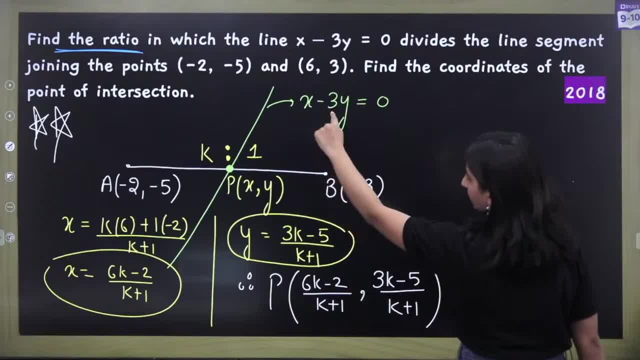 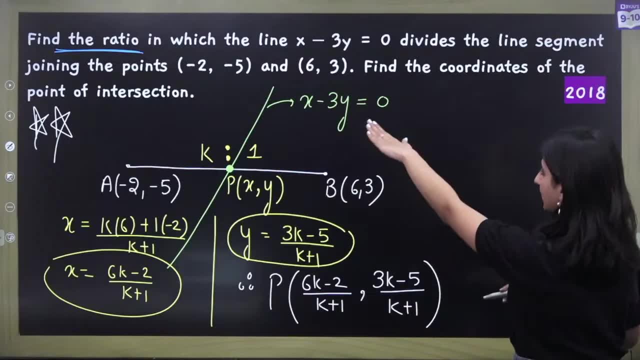 Now what did I say? Since P is minus 5 divided by K plus 1. The P lies on this line, So that means P will satisfy this equation. So if I put the coordinates of this P here, then we will satisfy. 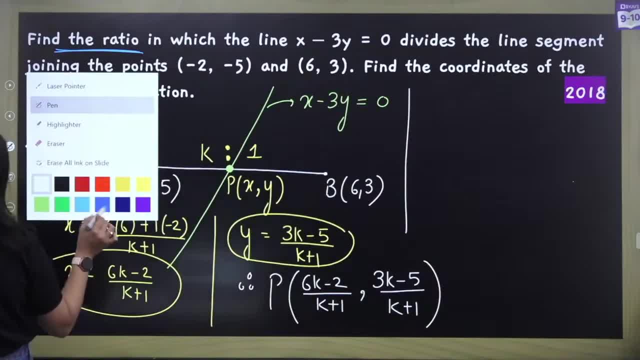 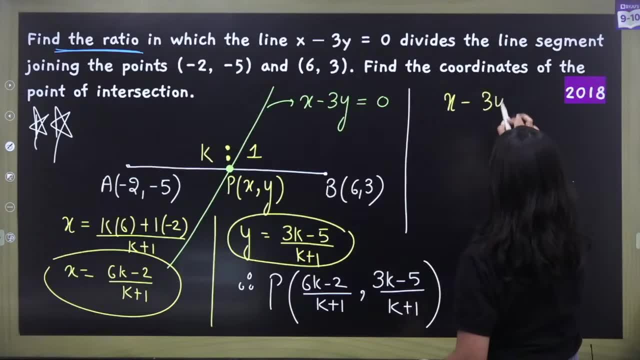 So now we are going to do the same Here. we are going to put the coordinates of this P point there. Come on. Instead of X, let's substitute. I have an equation: X minus 3Y equals to 0. 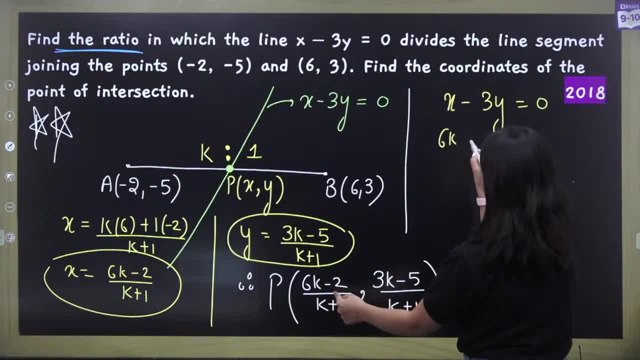 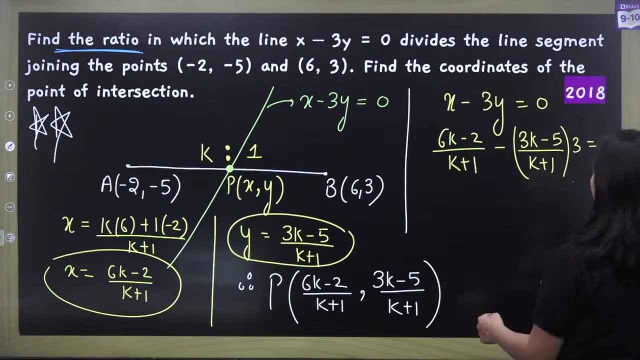 So instead of X I will put 6K minus 2 upon K plus 1.. minus here, 3k minus 5 upon k plus 1. multiply by 3b equals to 0.. Okay, I did the same thing, I just put values. 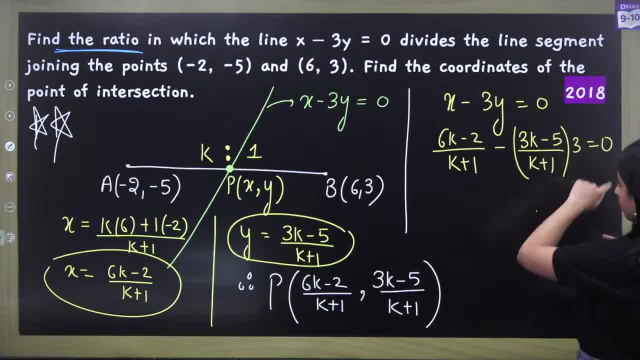 Okay. so if we see here, k plus 1 will be multiplied by 0 there. So what will be above? 6k minus 2, this becomes minus 3, 3 is a 9. k plus 5, 3 is a 15.. 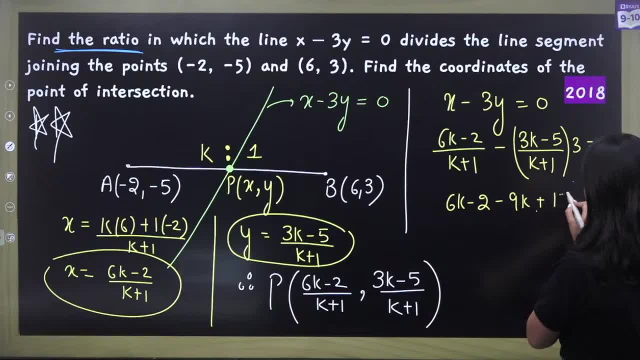 So 3: 3 is a 9, minus will come 5, 3 is a 15 will come, equals to 0.. Okay, so just solve this. what will be done quickly? someone will tell me This becomes 13 minus 3k. this is done. 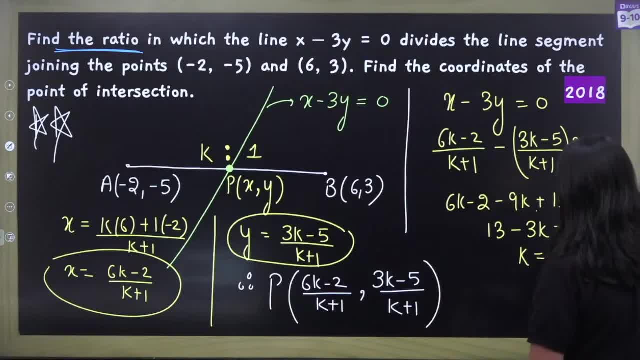 So how much value of k we got. We got k value 13 divided by 3.. Is it like this, yes or no? 13 divided by 3 is the value of k everyone. Is it like this, yes, clear. 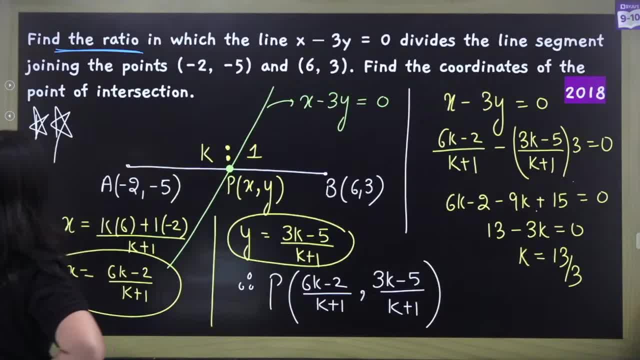 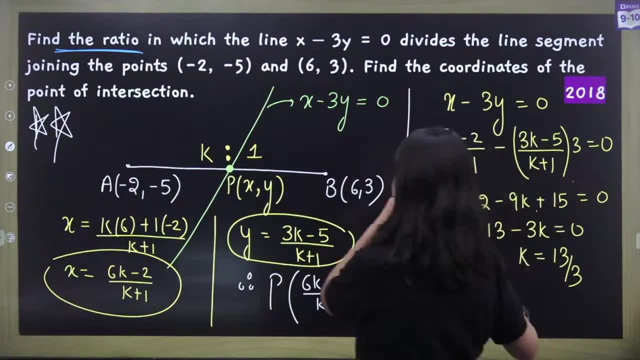 Okay, so you have got k value. what else do we need to find? Find the coordinates of point of intersection. We have taken it out, right, So sorry. k ratio has come. sorry, you have to put k value in this and take out the coordinates. 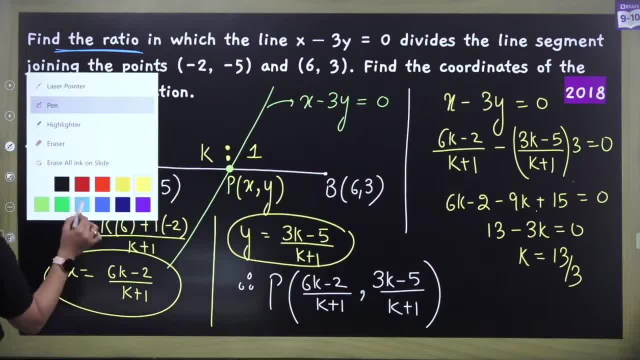 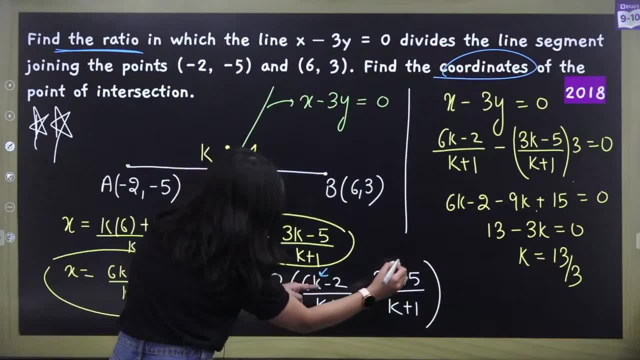 I think you will do that. Okay, we have taken out the ratio. after that final answer, you have to take out the coordinates. How to take out the coordinates? You will take out the coordinates by putting the value of k here. you have to put the value of k here. 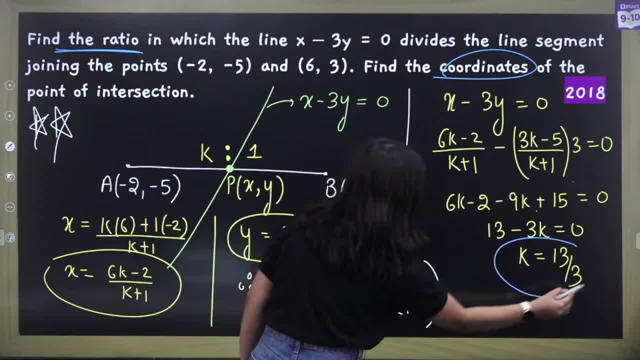 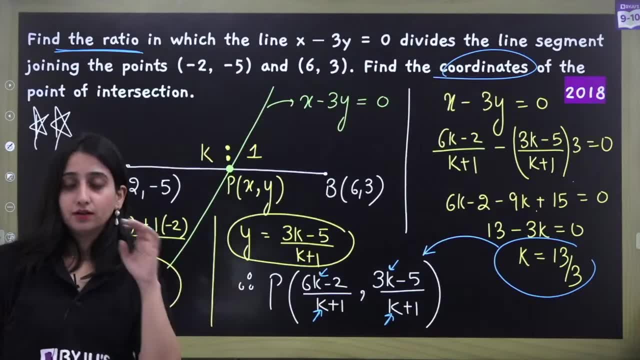 Okay, so you have taken out the value of k by 13, by 3, now you have to put it here by taking out the final coordinates. you have to tell me in the comment section what is coming. Okay, so this becomes a question of your weightage. 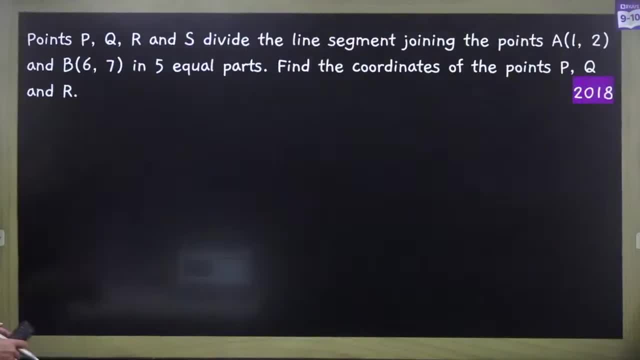 Okay, all the best, Yashvi. Next question. Next question: Point PQRS divide the line segment joining the points A and B in 5. Five equal parts find the coordinates of the point PQR. Now here, as we did, the question of the trisection, now such questions are also asked that: divided in 5 parts, divided in 4 parts, divided in 6 parts, how many parts can it divide the line segment? 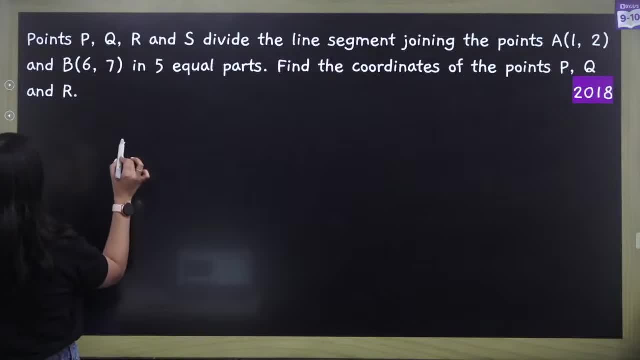 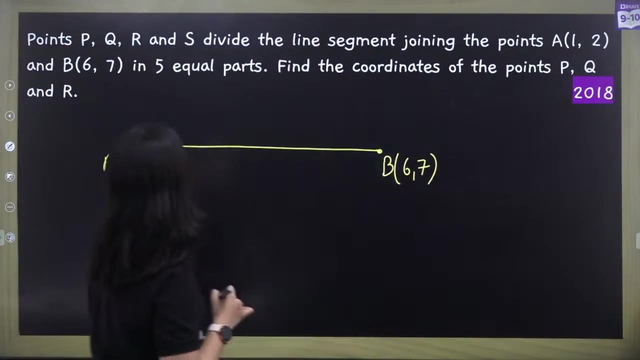 Okay, so here in this question, what we are doing, we have a main line, segment AB. what are the coordinates of A? 1 comma 2, the coordinates of B are 6 comma 7.. Okay, 6 comma 7, how many parts have we divided it? 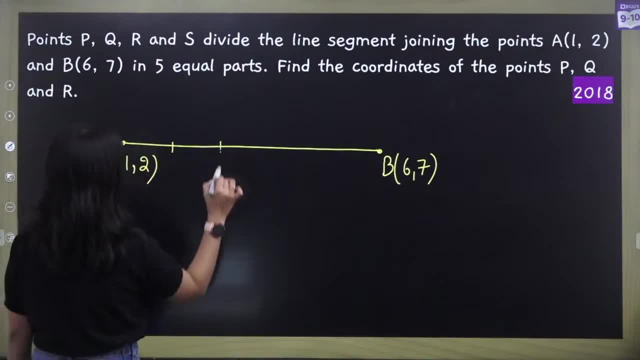 PQRS 5 parts: P, Q, R and S. See which coordinate will I take out first. See this carefully and give me the answer. See this carefully and give me the answer. We have one thing I am understanding, because these are all equal parts. so P is the midpoint of AQ. 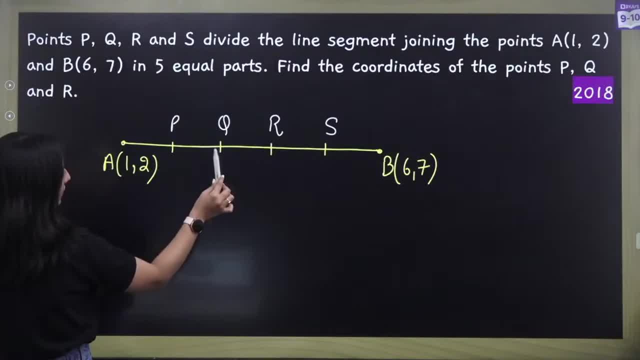 Q is the midpoint of PR. Q is the midpoint of PR. Q is also the midpoint of A or S. Q is also the midpoint of A or S. Are you understanding my point? I know how to solve it. Solve it very good and, happily, very quickly. 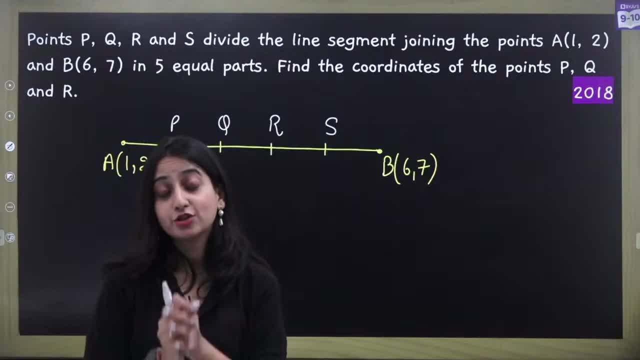 All the best to all of you who have Prevots tomorrow, and all the very best to all of you Now, all the students who have Prevots this week. all the best, Okay, come after doing good papers. Now let's remove the P. first. let's find the coordinates of P. 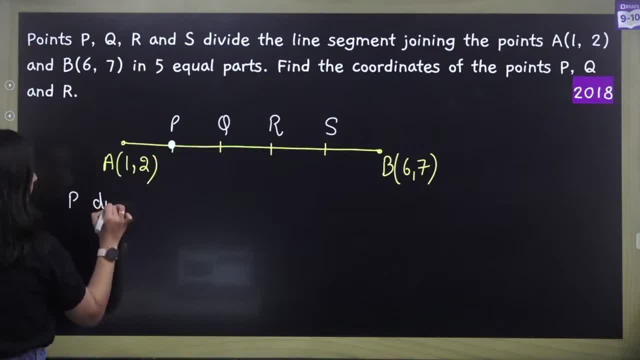 to find the coordinates of p. so p divides, p divides a, b. in what ratio p divides a, b in 1 is to 1, 2, 3, 4 in 1 is to 4 ratio. so section formula laga: do fatta fatta se to p ke coordinates. 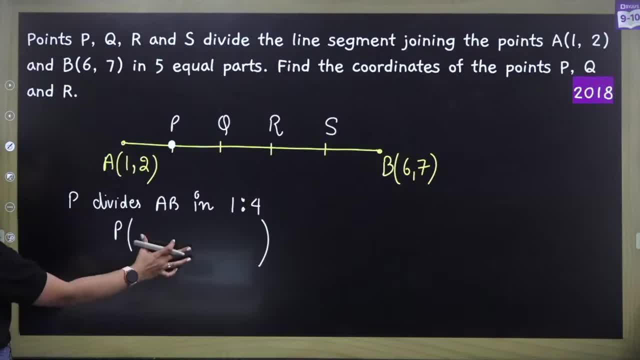 kya a jayenge p ke coordinates ma directly section formula laga rahi hoon to ye a jayenge aapke ye 1 is to 4 ka ratio mein divide ho raha hai p to ye a jayega, 6 plus 4, 6 plus. 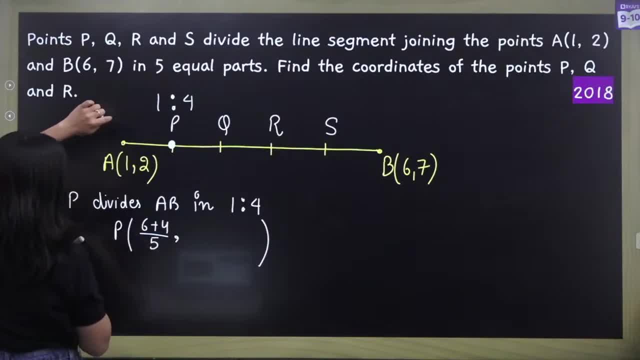 4. divide by 5 comma, yaha pe kya a jayega fir 7 plus 8. divide by 5 to p ke coordinates, kya ban gaye 10. divide by 5: this is 2 to ye 15. divide by 5, this is 3 to p ke coordinates. 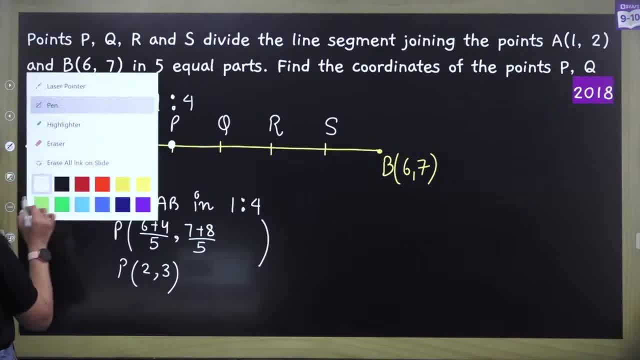 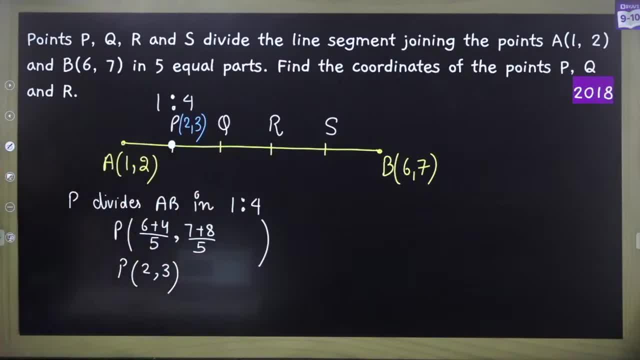 clear. yes, sab ke aage. 2 comma 3. is it clear? chal, 2 comma 3 aage right, bahut badhia. ok, abhi me kya karti ho abhi r ke coordinates: nikal le or s ke nikal le patao r k nikal le r ke. 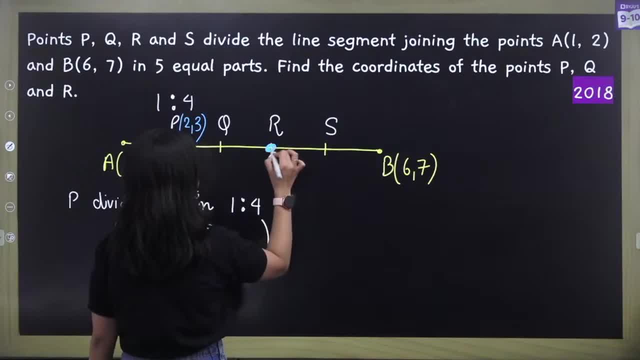 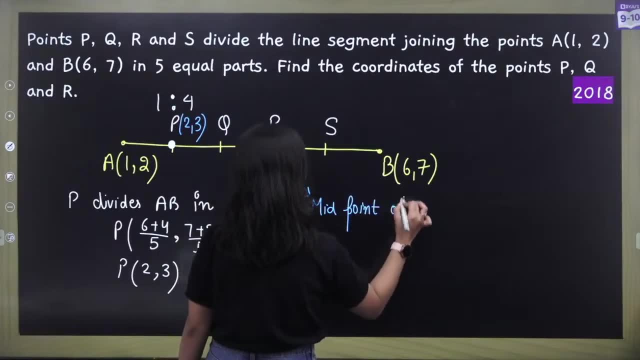 coordinates: nikal le kitne easy araam se nikal sakte ho kaisi ye r kis ka mid pointhe hai. r is basically mid point of ye kis ka mid point ban gaya. p b ka mid point ban gaya. yes. 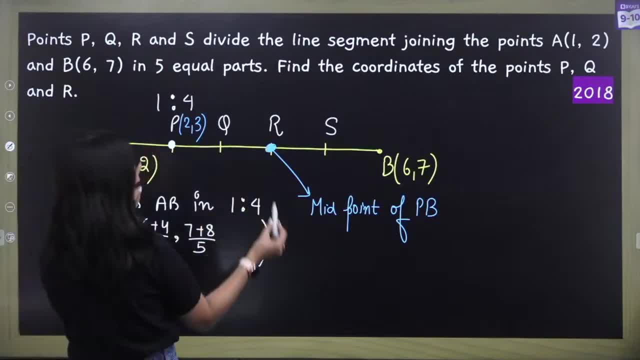 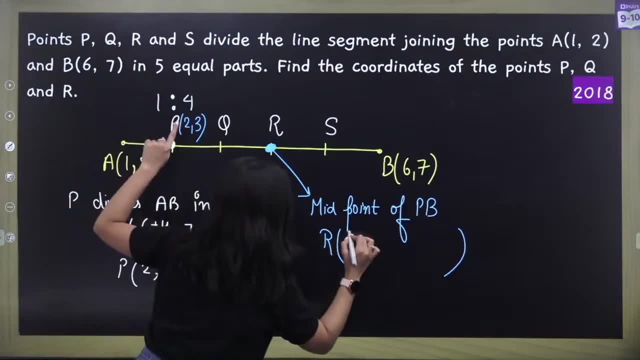 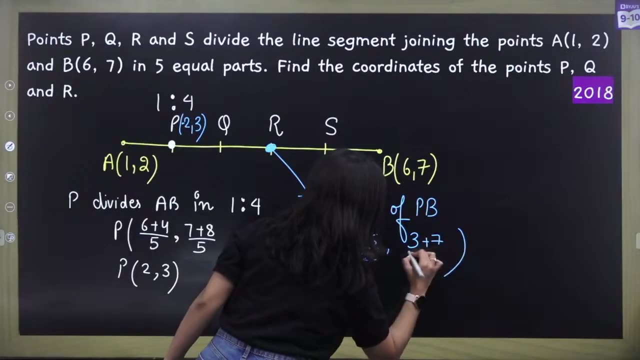 pb ka midpoint ban gaya hai. na so r k coordinates, kitne asani. se aajayenge to r k coordinates, hamare pass kya aajayenge. 2 plus 6 divide by 2 comma. 3 plus 7 divide by 2, so ye r k. 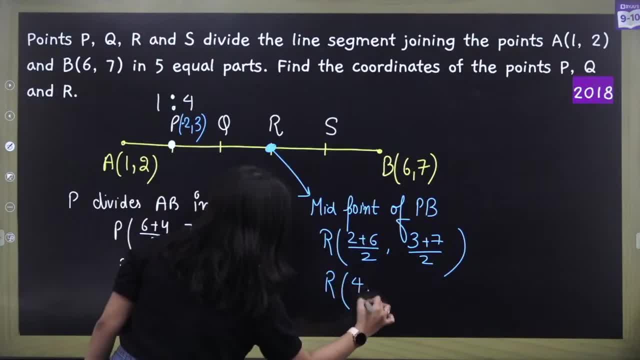 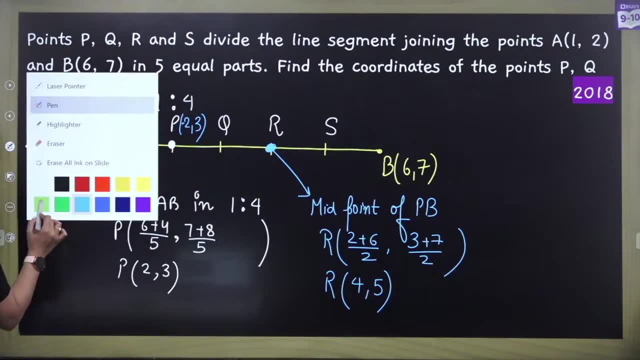 coordinates aajuk hai hamare pass: 8. divide by 2, that is 4, 10. divide by 2, that is 5. to 4 comma 5. I think ab baaki to aap easily nikal logay ab ye coordinates aajuk hai aap. 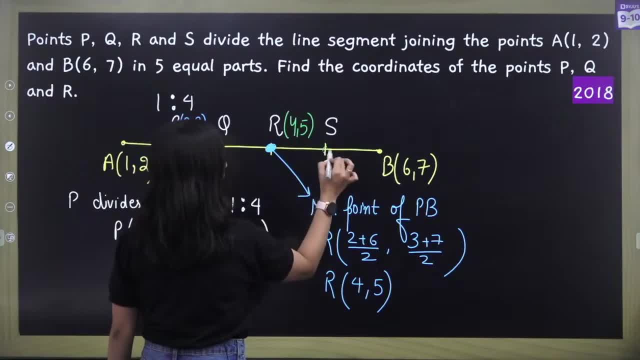 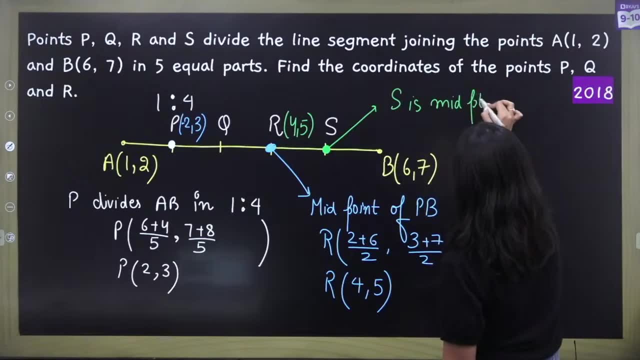 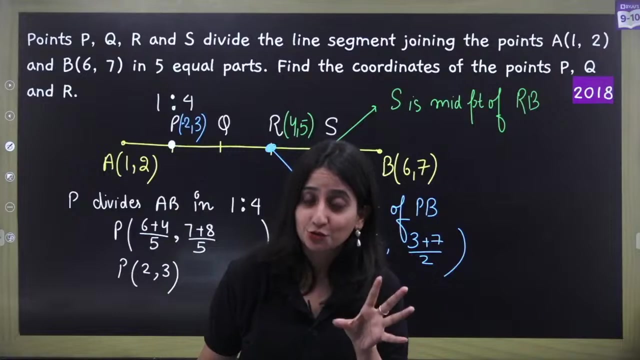 ke pass r k 4 comma 5 ab. ye jo s hai s kis ka midpoint hai? s is the midpoint of r b ispe laga lo. similarly, q is the midpoint of pr. I think baaki saare jo coordinates hai wo aapke midpoint formula se. hi nikal jayenge baar baar section formula lagane ki zuruvat. 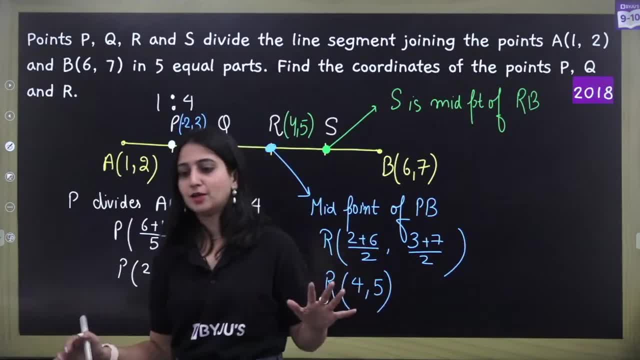 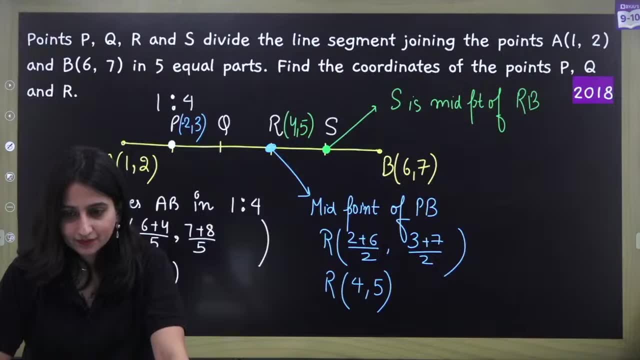 ni padhi section formula ek baar laga diye. baaki saare time hamne midpoint formulas laga diye. is it clear? yes, bacha, sabko samajh me aagea, sabko samajh me aagea ma'am, how one is to four dhanya kitne parts me divide kare hain. 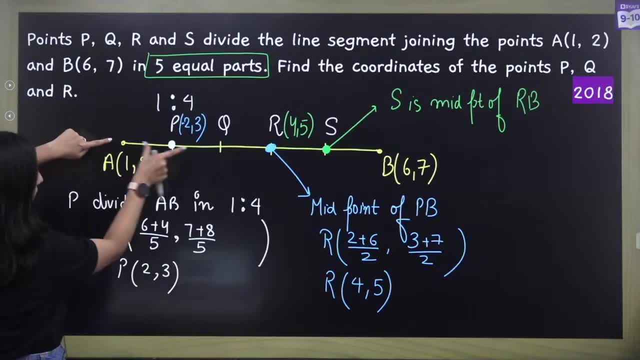 line segment ko 5 equal parts me. so these are 1, 2, 3, 4, 5 parts to agar p ki baat karun. ya ha per agar p ki baat karun, dhyan se dekho to p ke left side me, kitne parts hai to aap. 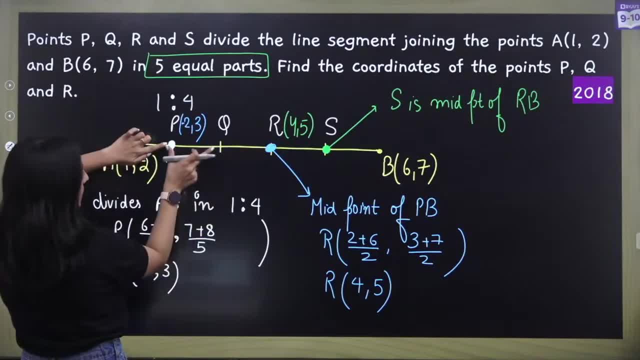 parts. only one part is there and right side me kitne parts hai: 1,, 2,, 3, 4. isi liye 1 is to 4 ka ratio. me divide ho raha. hai clear? maine ask. nikalna bata diya agar aap se question. 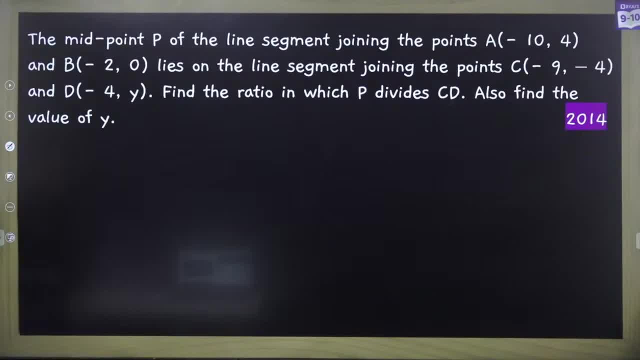 me pooch liya jaye takki aap nikal pao chalo. next question: dekho zara. question says the mid point of P. the question says the mid point of P of the line segment joining the points A and B. 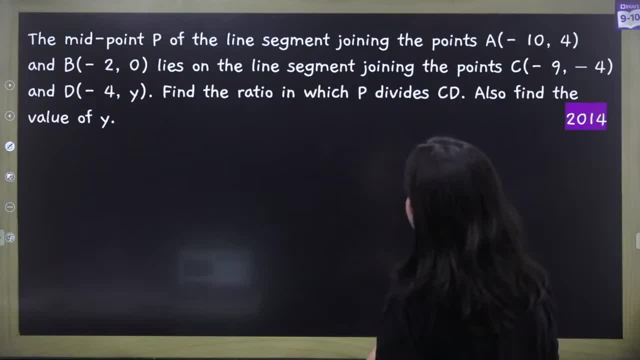 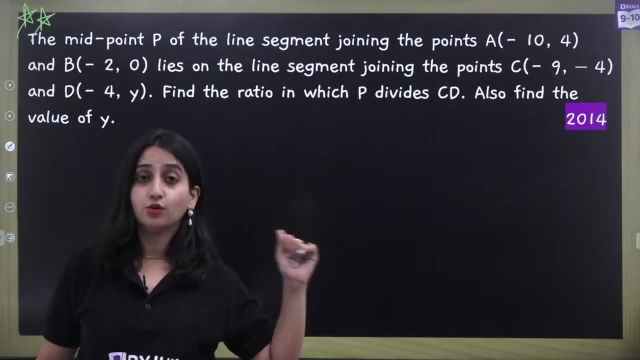 lies on the line segment joining the points C and D. very interesting and important question. star mark karo isko chalo. very important and interesting question. koi bacha try karna chahta hai. those who want to try this question out on yourself ek kaam karo. 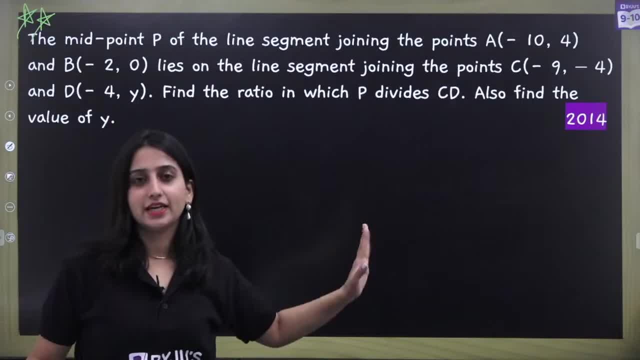 pause karlo zara screen ko. pause the screen. pause the video. try it on your own right and uske baad play karke dekhna ki kya sahi kiya hai. nahi kiya jo mere saath karna. 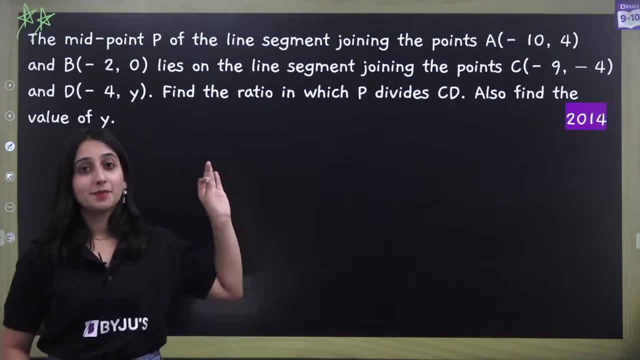 chahte ho, mere saath bhi kar sakte ho, but still, main chahti ho ki aap ek baad try karo aur dekho, ki aap ye question ka solution nikal paare ho, ki nahi tike? 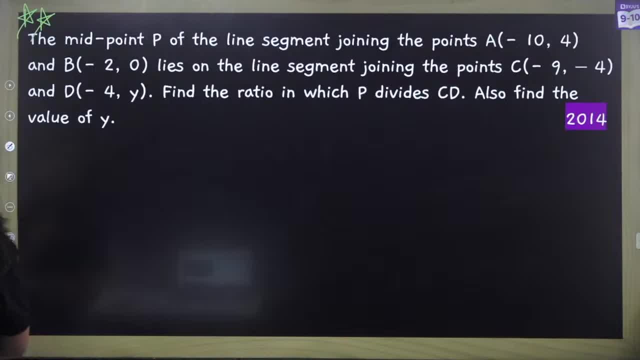 chalo. so let's solve this question. the mid point of point, the mid point P. P is the mid point. it is given to us. P is the mid point of the line segment joining A and B. so I am drawing a line. 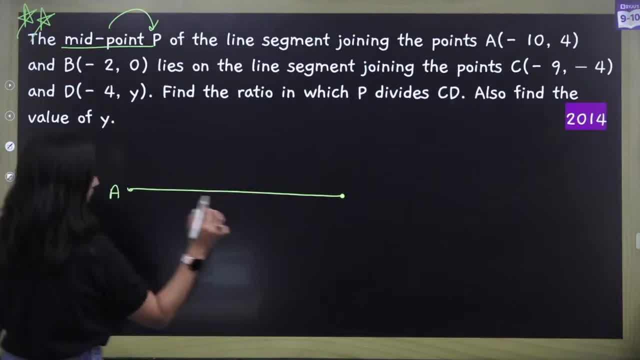 segment. this is my line. segment A, B to P is ka mid point hai. P is the mid point of A, B. achcha A ke coordinates, kitne de rakhi hai minus 10 comma 4, so A ke coordinates hai amare paas. 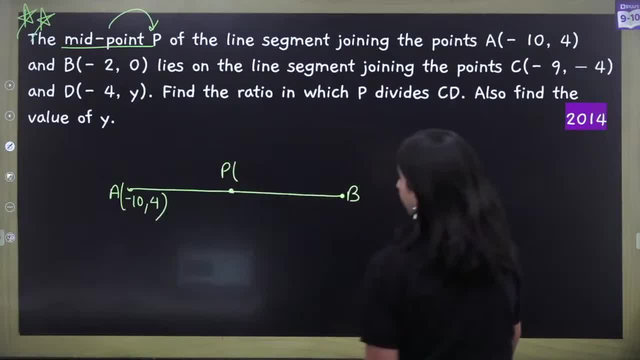 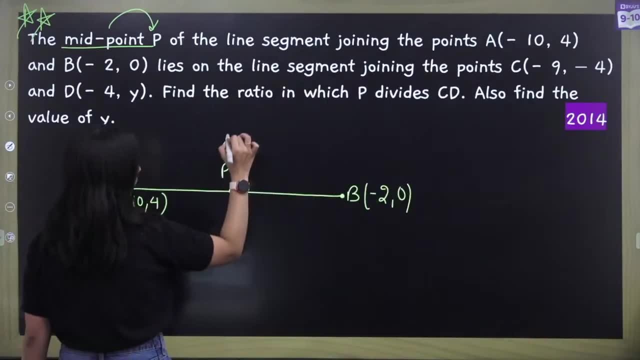 minus 10 comma 4 B ke coordinates hai. we have coordinates of B as minus 2 comma 0,. since P is the mid point, P, kya hai question mein given hai? P is the mid point of A, B right. 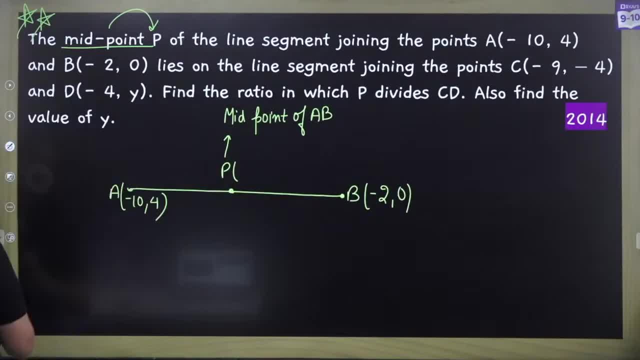 so if P is the mid point of A, B, I can clearly, I can easily find the coordinates: vo a jayenge minus 10 minus 2, that is, minus 12 upon 2, hai na to minus 12 upon 2. kya ho gaya, amare paas. 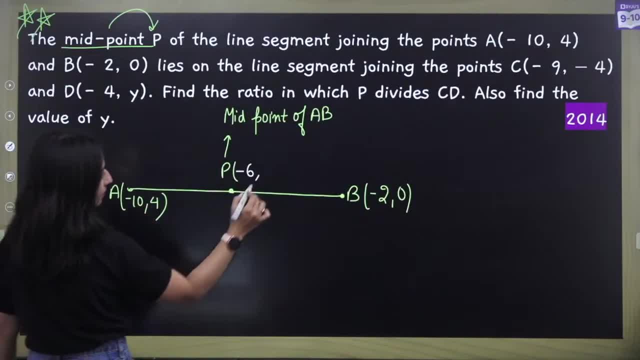 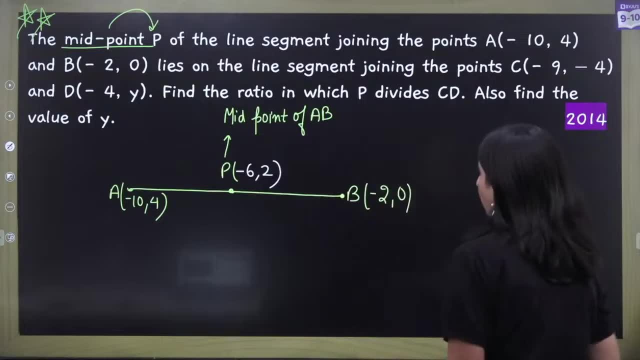 minus 6, comma 4 plus 0, divide by 2. 2 ho gaya to ye apke P ke coordinates ban gaya. yes, sab ke paas aage P ke coordinates. bahut badiya ab aage padho kya bol raha. 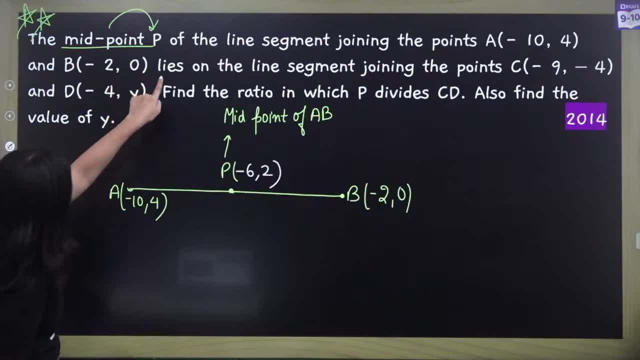 ho. this mid point P lies on the line segment joining the points C and D. kya ta ye jo P hai. ye ek aur line segment ke upar lie kar raha hai maine ek aur line segment bana di blue colour ki line segment bana di is. 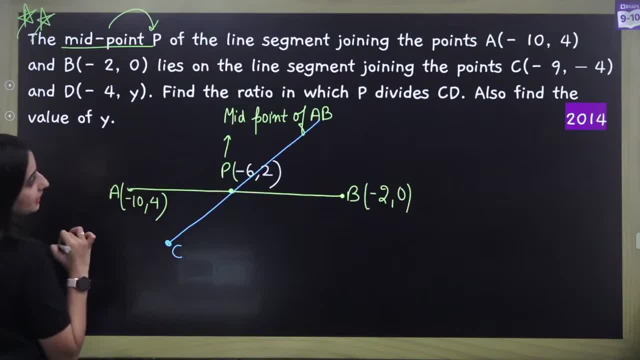 line segment ke jo points hai. ek point hai C, C ke coordinates de rakhi hai minus 9 comma minus 4, and the other coordinate is given as D minus 4 comma Y. this D is given as minus 4 comma Y, right so. 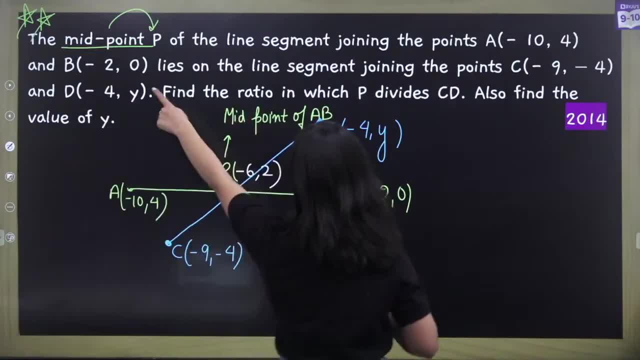 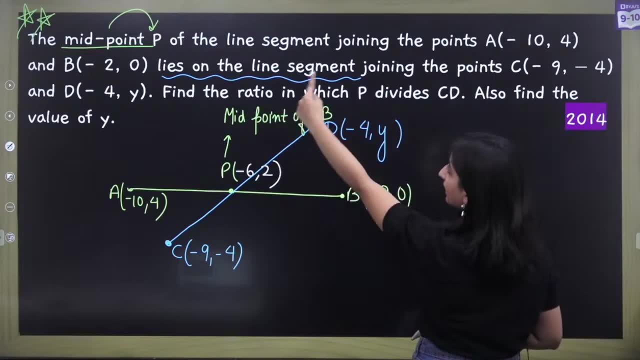 the question says. the question says that this point P it lies on the line segment ye P point hai wo lie kar raha hai kis line segment pe jo ki in 2 points ko join kar ke ban raha hai to blue wali line segment. 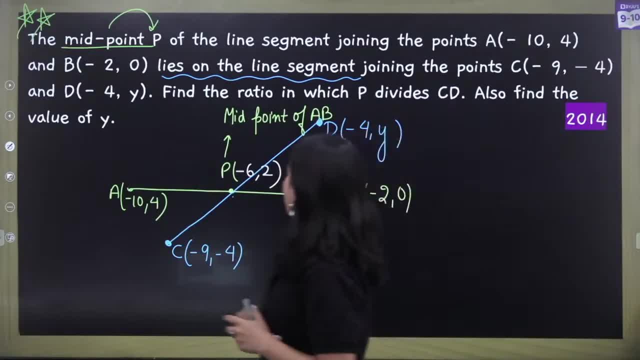 ki upar P lie kar raha hai. to aapko diagram se dikh raha hai: find the ratio in which P divides C, D. ek cheez ka dhyan rakna, jahaan pe aap galti kar sakte. 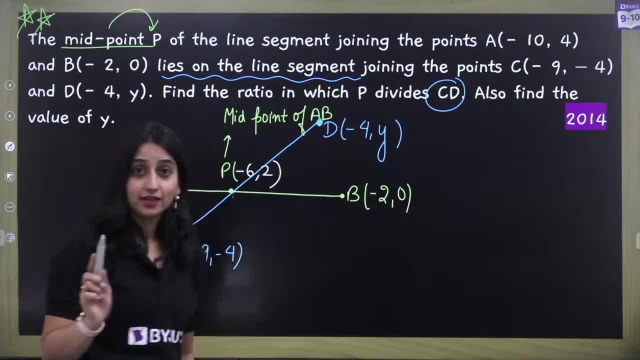 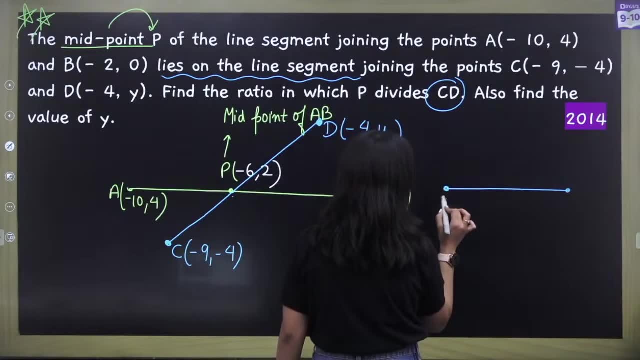 usne C D bola hai. usne C D bola hai, jab aap ratio loge, agar kisi bache ne line segment aise bana diya. suppose ye C hai aur ye D hai to maal lo ki ye P point. 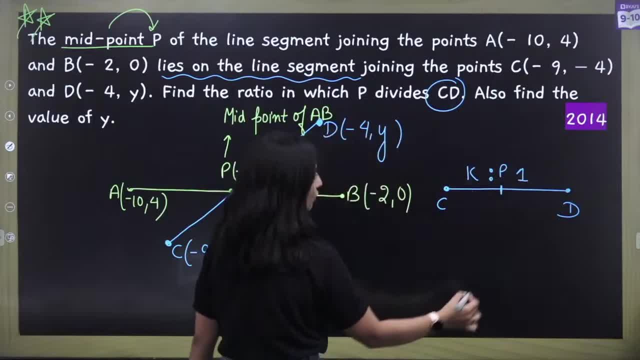 ko aapne aise divide kar diya, ma'am, ye K is to 1, ho jayega to bilkul theek hai, agar aapne aise line segment bana diya, yahaan pe aapne. 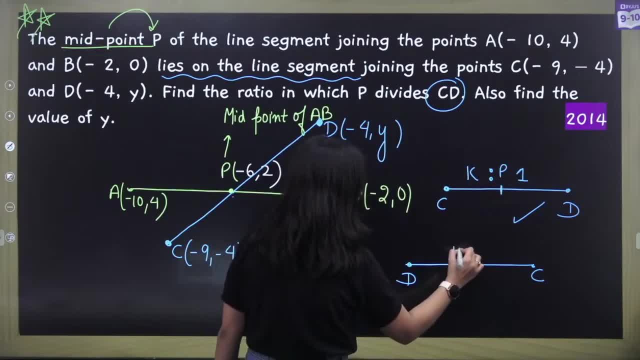 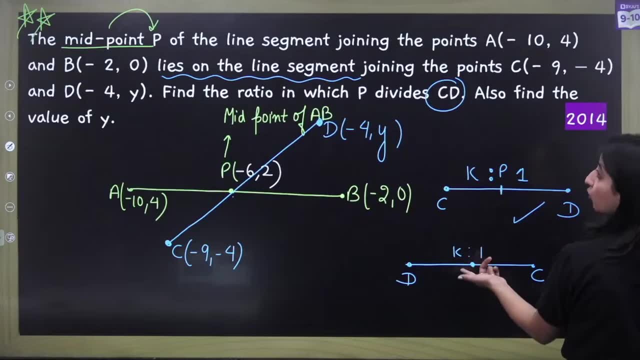 D bola aur yahaan pe aapne C likha aur fir aapne ye K is to 1 bol diya. theek hai, yahaan pe dhyan rakna ki aapki ratio, ratio reciprocal ho jayengi kyu. 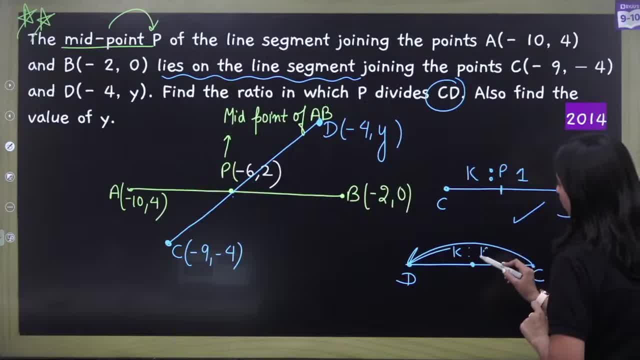 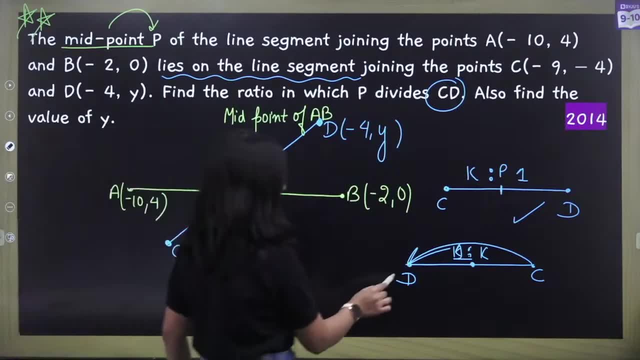 kyu ki aapne C, D ka ratio nikalna hai. so K is to 1 ka dhyan rakna ye silly mistake aap yahaan pe kar sakte ho? answer me, change aa jayega. are you getting my point ki maine? 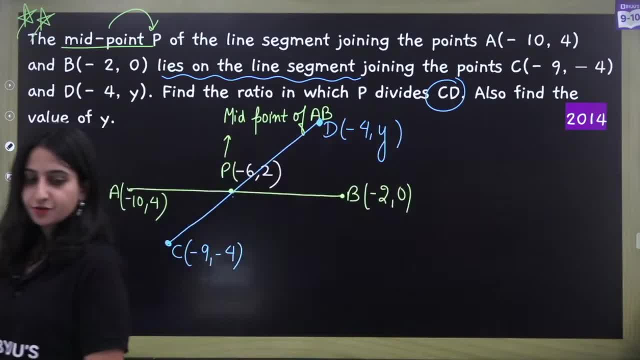 kya samjhaya abhi aapko yahaan pe? yes, sabko samajh me aaya to ratio reciprocal ho jayengi, chalo to yahaan pe is ratio ko kyu ki wo bol raha hai ki. 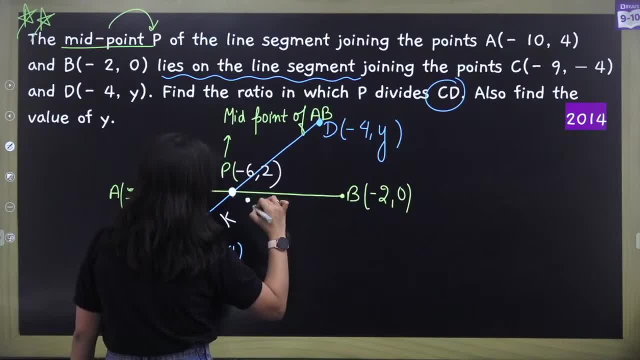 kis ratio me divide kare. to maine isko bol diya: K is to 1 ka ratio theek hai. to maine K is to 1 ka ratio le liya. bas, ab aapne kya karna hai? section formula lagana hai. 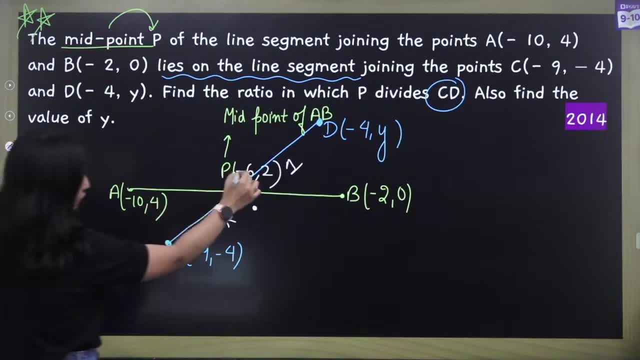 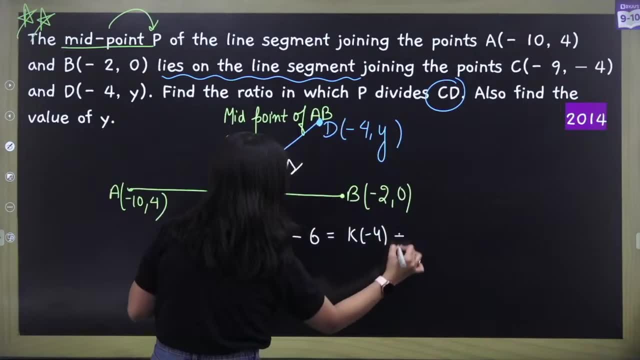 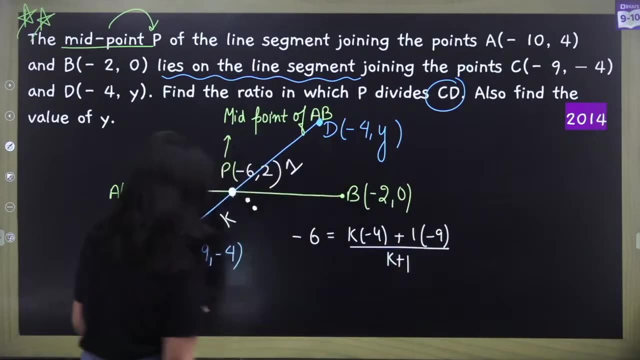 kum section formula laga dete hain bache to section formula me x coordinate, that is minus 6, kiske barabar hoga K into minus 4 plus 1 into minus 9. divide by K plus 1 to zara K ka value, batana kya aaya. 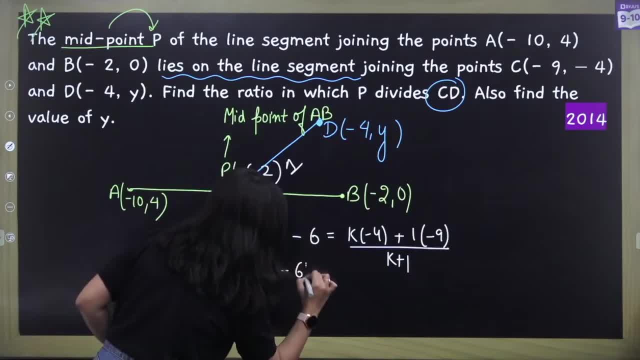 K ka value. kya aayega hamare pas yahaan pe aajayega. minus 6 K minus 6 equals to minus 4 K minus 9, to 4 idhar aaya. minus 6 K minus 9 equals to minus 4 K minus 9. 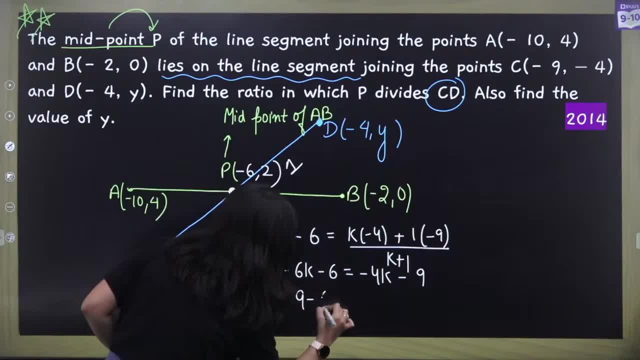 aayega ya fir 6 udhar chala jayega 9 idhar aaya ye ban gaya 9 minus 6 equals to 6 K minus 4 K. to ye ban gaya 3 equals to 2 K. 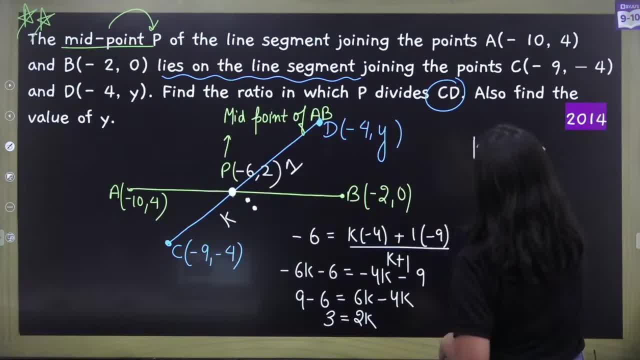 to K ka value aaya to K ka value aaya 3 upon 2, to ratio ban gaya hamare pas. 3 is to 2 to 3 is to 2 ka hamare pas ratio aaya. theek hai ab hame. 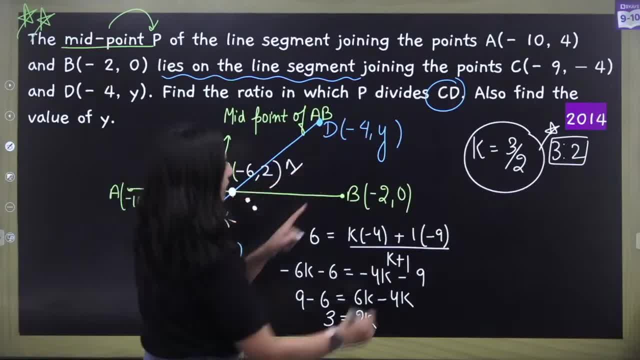 y coordinate bhi nikalna hai. na y ka value bhi nikalna hai. ye y bhi to nikalna hai. ye wala y chalo isko kese nikalna hai. ab hum y ke liye section formula laga dete hain. 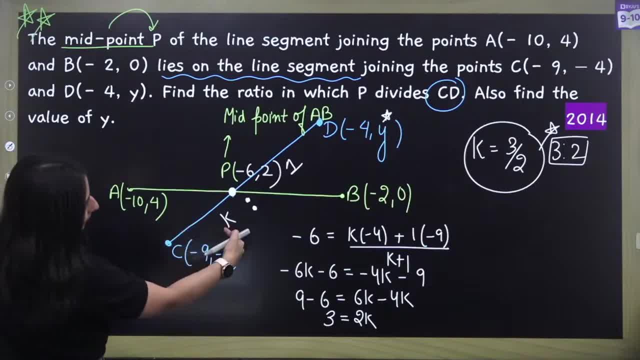 to uske liye ham kya karenge? ab hume K ka value pata? ye ban chuka hai. 3 is to 2 to chalo. abhi section formula laga dete hain: apka y kiske barabar ho jayega. 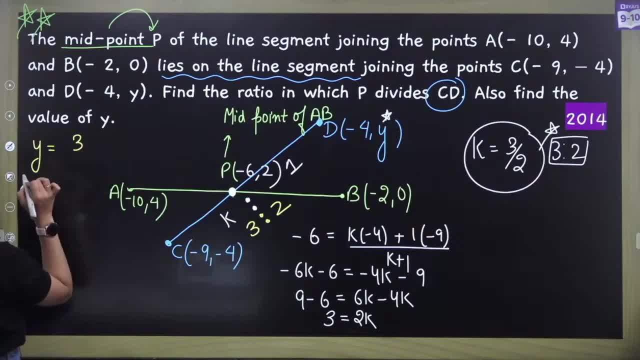 y will be equal to 3 into y. sorry my bad, not y is equal to ye 2 de rakha hai hamare pas. this is 2 is equal to 3 into y, 3 into y plus 2 into minus 2 minus 4. 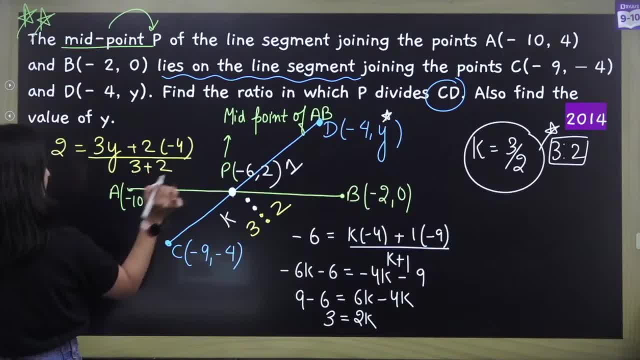 divide by sum 3 plus 2 to ye ban jayega 3, 4,, 5, 2 is a 10 equals to 3y minus 8 to ye ban jayega 3y equals to 10 plus 8. 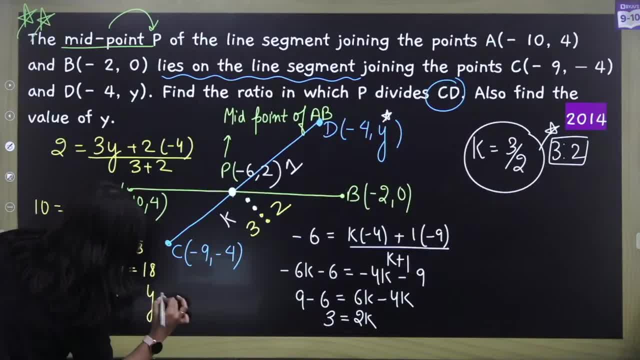 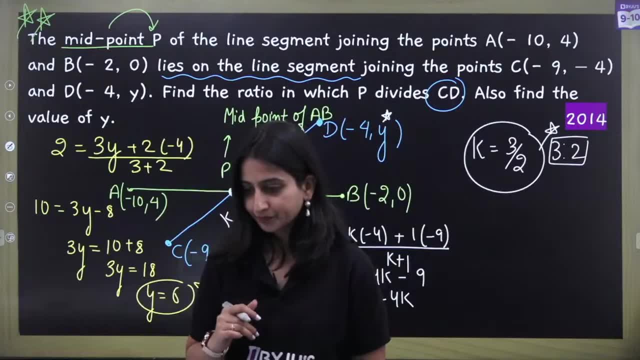 3y equals to 18, so y ka value a jayega apke paas 6 to beta. ye 3 to 4 marks ka question hai: no, beta, aap apni marzi se 1 is to 1 ka ratio nahi le sakte. 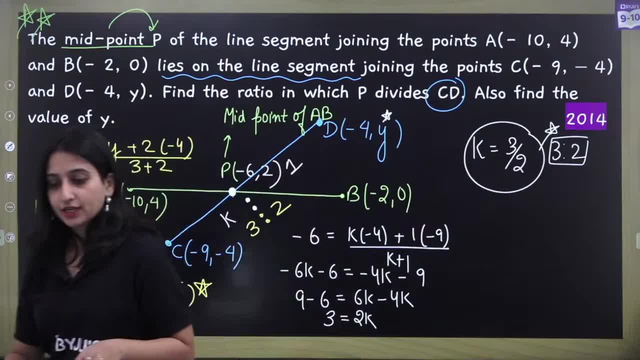 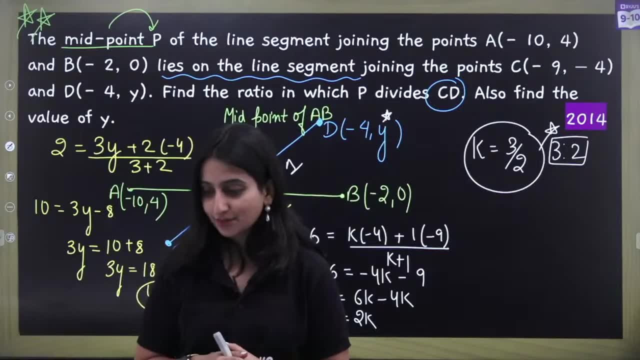 kyunki usne nahi de rakha hai ki this is the midpoint. agar midpoint de rakha ho, fir you can take 1 is to 1. otherwise you cannot take the ratio 1 is to 1. ok, don't assume that it is the midpoint. 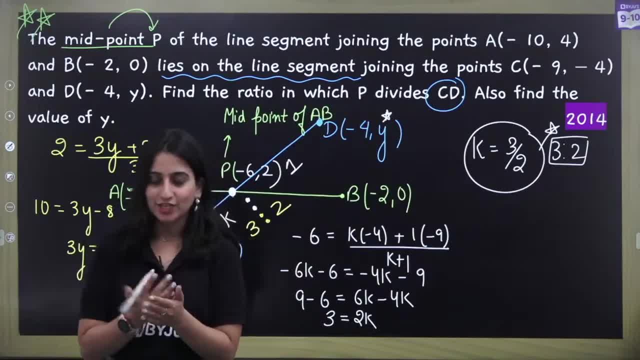 so jin bhi bacho ne ye mere solve karne se pehle solve kar diya the question. very good to all of you and jinko ye samajh me aage, aap logon ke liye bhi shabashi. 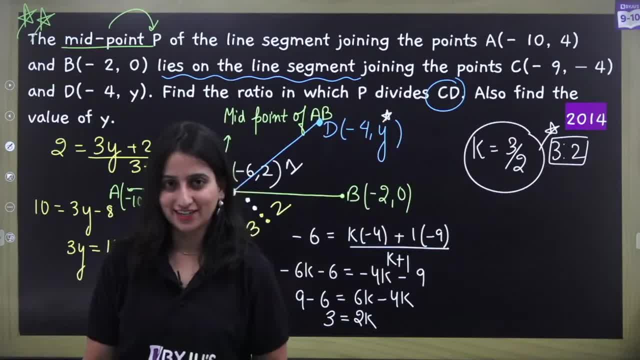 kyunki aap bethe ho aur aapne ye question samajhne, ki koshish kari hai. ok, so make sure, agar aapko koi bhi aisa question lag raha hai, ki ma'am samajh me nahi aaya. 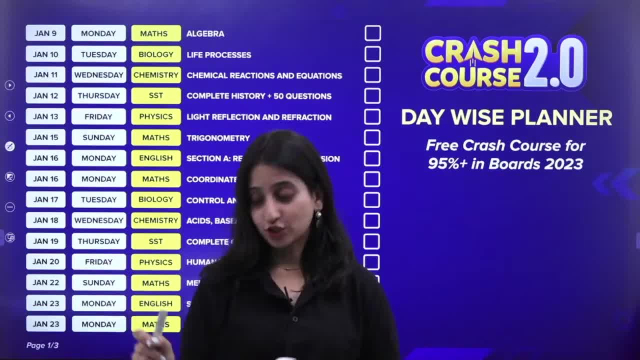 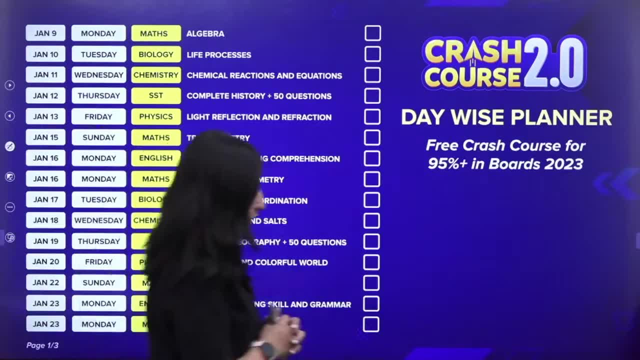 to ek bar. aap dubara se dekho aur usko dubara se practice karne ki koshish karo. aap surely samajh loge. ok, chalo, so aapko pata hai, ki crash course 2.0 is going on. 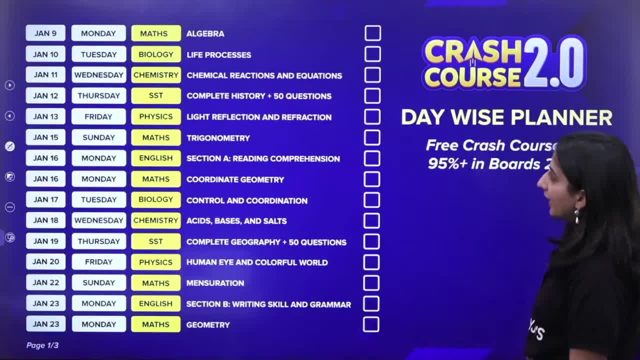 yes, ok to, ye aapka day wise planner hai. to jo, jo aap session dekhte ja rahe ho. honestly, achche se unke aage aap tip tick laga sakte ho. maine aapko algebra kara diya hai. 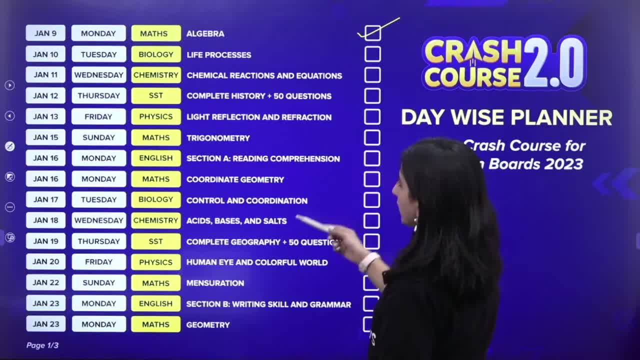 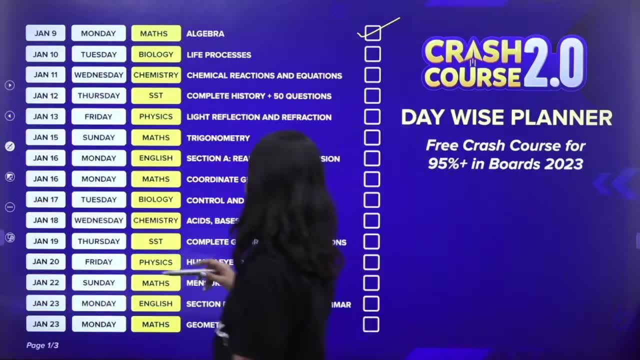 to ye saare sessions aapke ho chukke hai right. so next class, aapki maths ki trigonometry hai ok. uske baad ye coordinate geometry hum karne wale hai right. so ye dekho maths ki chapters. you can see.